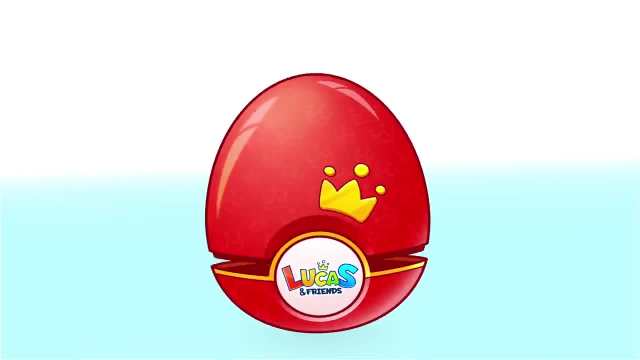 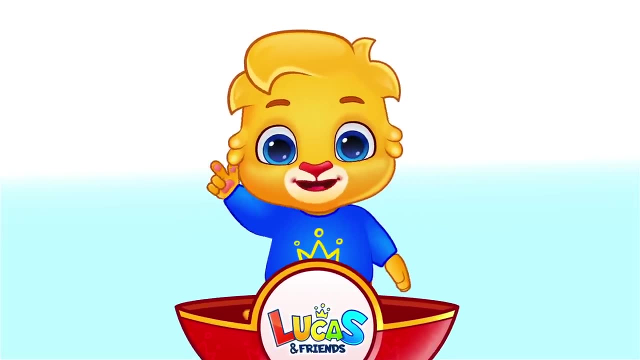 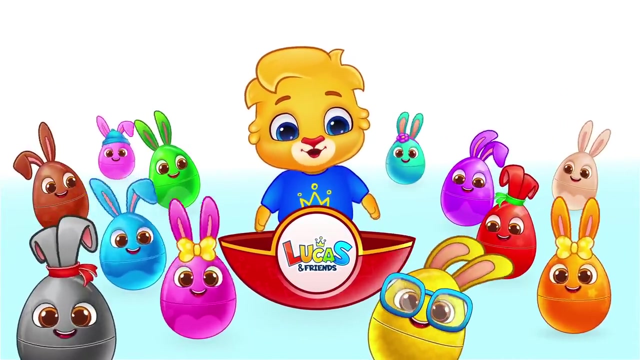 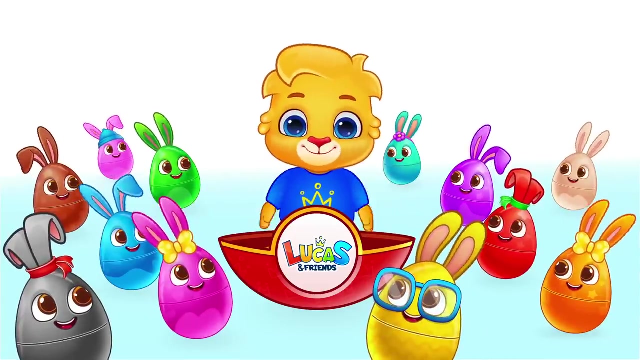 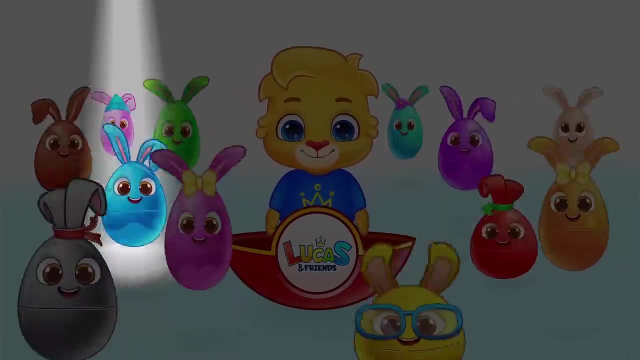 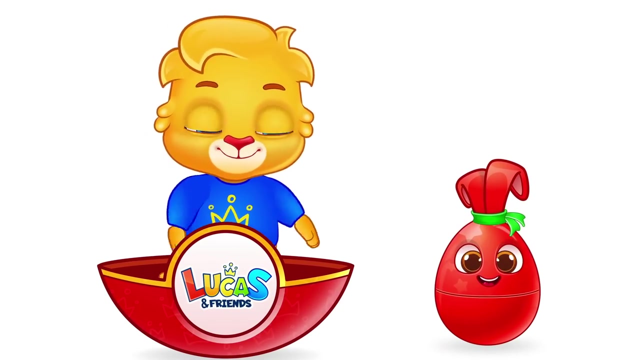 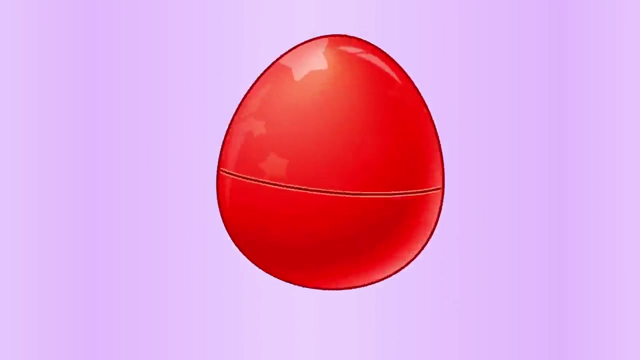 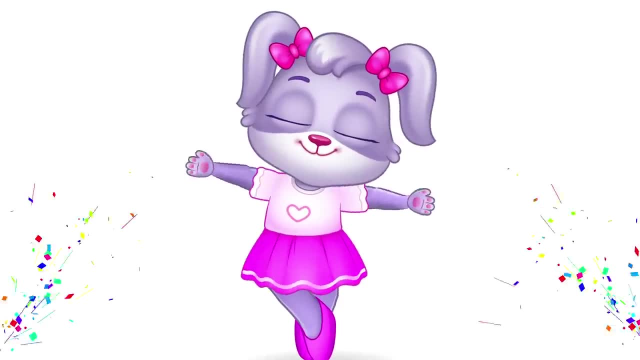 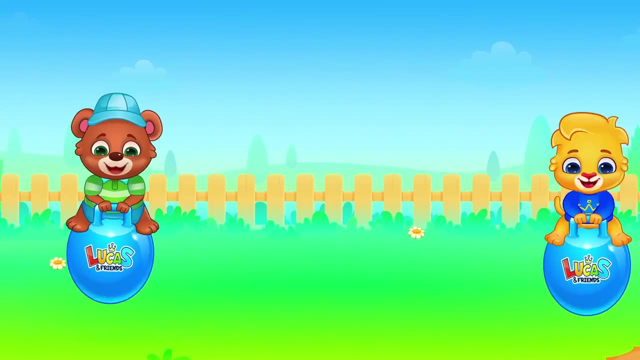 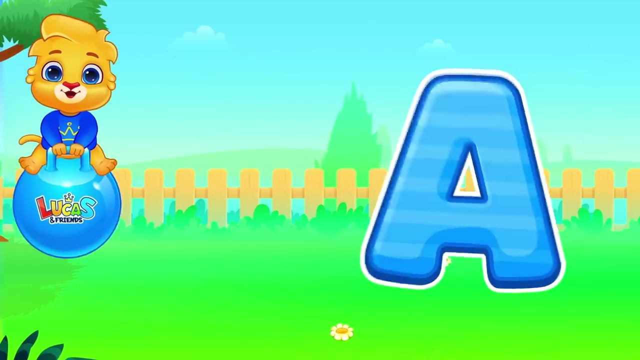 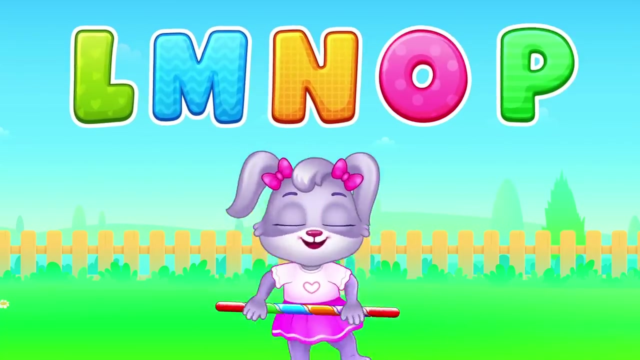 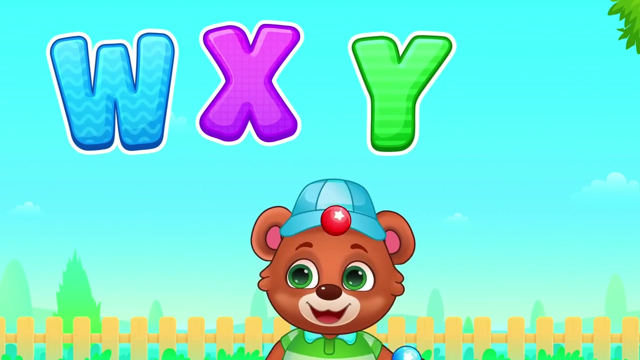 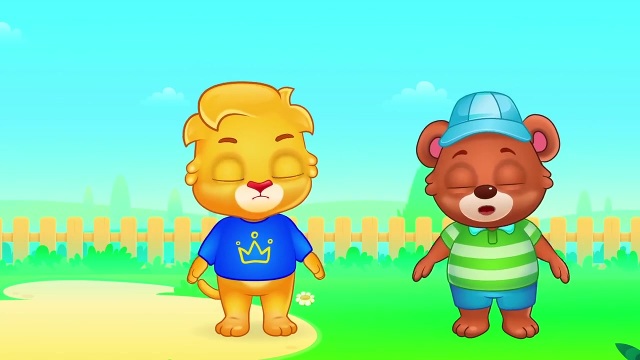 A, B, C, D, E, F, G, H, I, J, K, L, M, N, O, P, Q, R, S, T, U, V, W, X, Y and Z. now I know my A, B and Z. next time won't you swim with me? 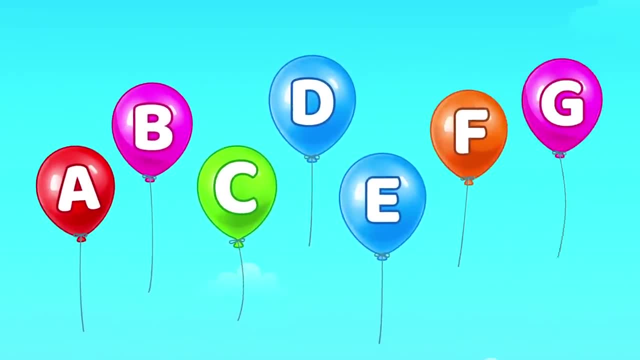 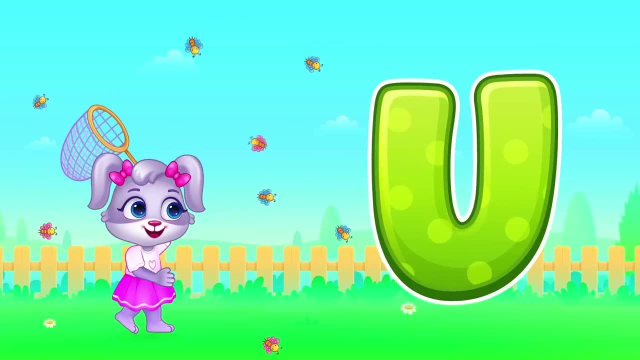 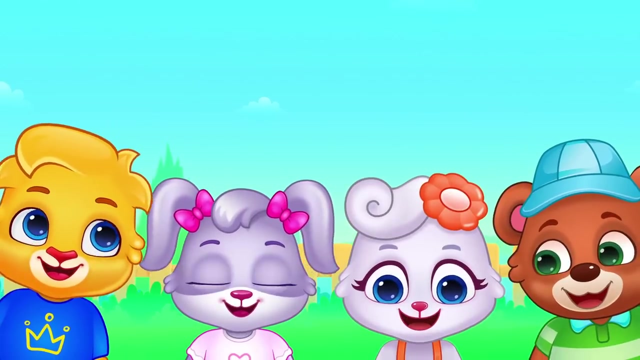 A, B, C, D, E, F, G, H, I, J, K, L, M, N, O, P, Q, R, S, T, U, V, W, X, Y and Z. now I know my A, B and Z. next time won't you swim with me? 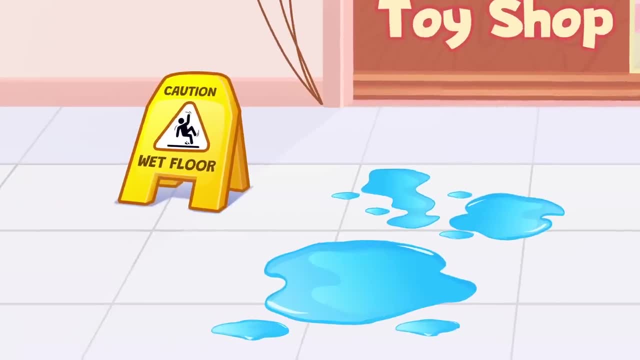 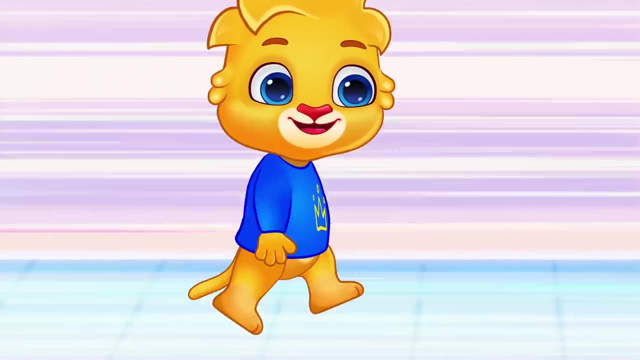 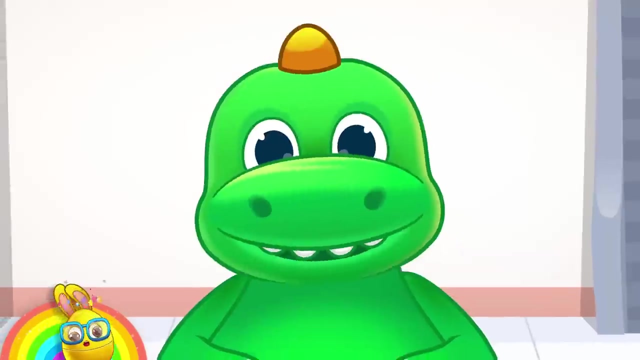 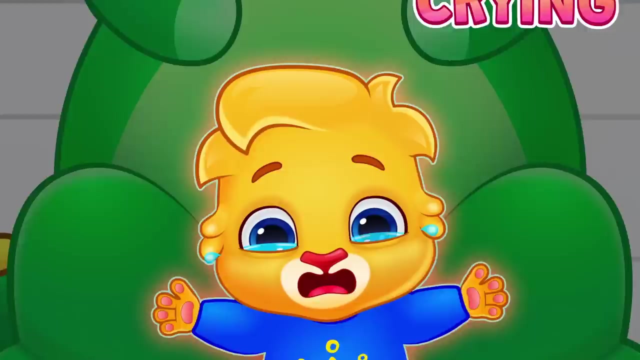 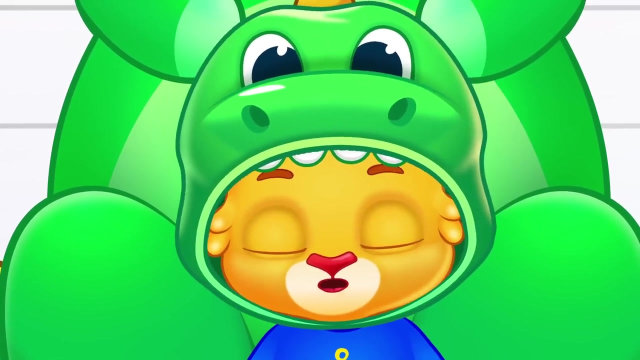 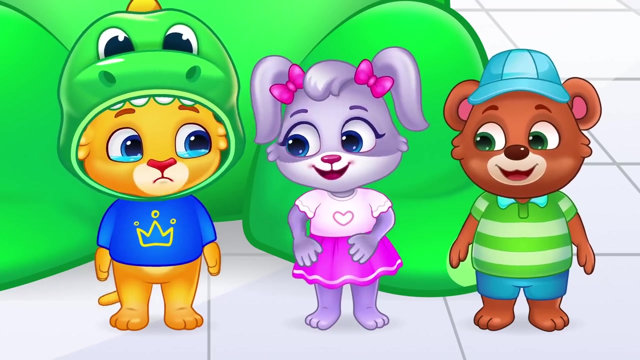 A, B, C, D, E, F, G, H, I, J, K, L M N, O, P, Q R S A, B, C, D, E, F, G, H, I, J, K, L M, N, O, P, X, Y and Z. now I know my A, B and Z. next time won't you swim with me? 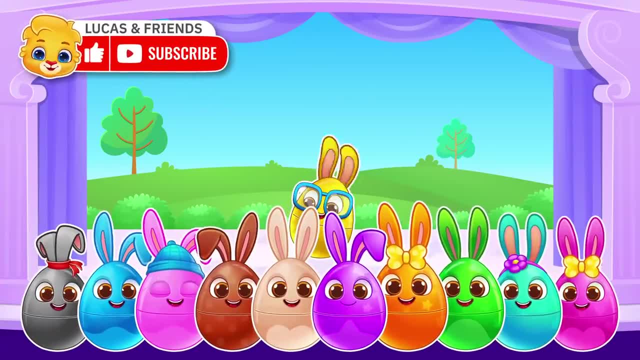 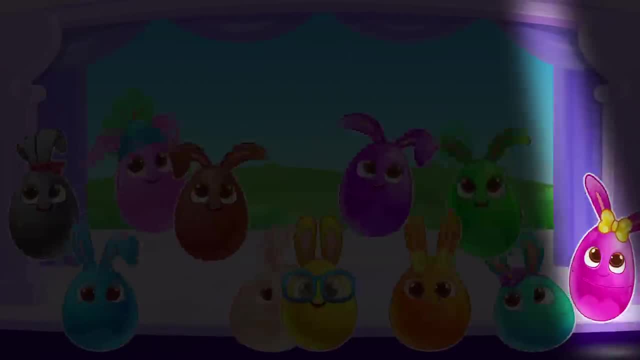 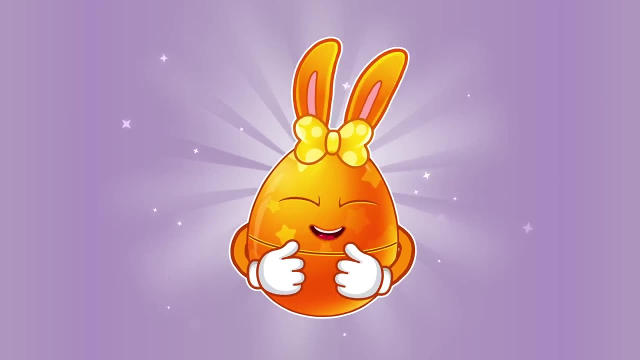 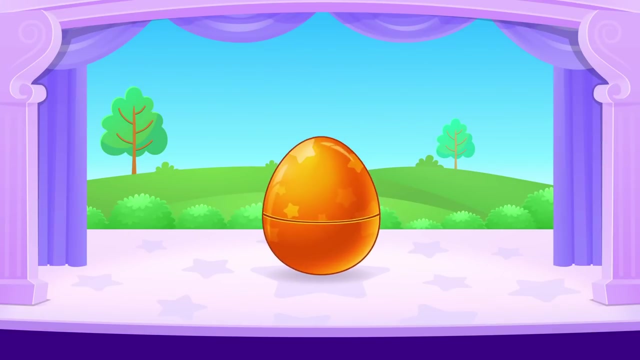 A B C D E F H I J K L M N O P Q? R. S. A B C D E F H I J K L M N O P Q R. S. 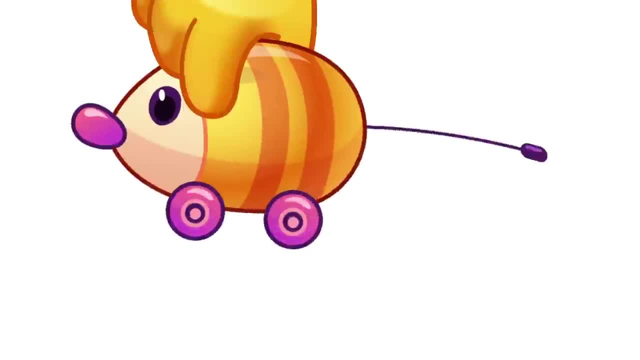 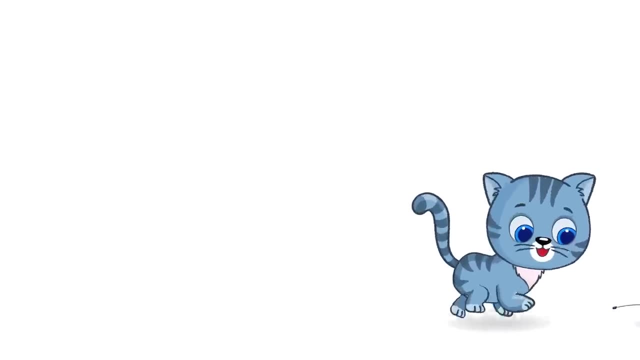 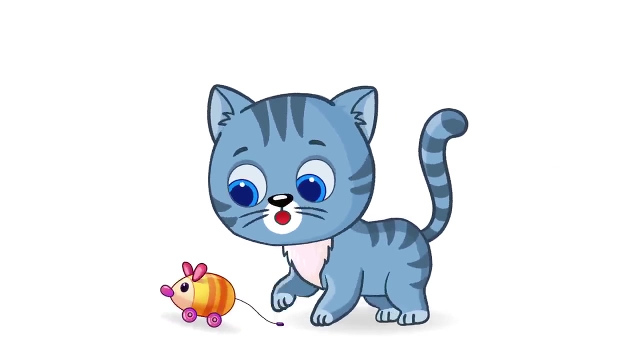 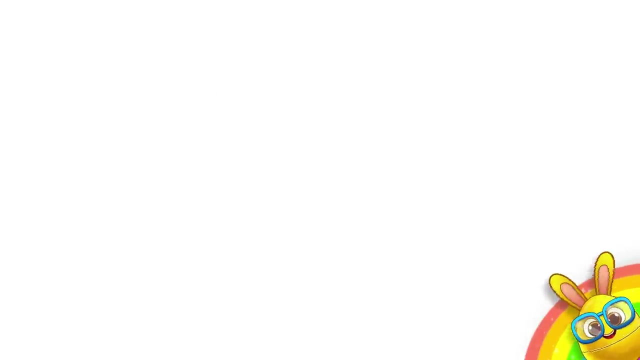 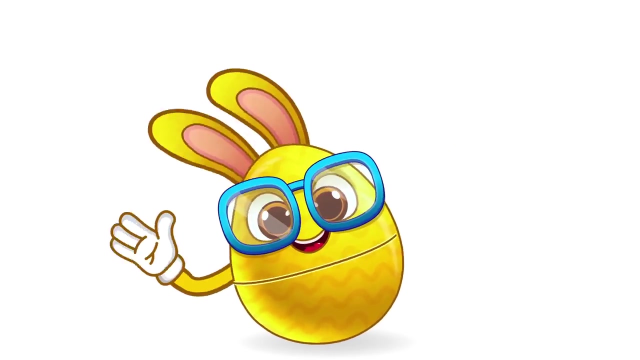 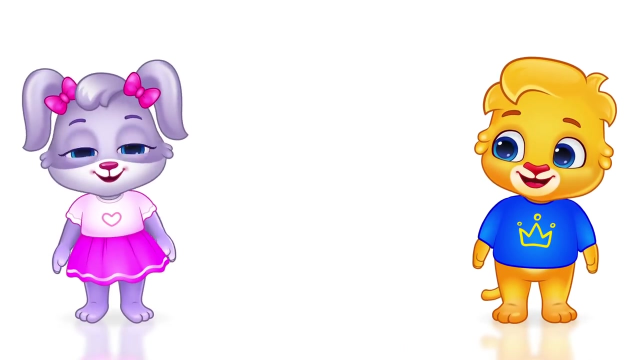 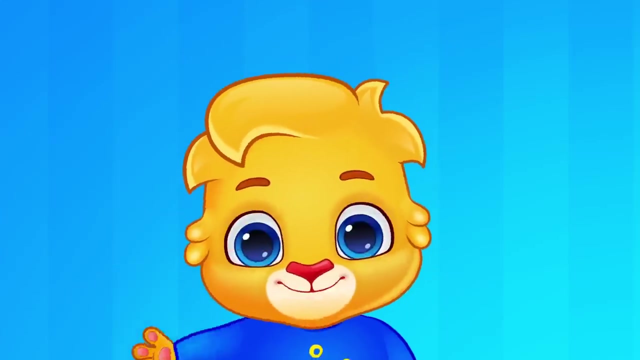 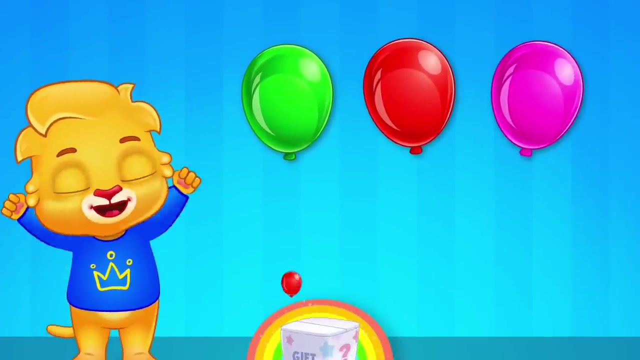 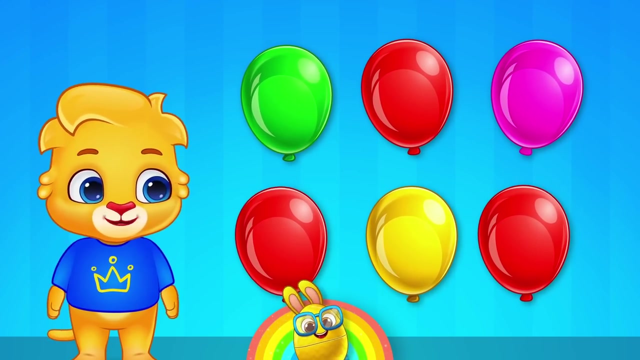 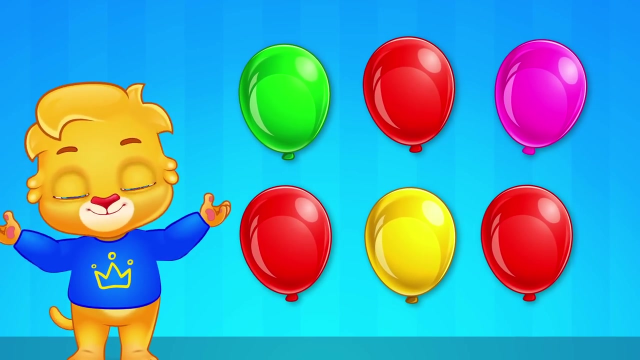 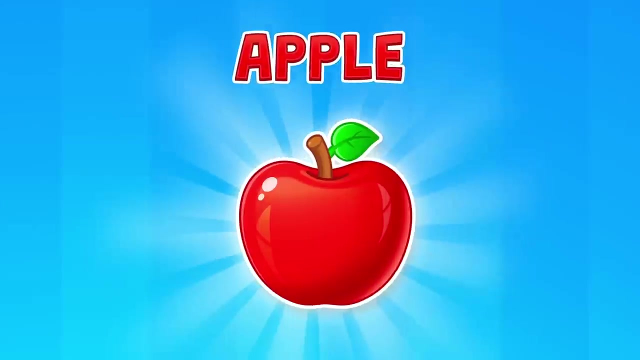 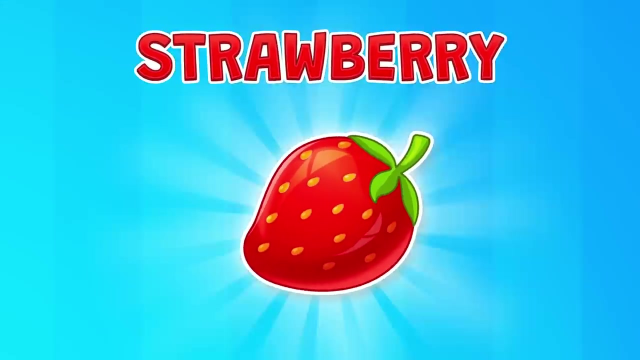 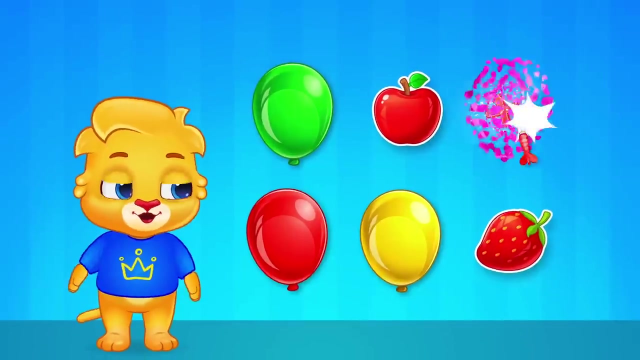 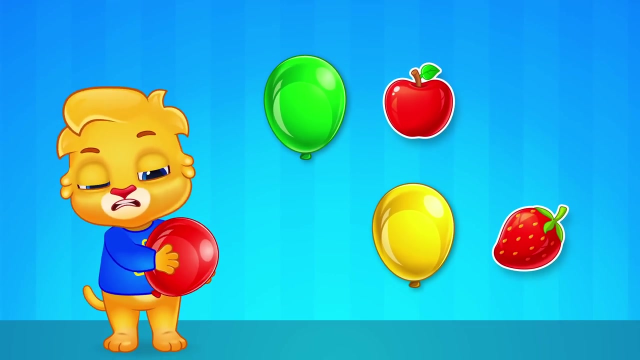 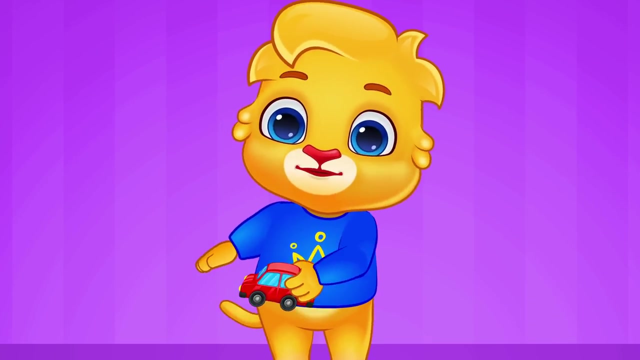 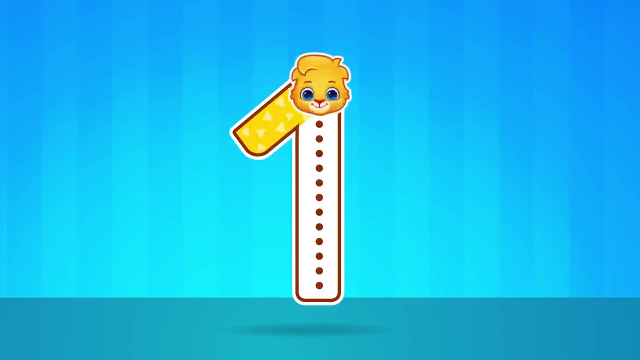 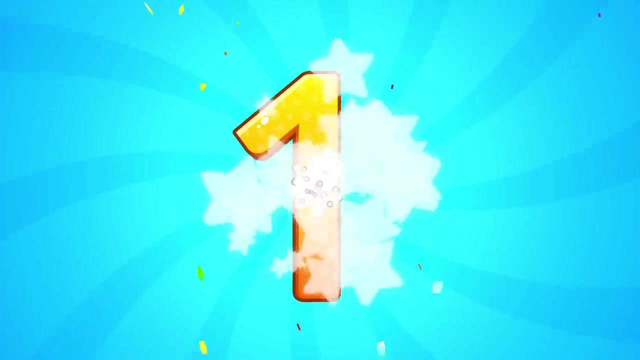 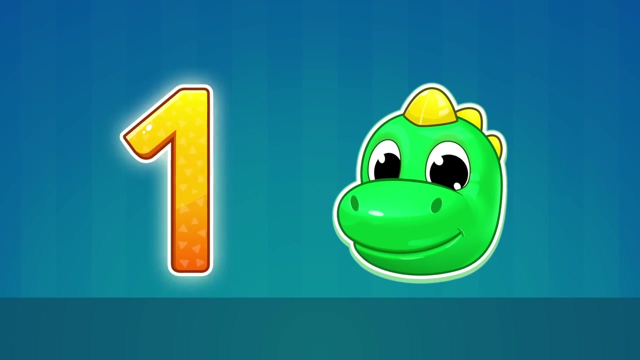 Oh, Oh, Hi, i'm lucas, hi, i'm ruby, and we're lucas and friends, Hi friends. Oh, Look, six balloons, Hey friends, red balloons. who's ready to pop them? Red apple is red, Right strawberry is red Is red. Yeah, Dinosaur, what dinosaur. 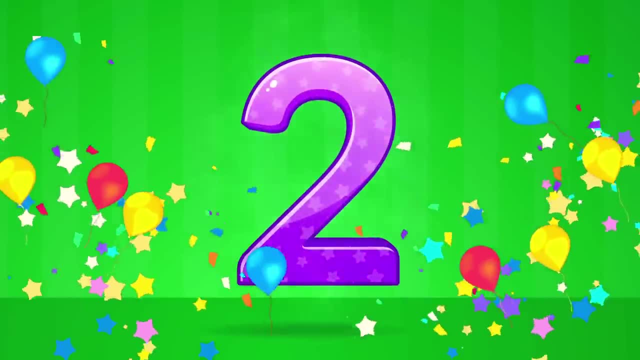 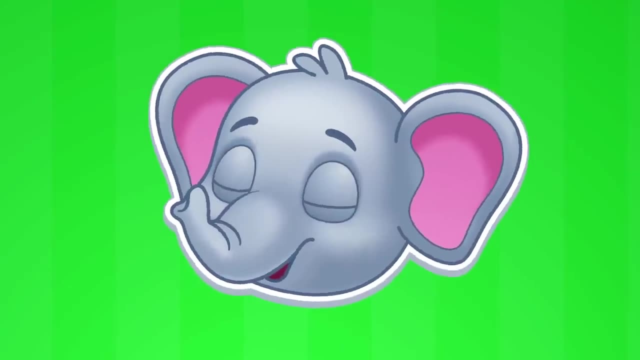 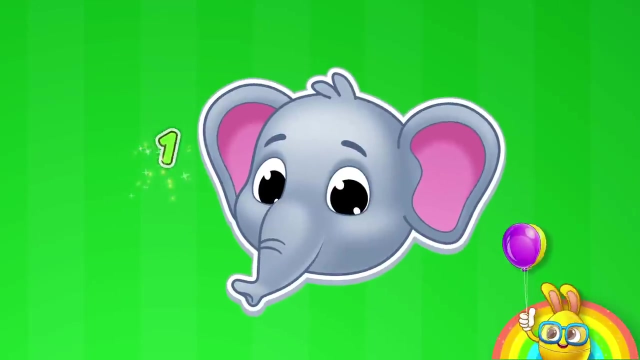 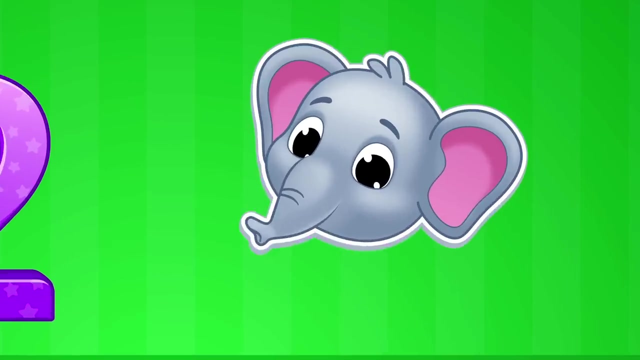 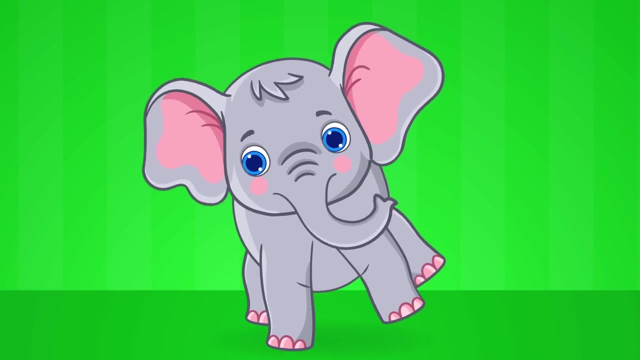 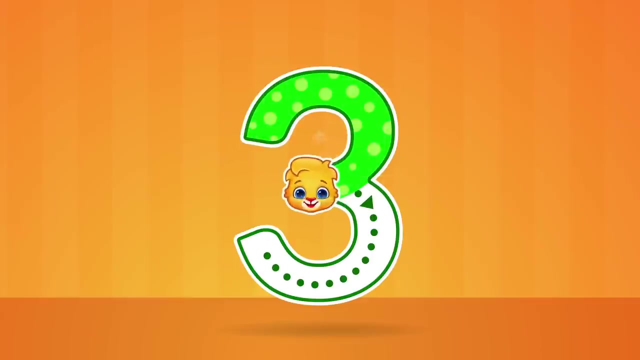 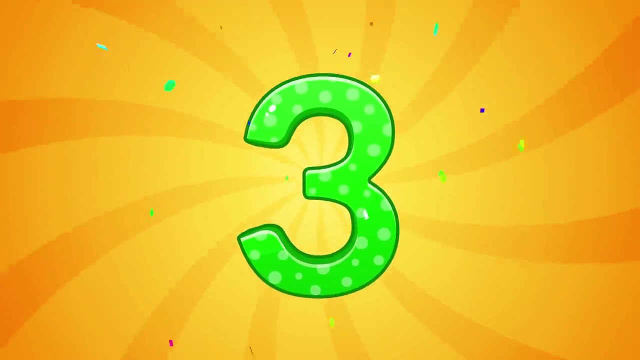 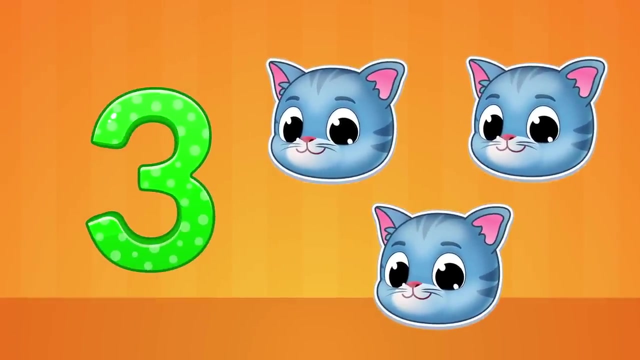 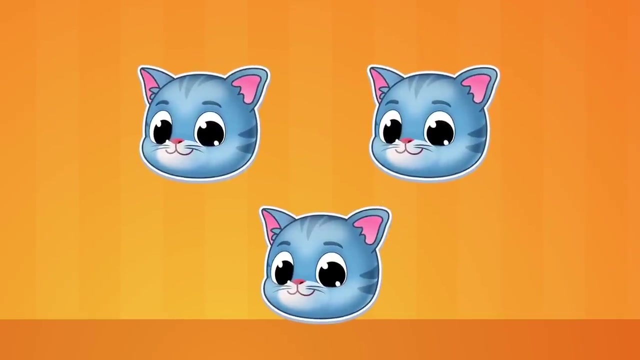 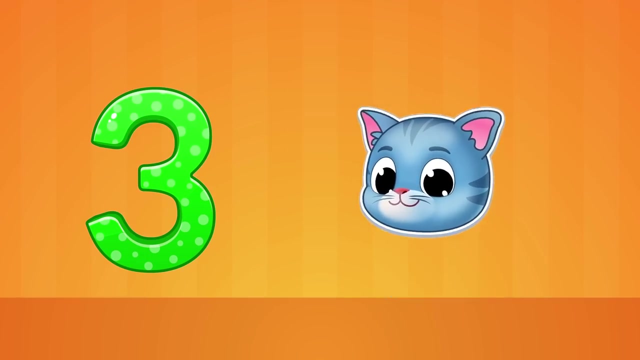 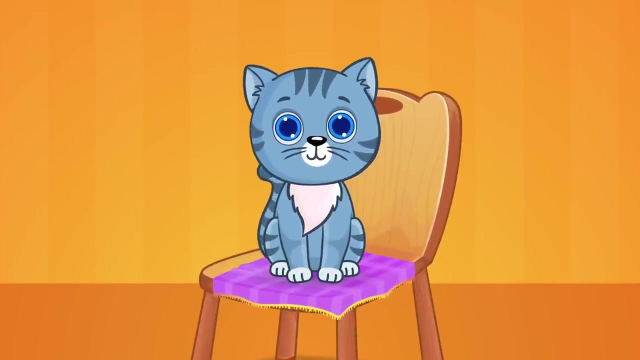 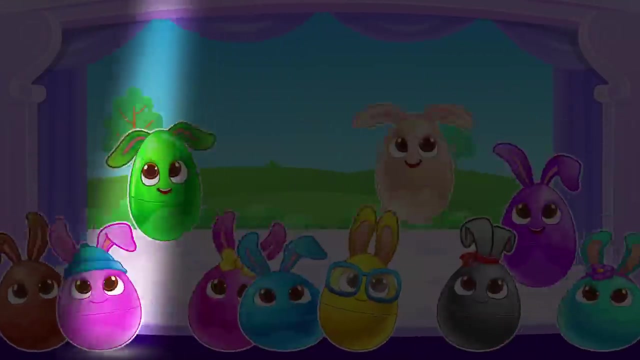 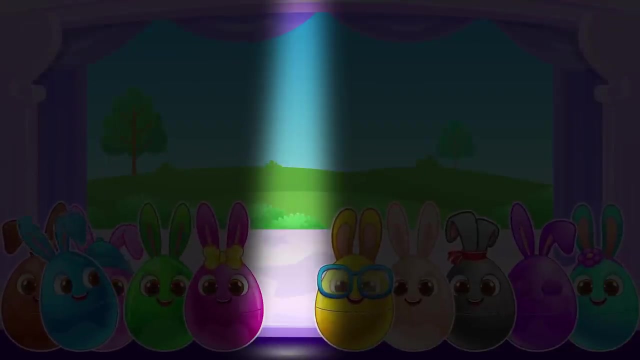 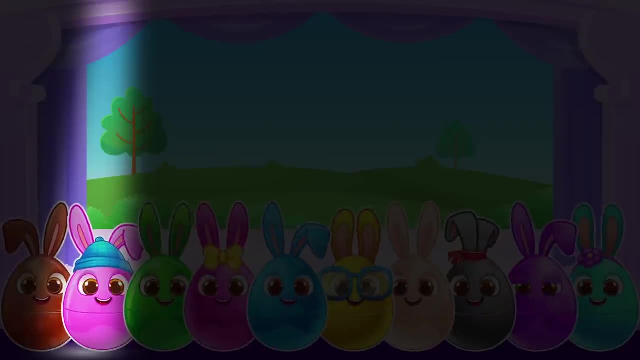 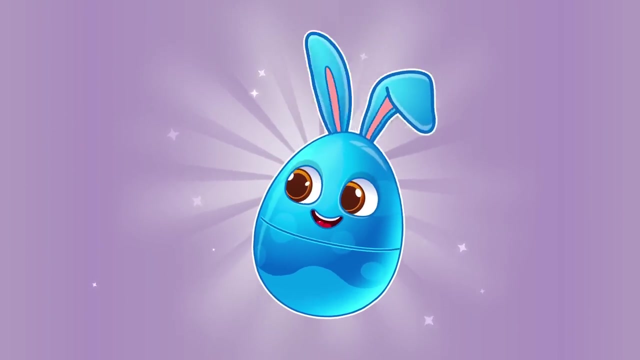 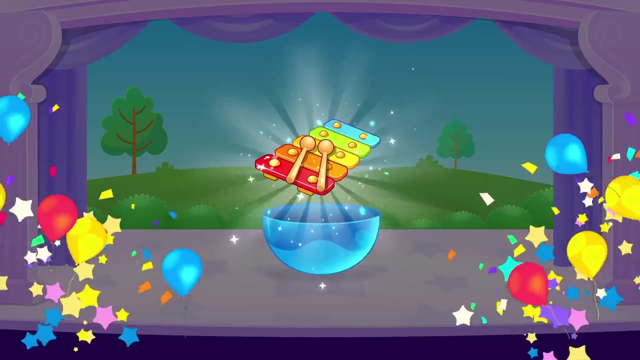 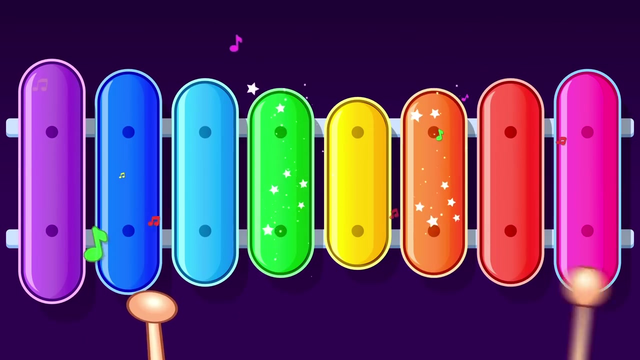 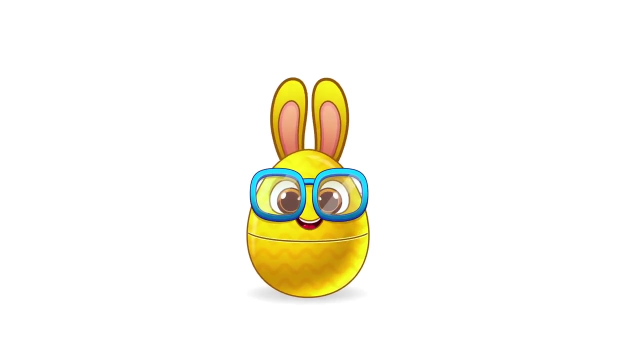 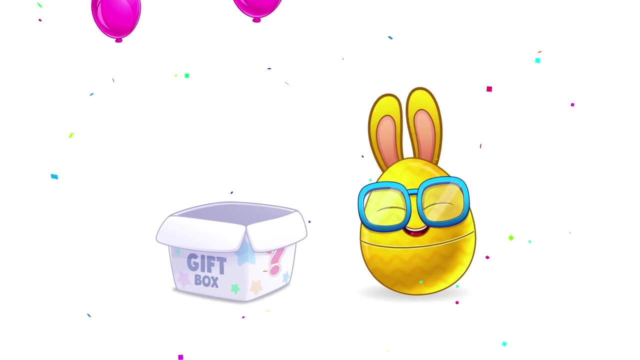 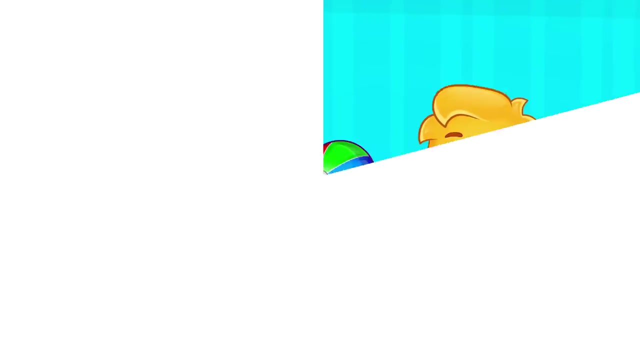 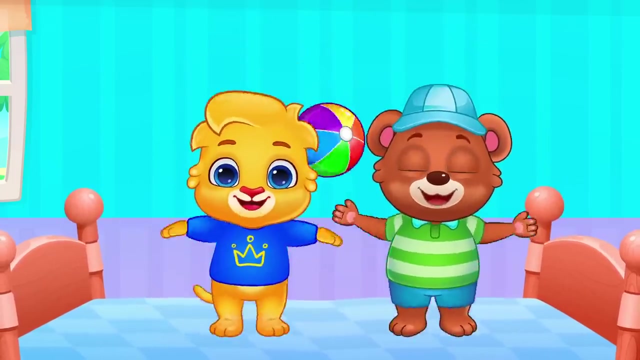 Spirulip: Uh, Huh, Huh, Huh, Wee, hee, hee, hee, Yippee, Wee, hee, hee, hee, Huh, Huh, Ha. I will be the next Five little monkeys jumping on the deck. 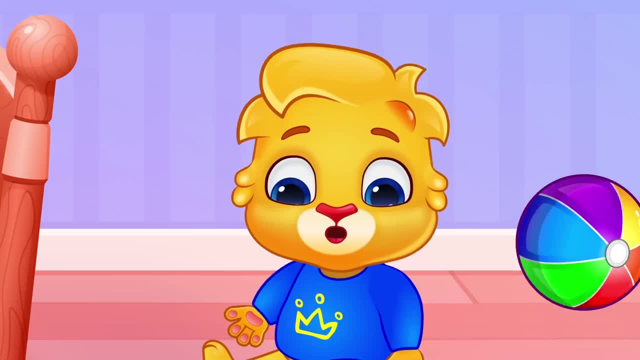 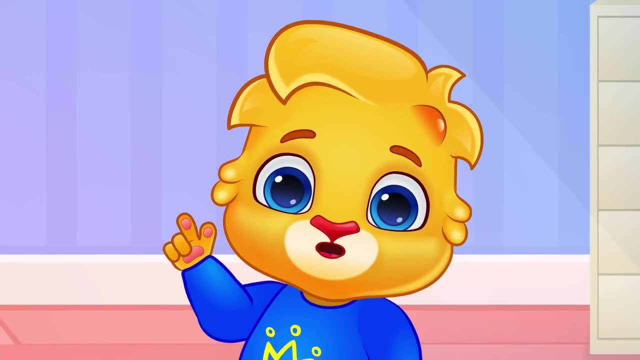 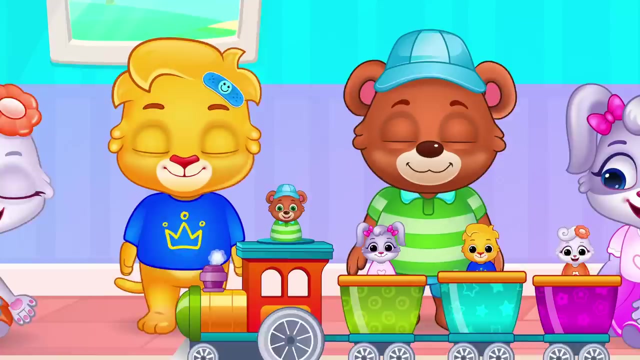 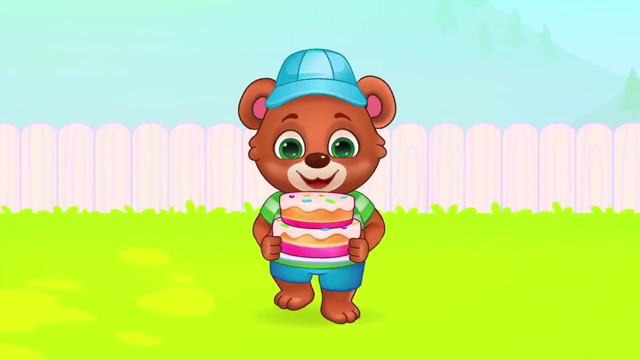 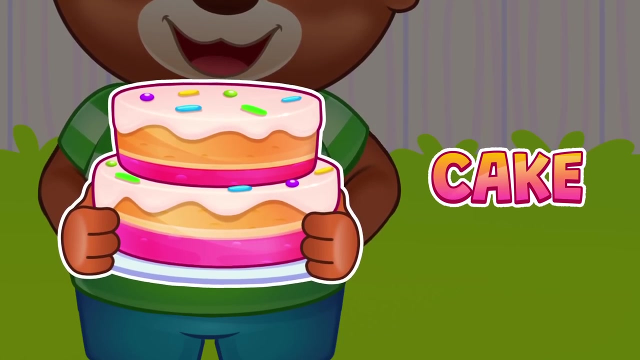 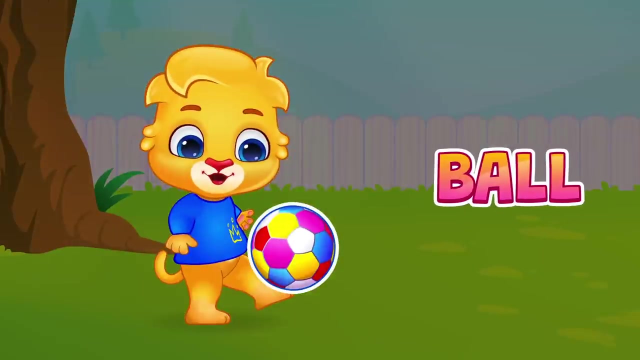 One fell off in the bed. Mama called the doctor and the doctor said: No more monkeys jumping on the bed. No more monkeys jumping on the bed. Yummy Cake. See Is for cake Ball. Lucas is playing with one ball. 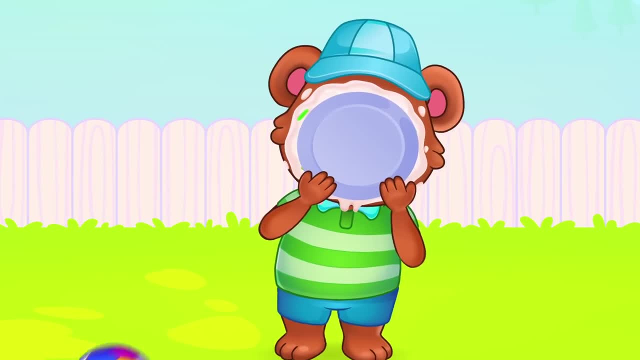 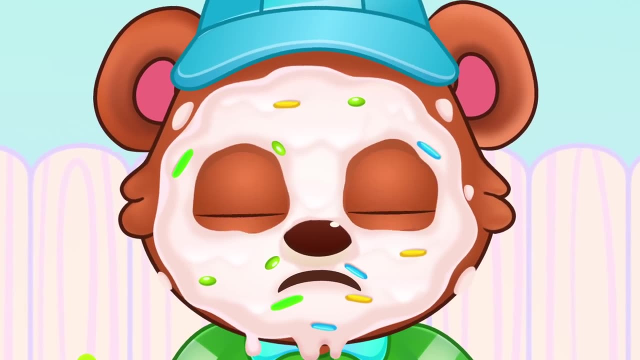 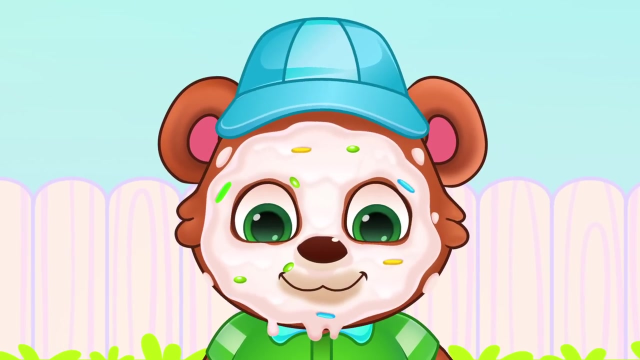 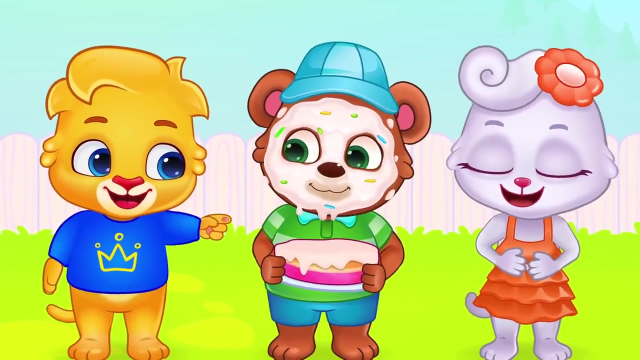 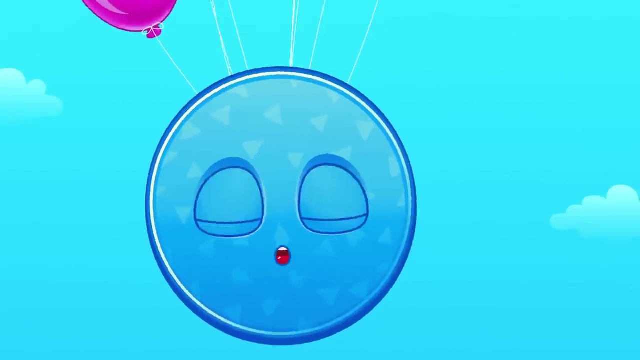 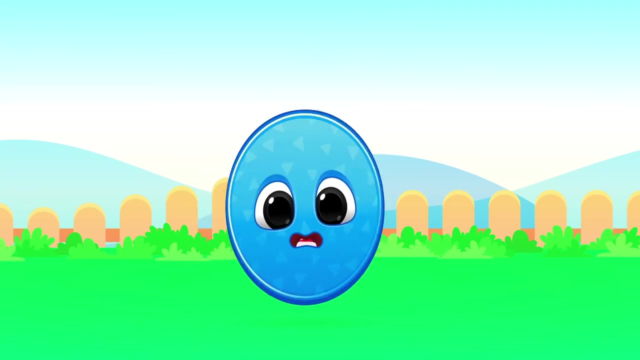 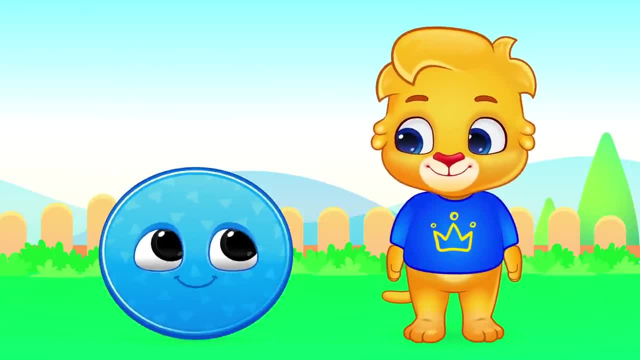 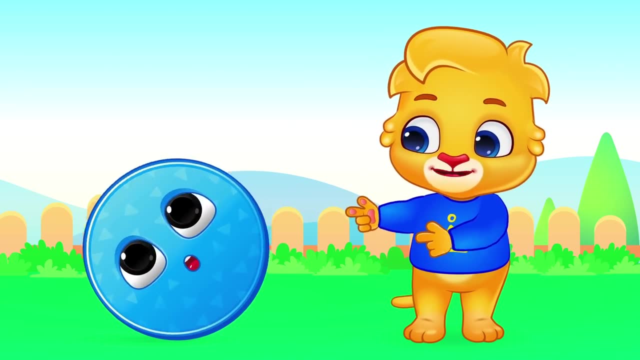 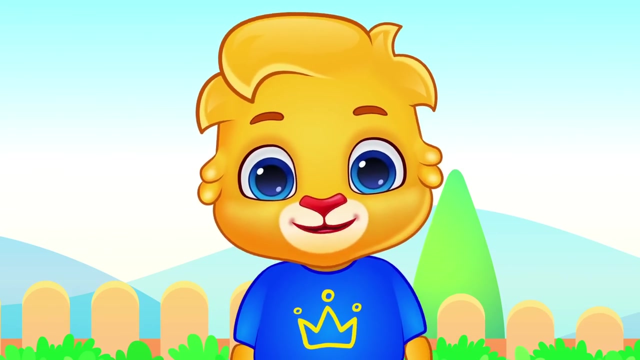 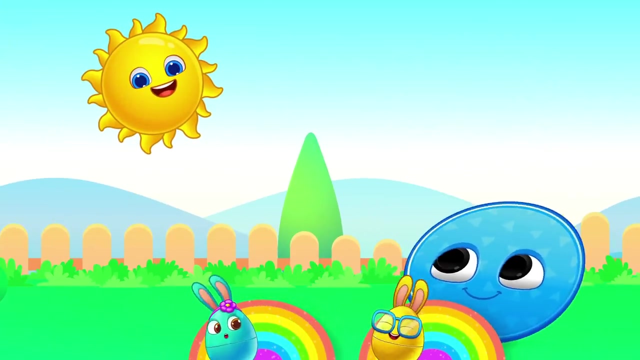 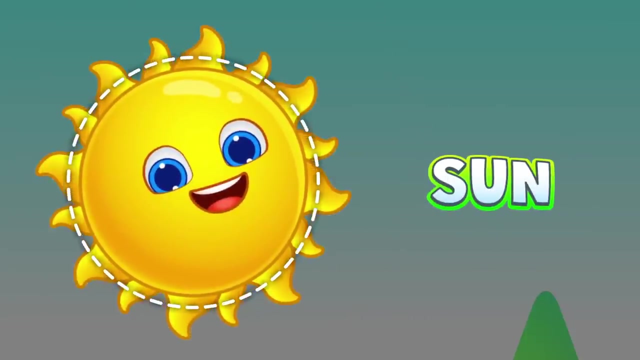 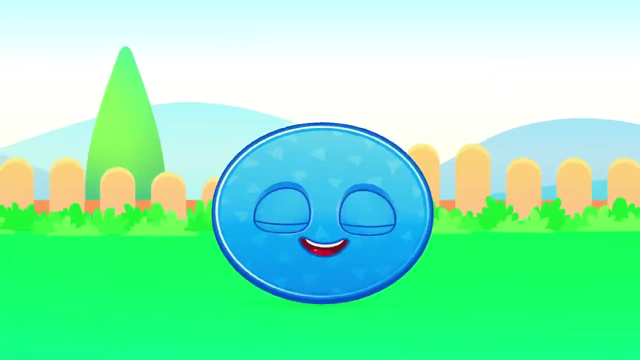 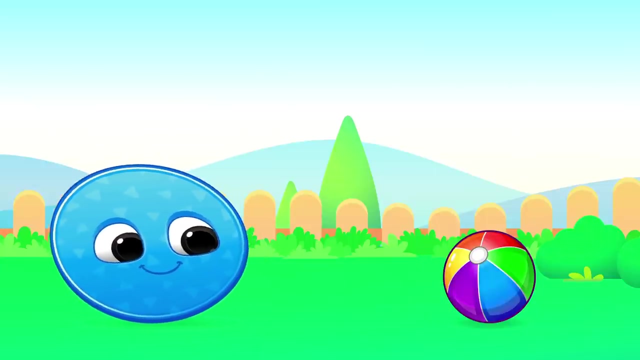 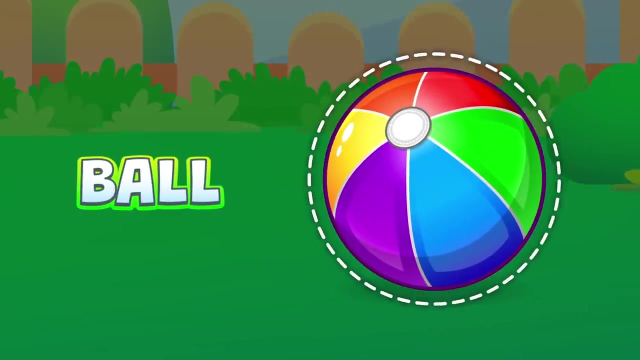 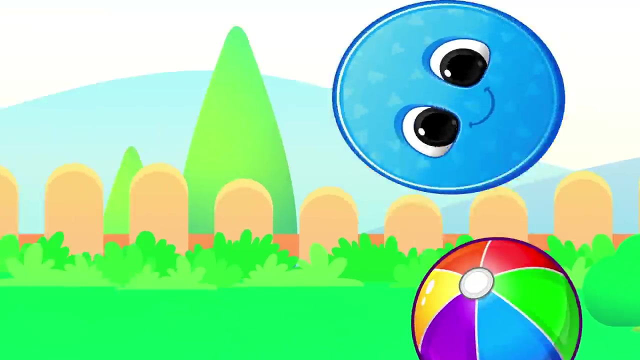 Hello, Hello. Do you know what shape is this Circle? Yes, Yes, you are right, my friend, The sun is circle, A ball is circle, A ball is circle, A ball is circle. Yay. 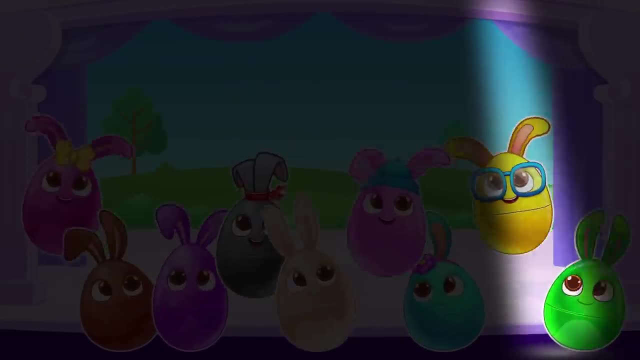 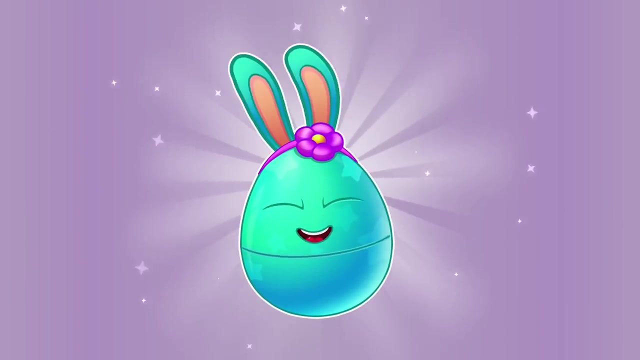 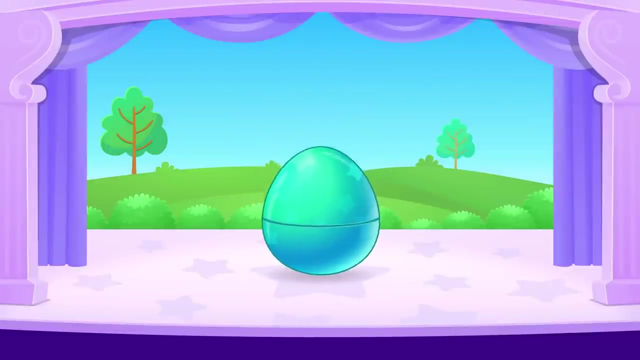 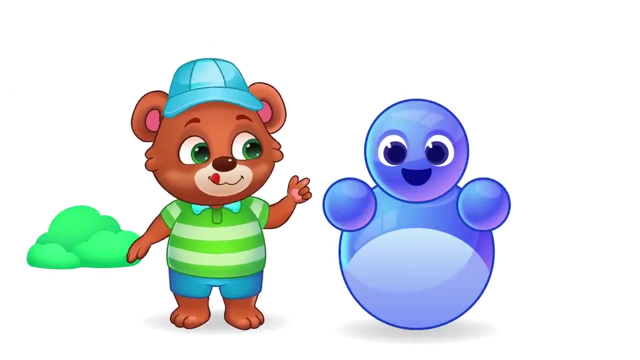 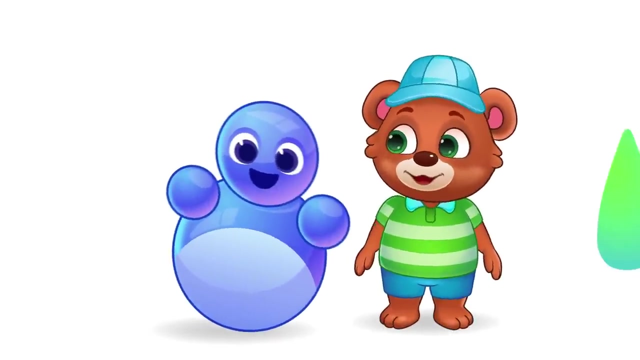 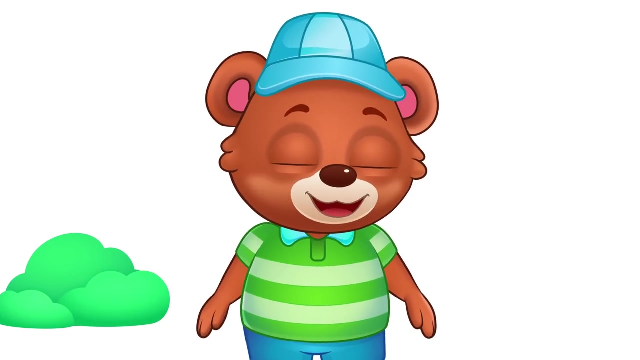 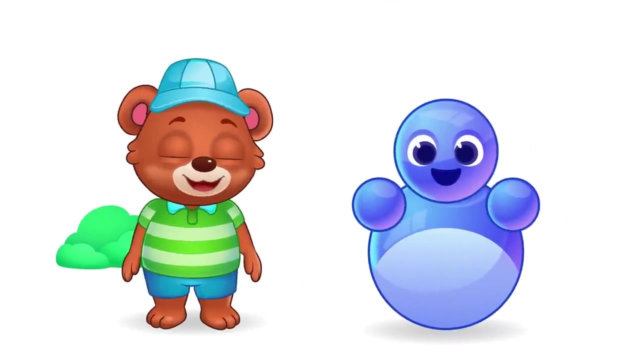 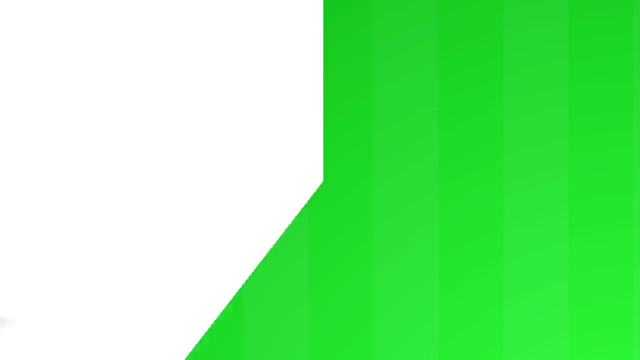 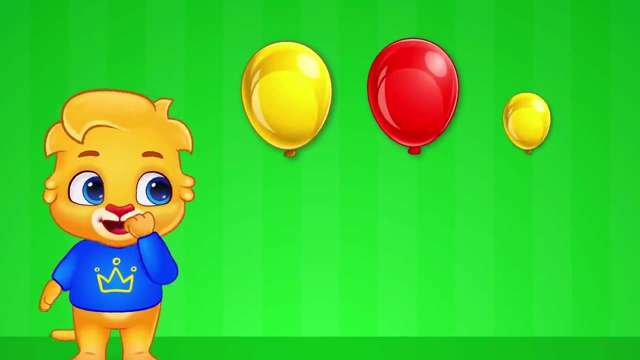 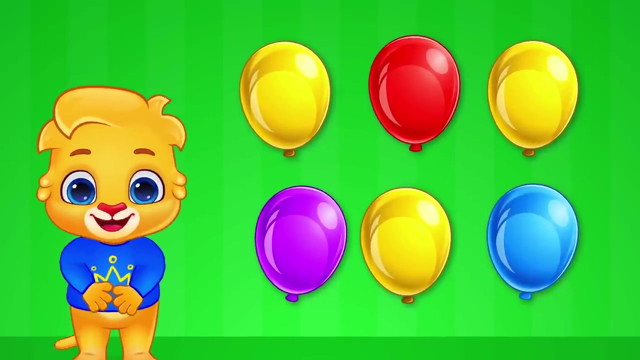 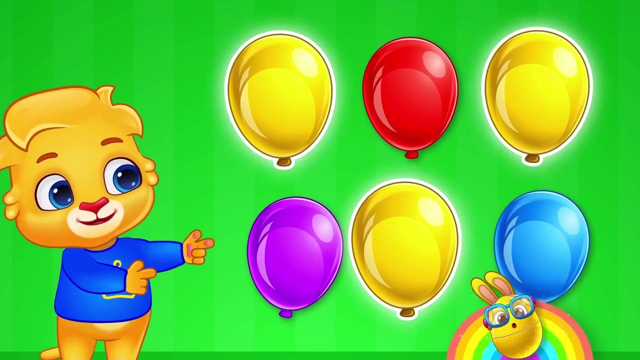 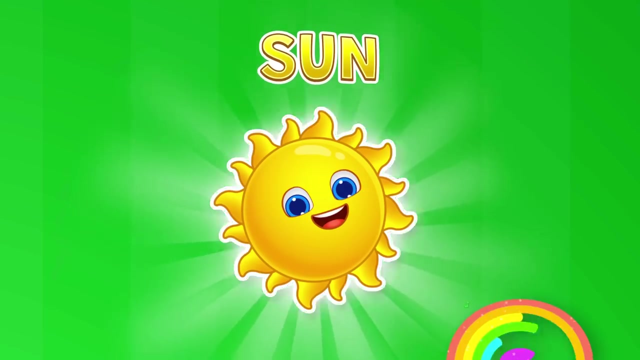 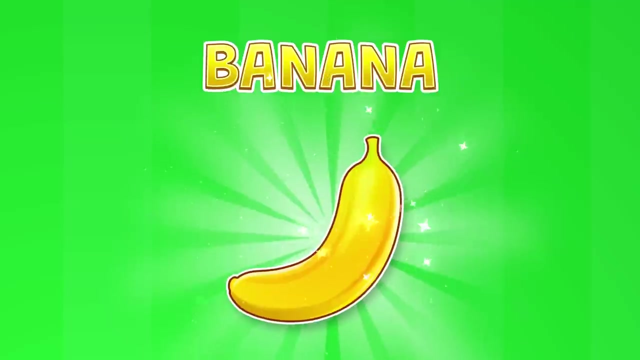 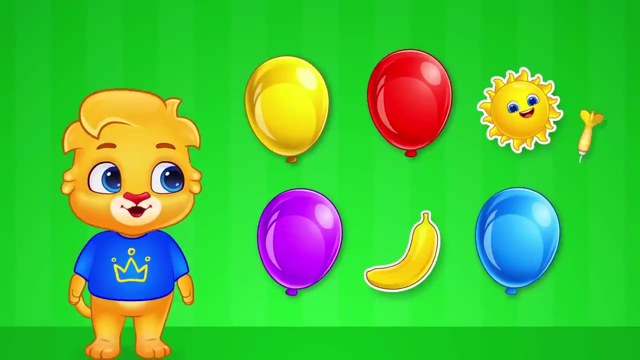 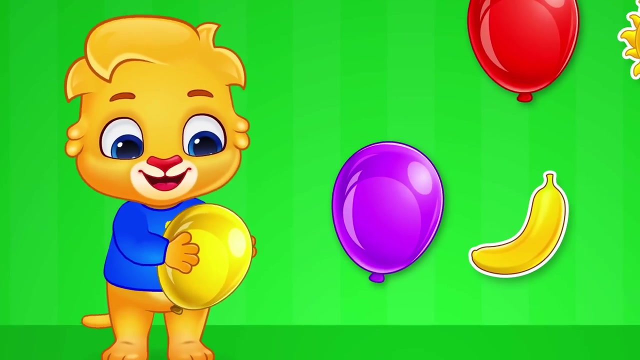 Hey friends, look six balloons. Hey friends, Yellow balloons. Who's ready to pop them? Woah, Yellow balloons, Who's ready to pop them? You thi you arel you'rer. Sun is yellow. Yellow Banana is yellow, Yellow Duck is yellow. 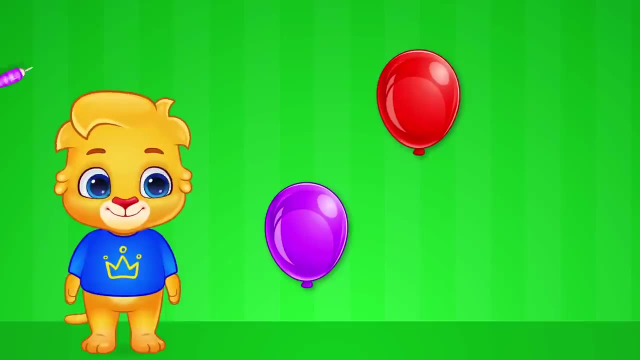 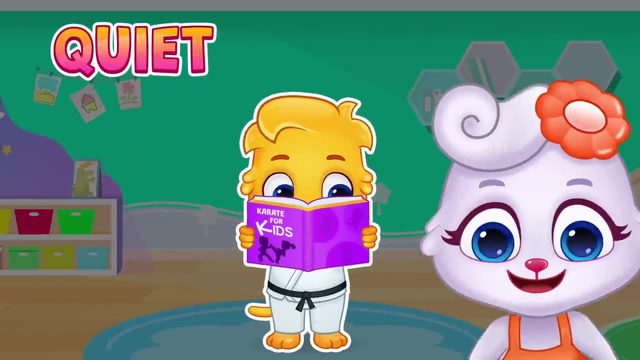 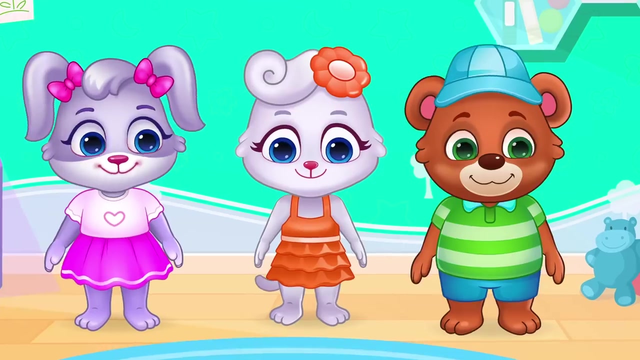 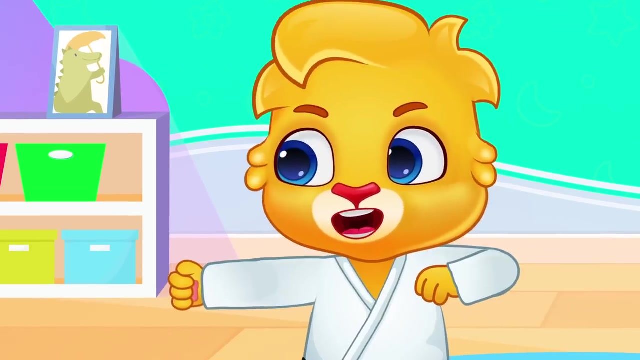 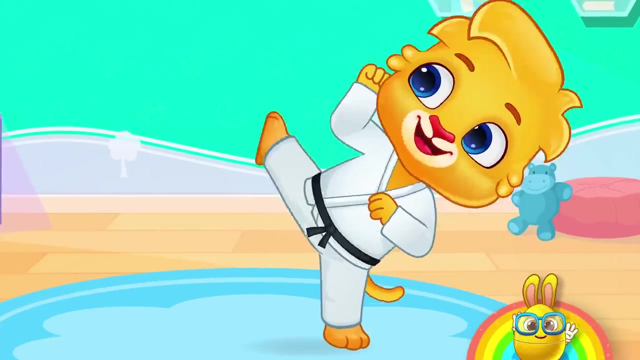 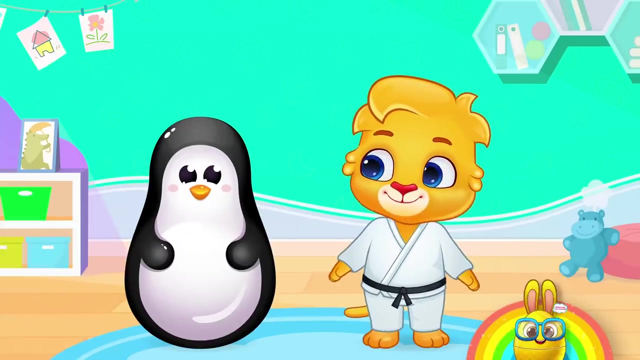 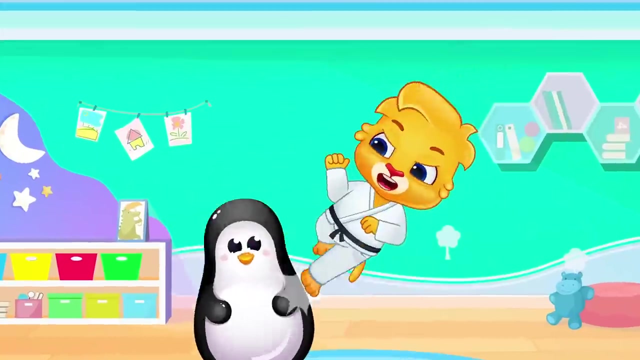 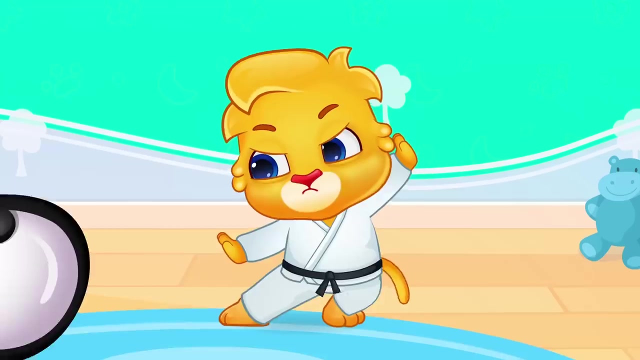 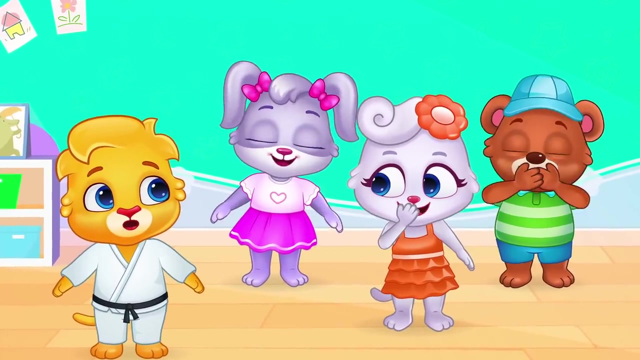 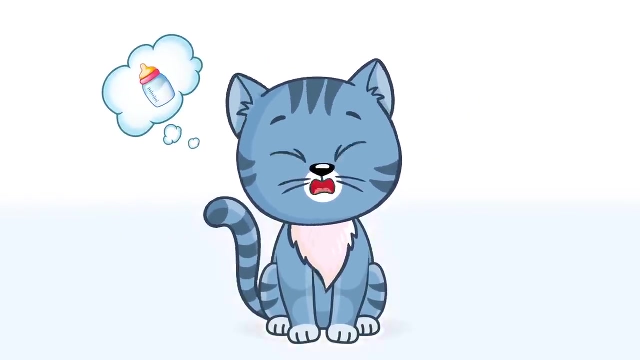 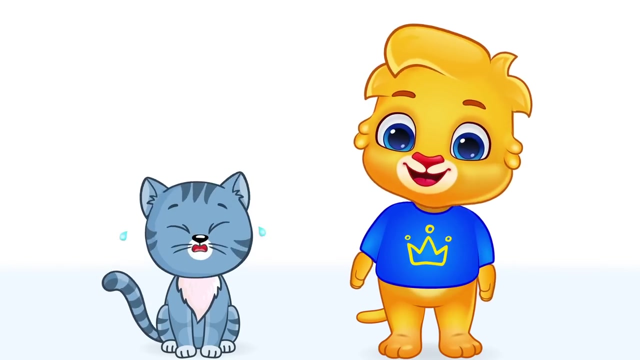 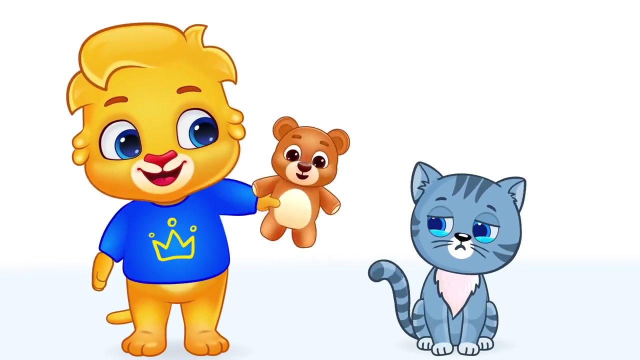 Black is black. Quiet. Lucas wants quiet. Hey, Yes, yes, yes, Meow, Meow, Clap. Lucas's friends are clapping. Ow, Oh, They're laughing Cry, Yeah, Cry, Yeah, Cry. 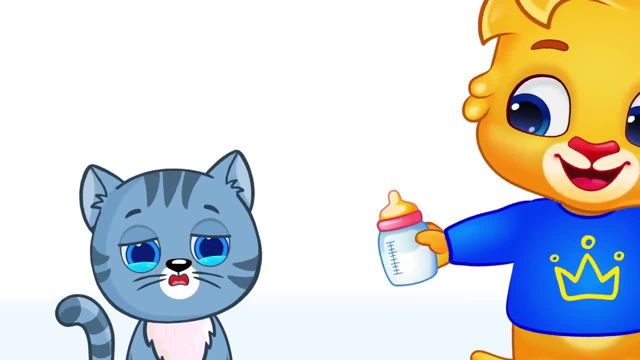 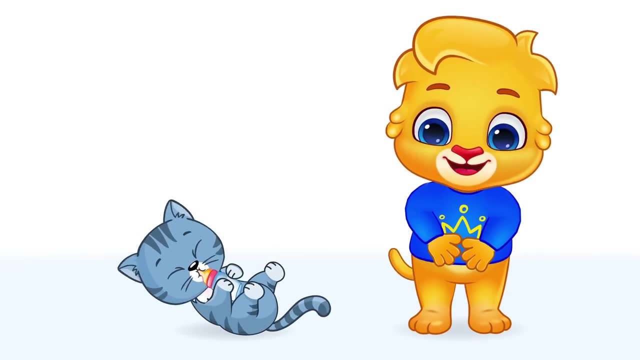 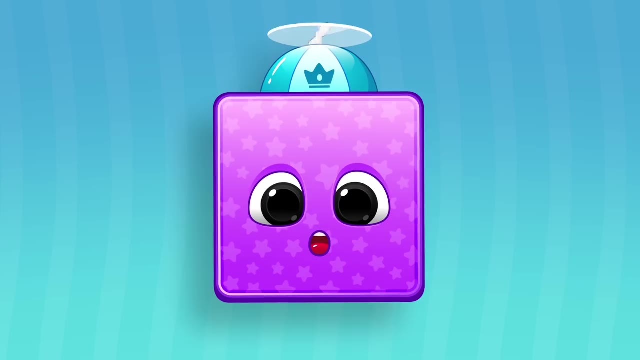 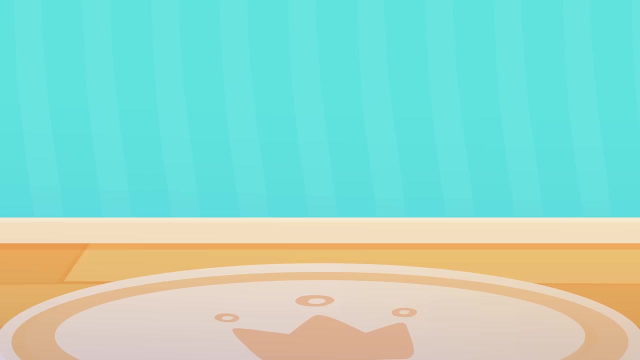 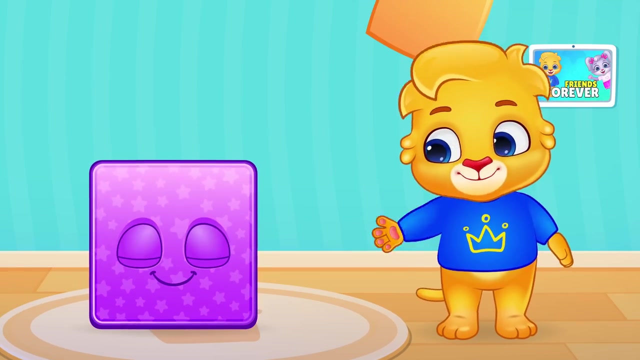 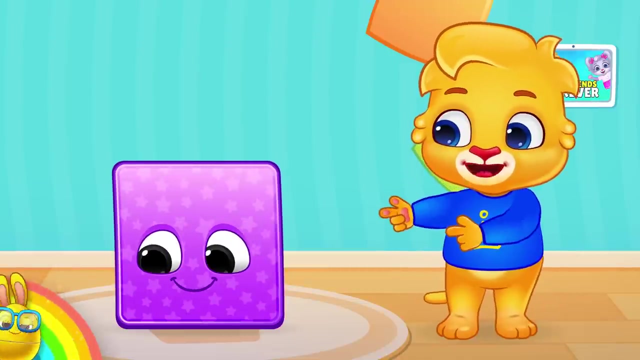 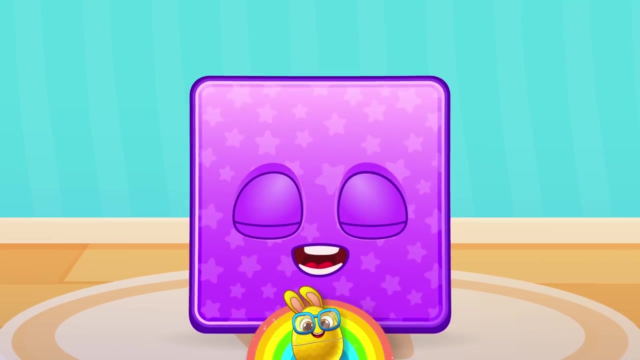 Yeah, Wow, La-la-la-la-la-la. Hello Yeah, Aha, Hello, Hello. I'm Lucas. Oh, What shape is this? Hmm, Will you help me please Square? Yeah, Yeah, Huh. 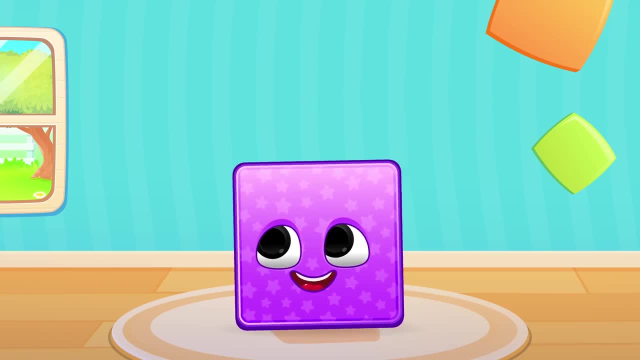 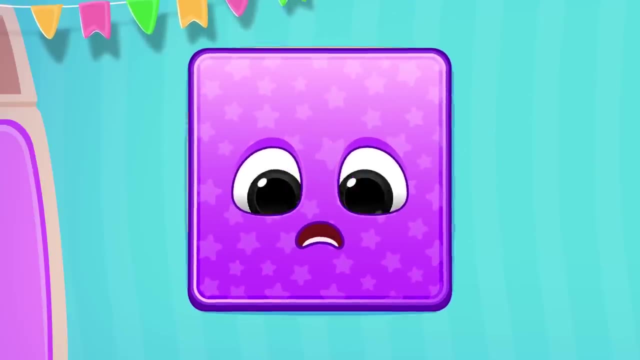 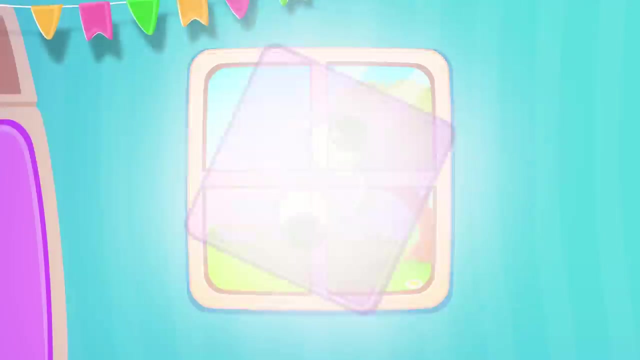 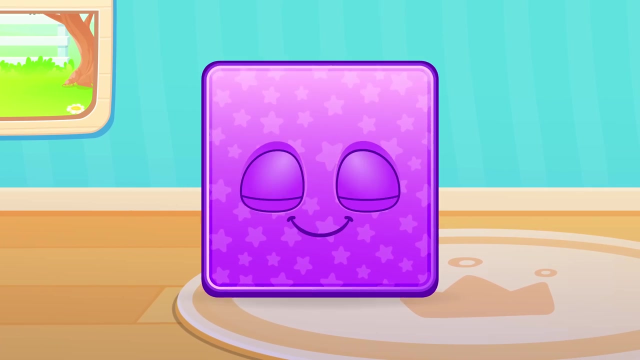 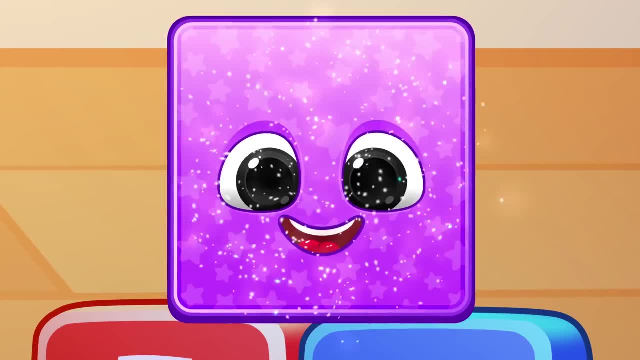 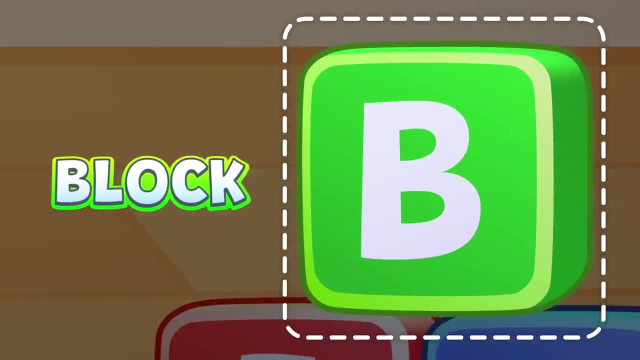 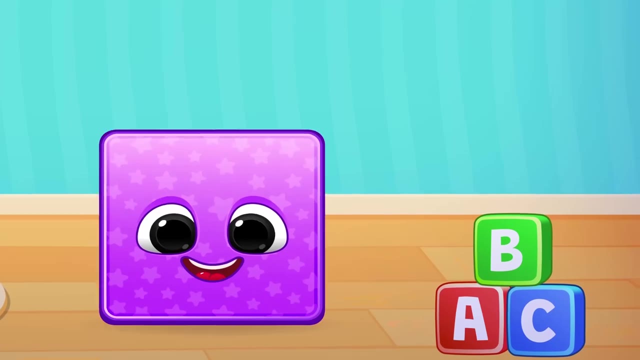 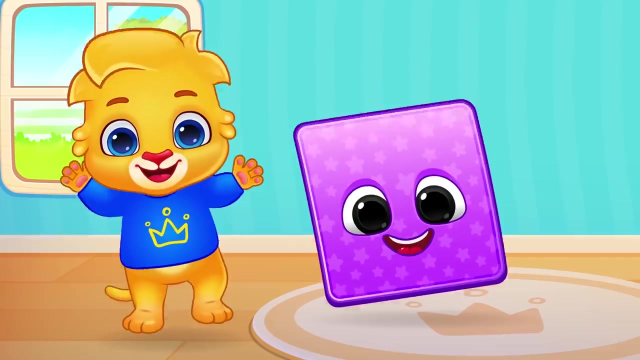 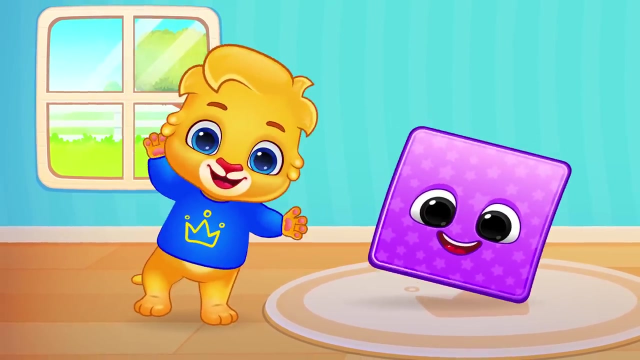 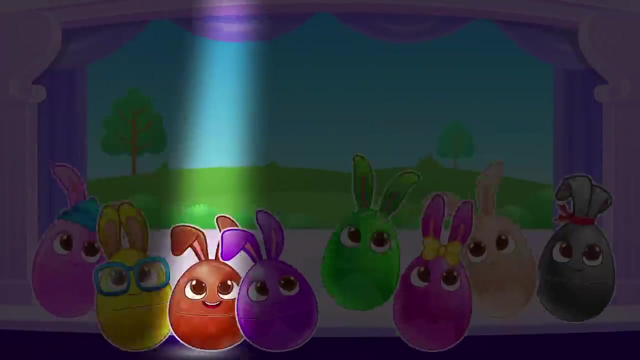 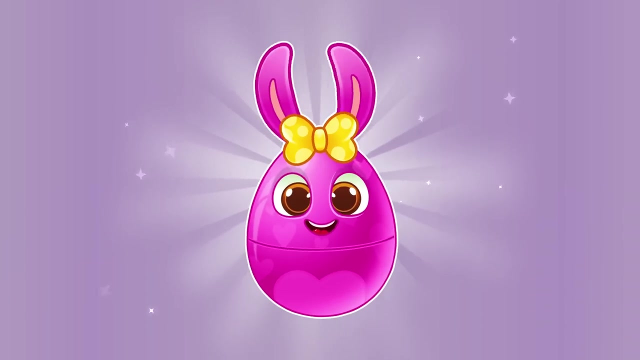 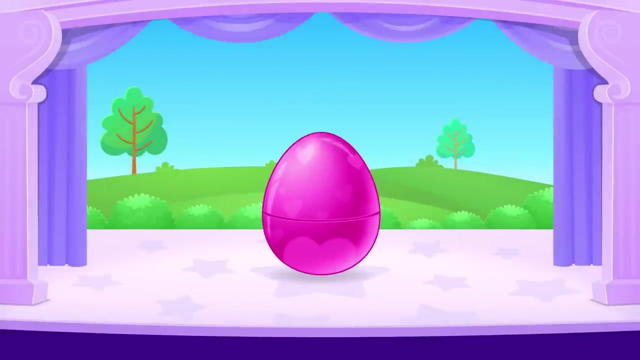 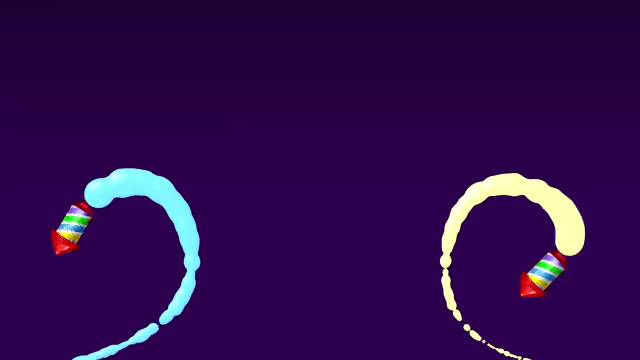 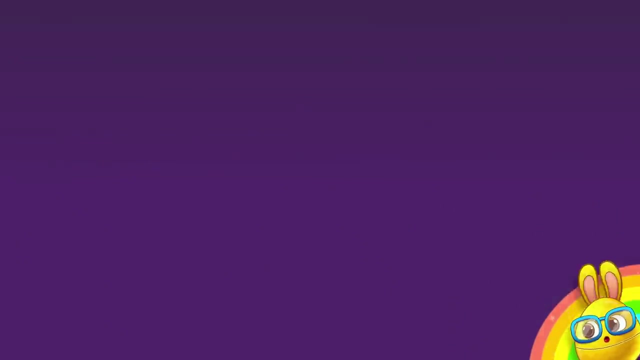 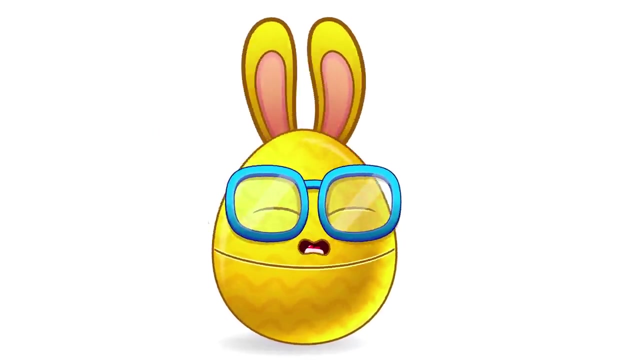 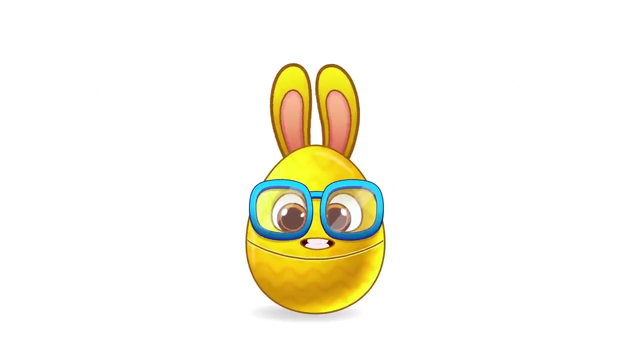 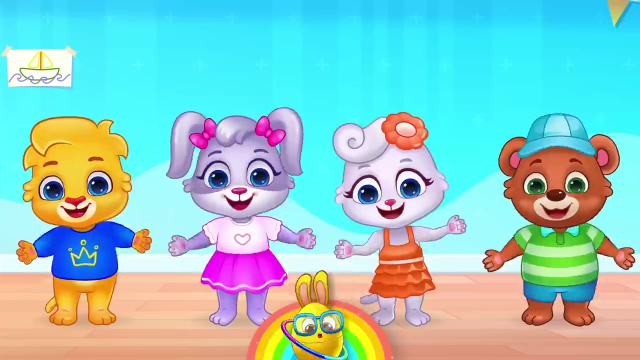 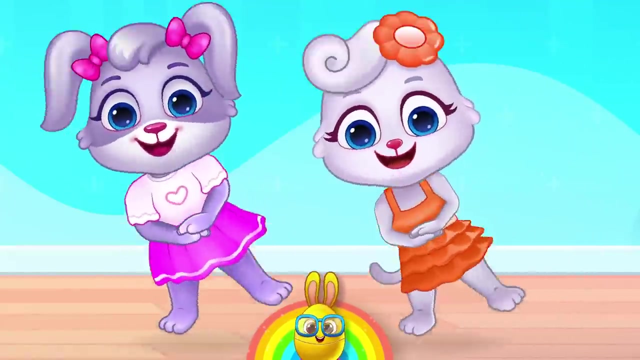 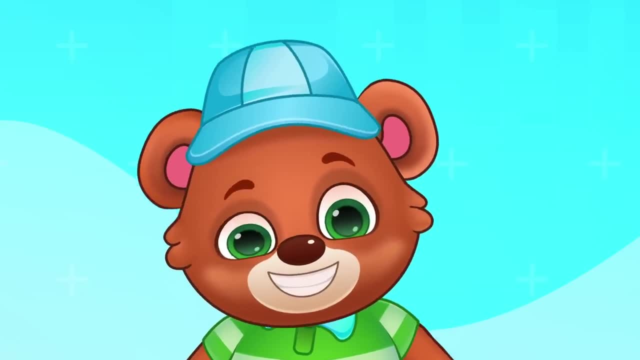 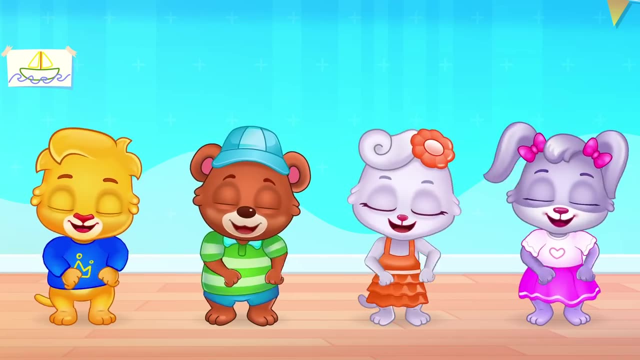 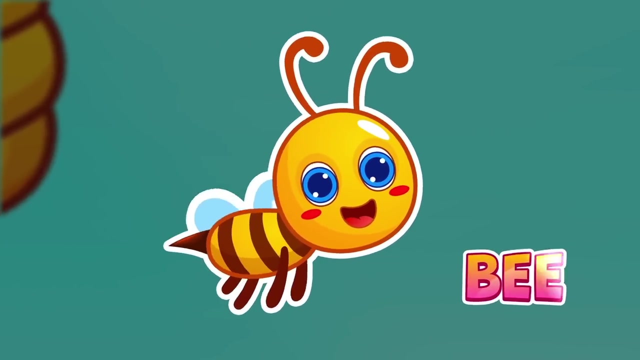 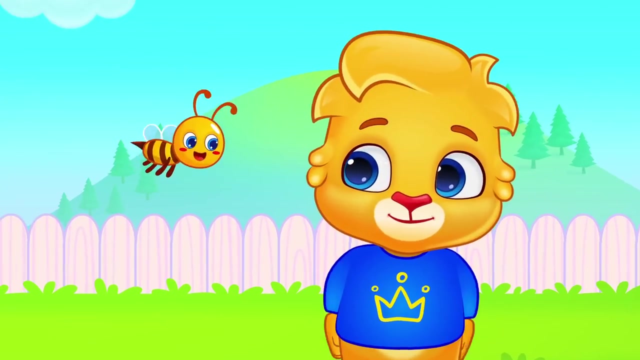 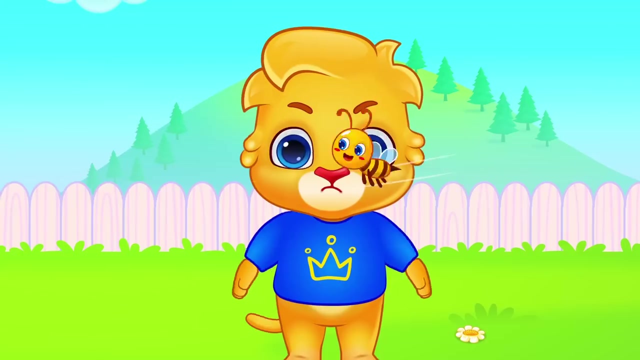 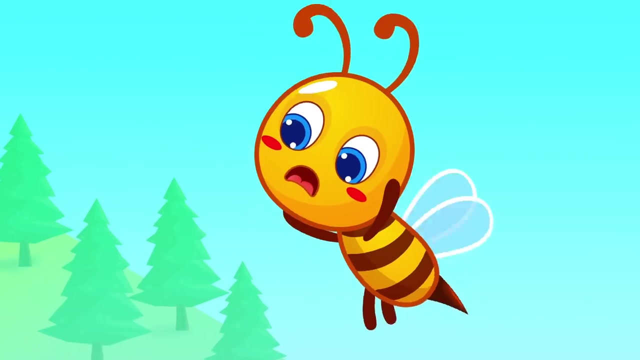 If you're happy and you know it, then your face will surely show it. If you're happy and you know it, clap your hands. This is a bee. Bees live in a hive. Bees live in a hive. Lucas is running behind the bee. 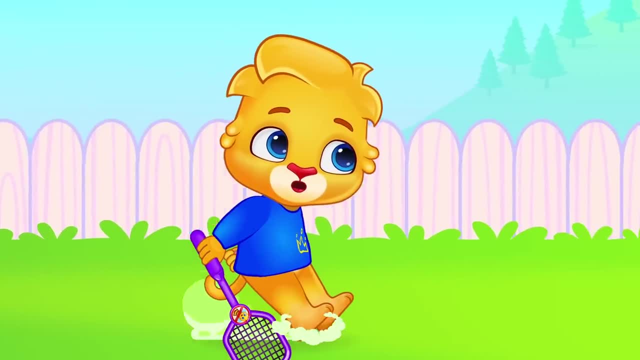 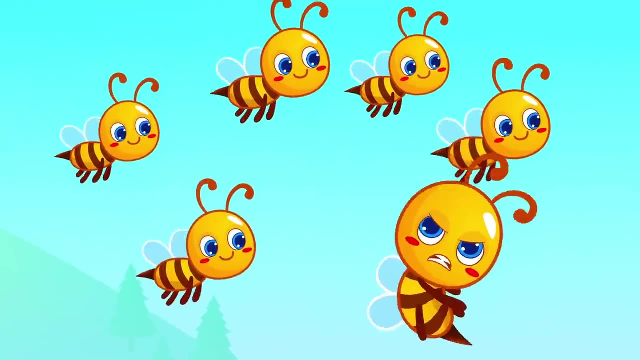 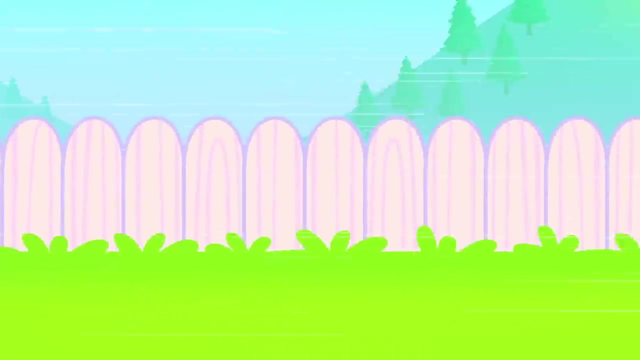 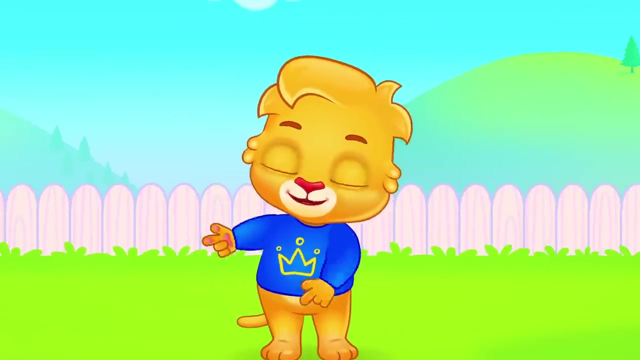 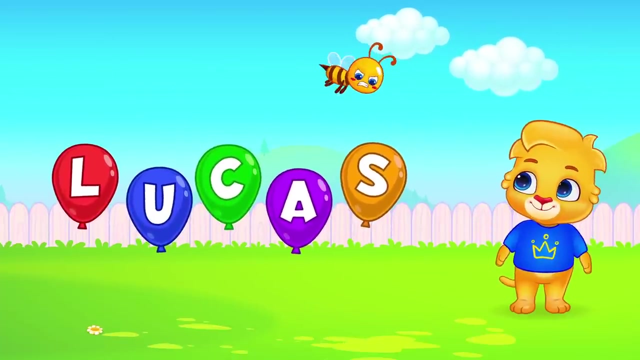 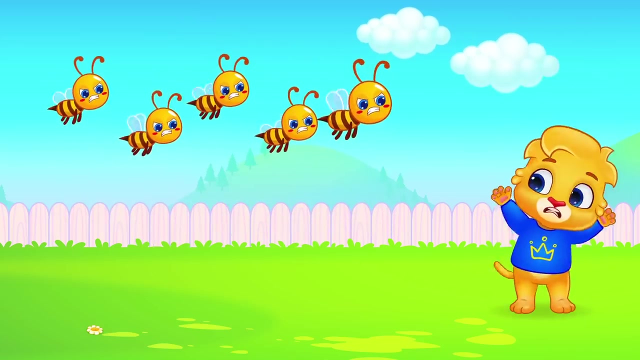 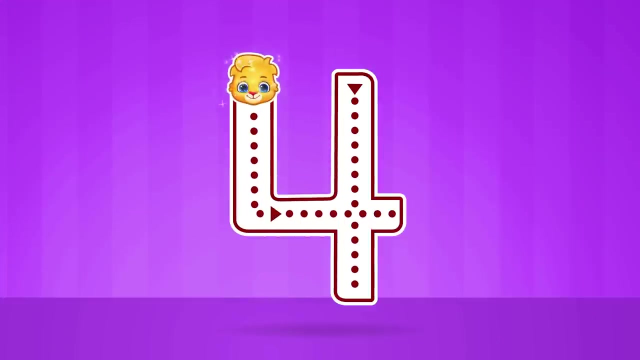 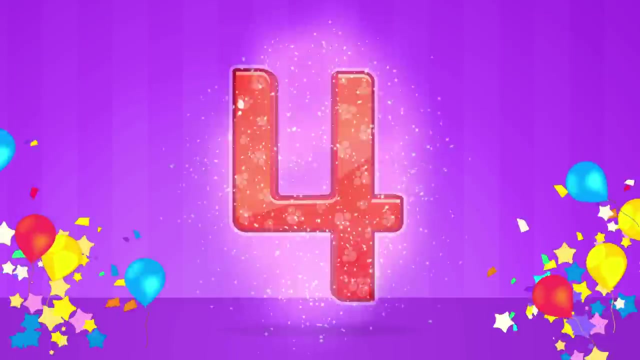 Bees live in a hive. Bees live in a hive. Hi, I'm Lucas. It's spelt L-U-C-A-S. It's Lucas. Hey, stay here. Good day, Good day, Yeah, Yeah More. 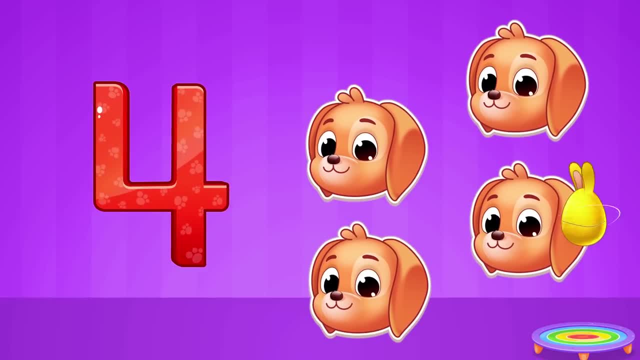 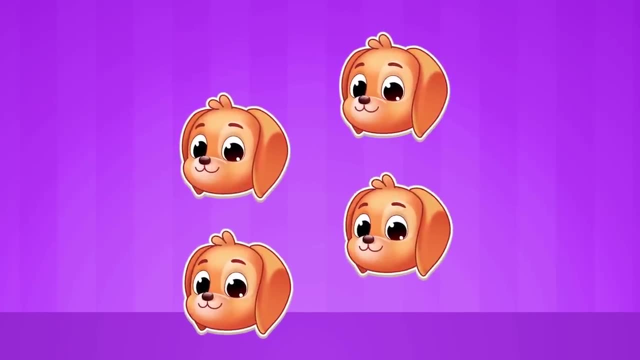 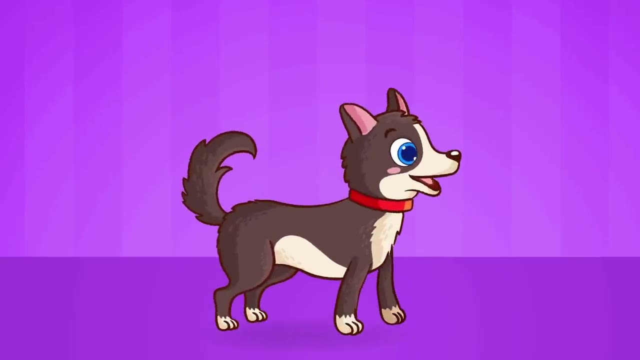 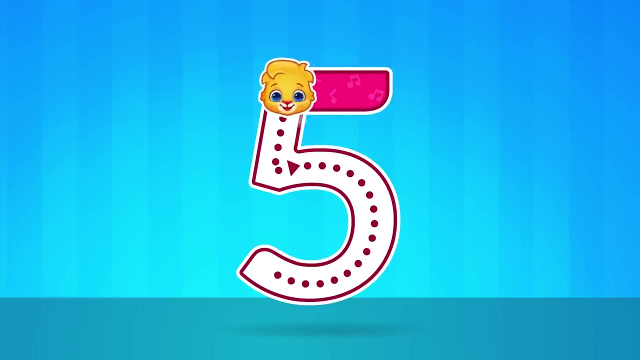 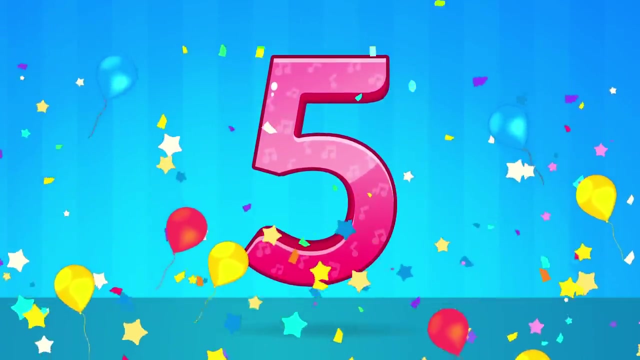 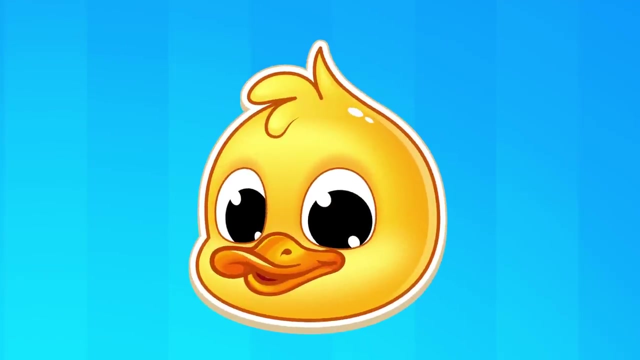 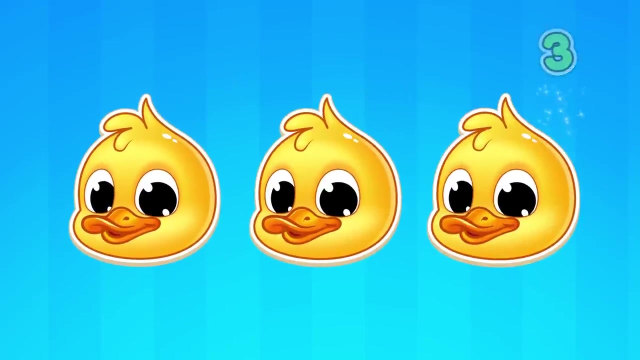 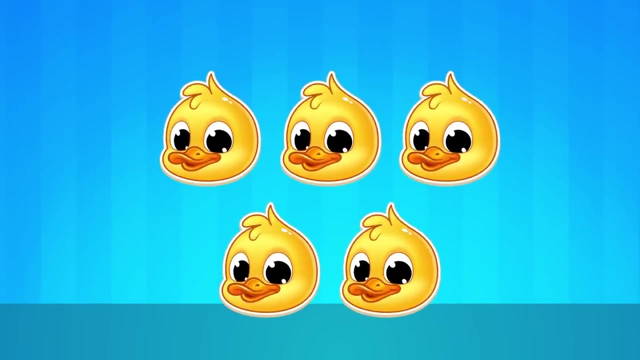 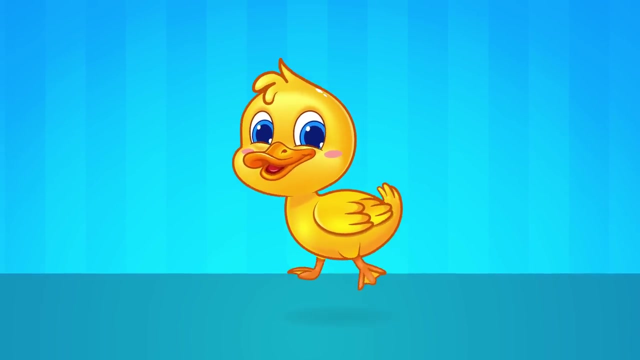 Dogs: Four dogs: One, two, three, four, Four dogs. Yeah, Yeah, Yeah, Dogs Ducks, Five ducks: One, two, three, Four and five, Five ducks. Quack, quack, quack. 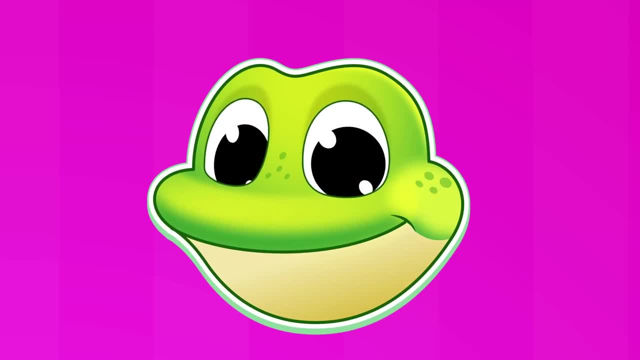 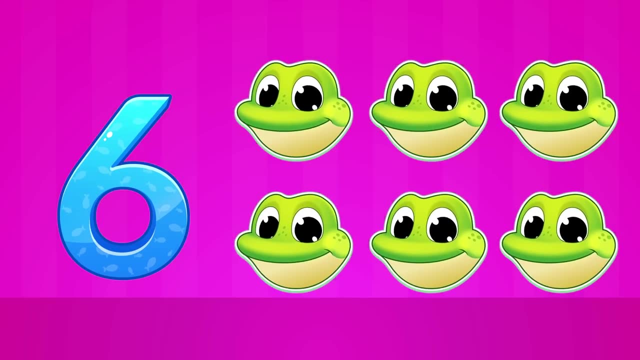 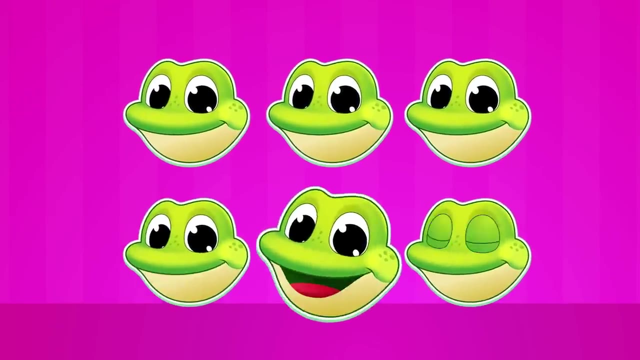 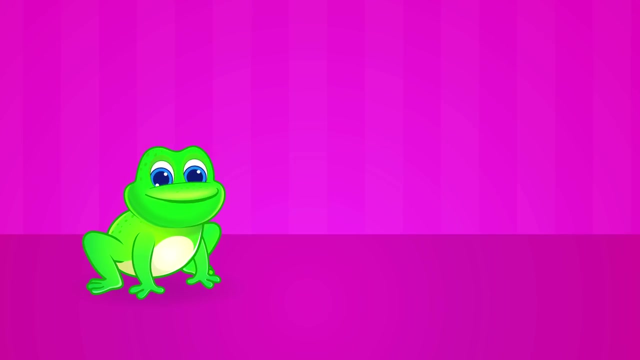 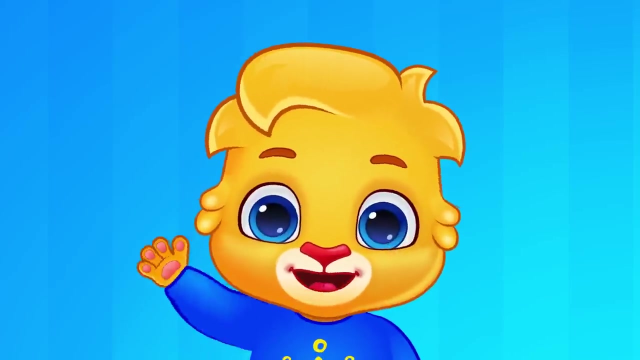 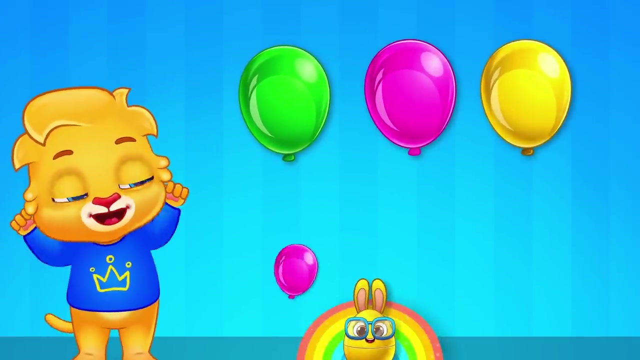 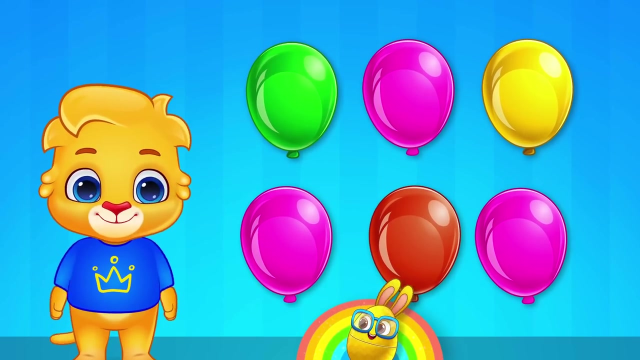 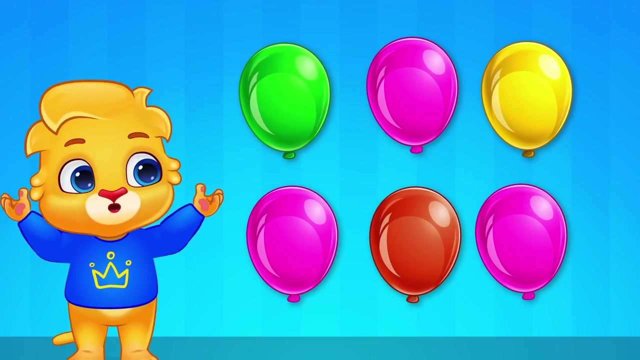 Six Frogs, Six frogs. One, two, three, Four, five, six, Six frogs. Hi friends, Woo-hoo, Yeah, Yeah, Look, Six balloons, Hey friends, Pink balloons. Who's ready to pop them? 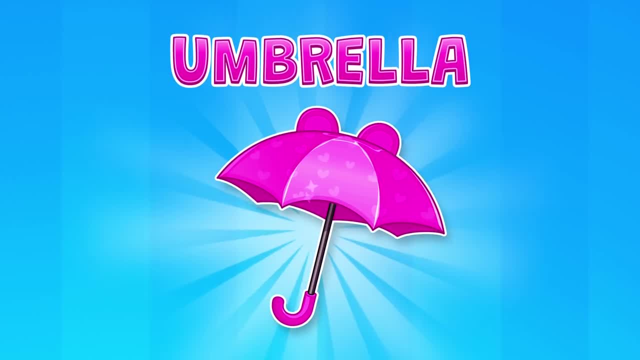 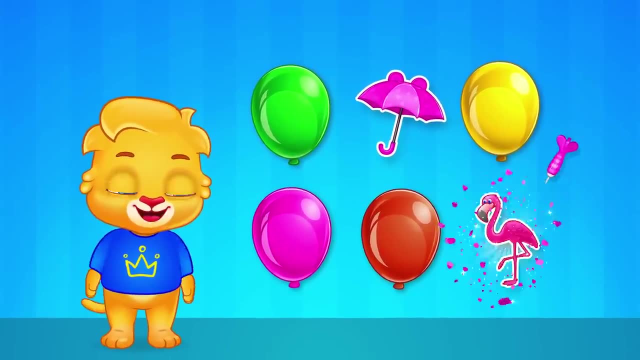 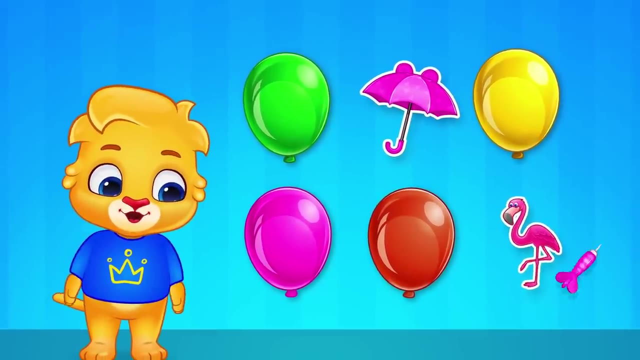 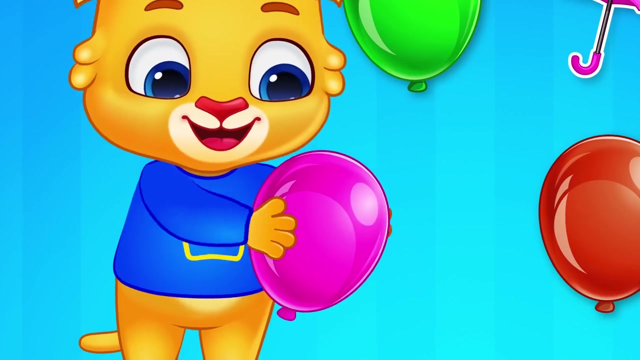 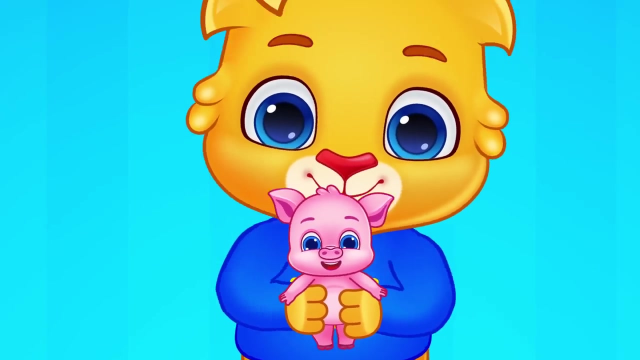 Oh, Pink Umbrella is pink, Pink Flamingo is pink. Ha-ha, Oh, No, no, no, no, no, no, Pink, Yeah, Pink is pink. Woo, What Ha-ha-ha? 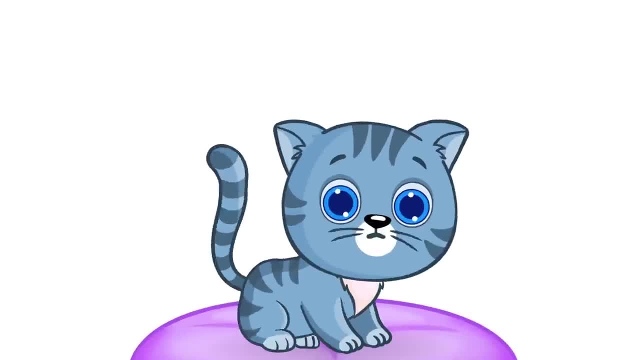 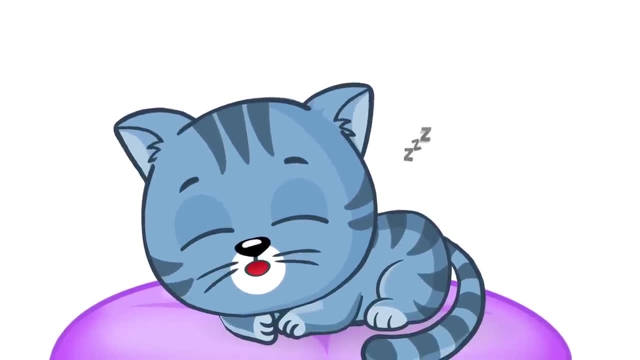 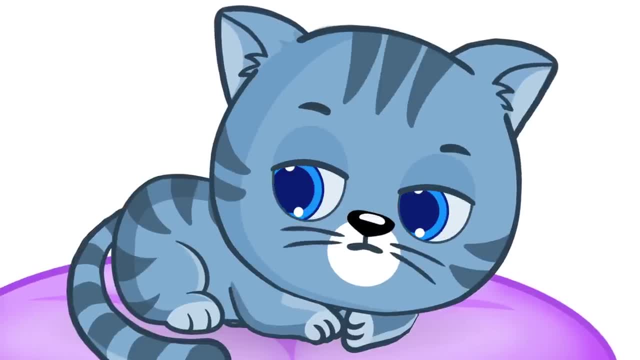 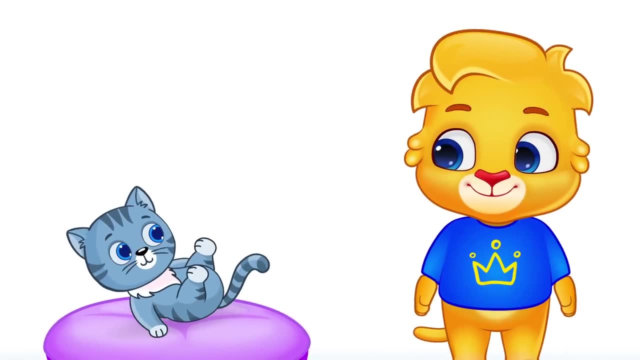 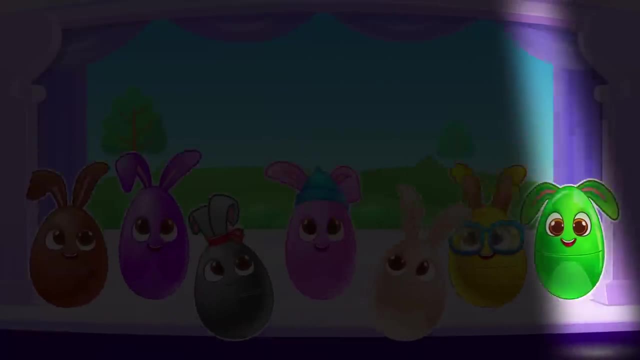 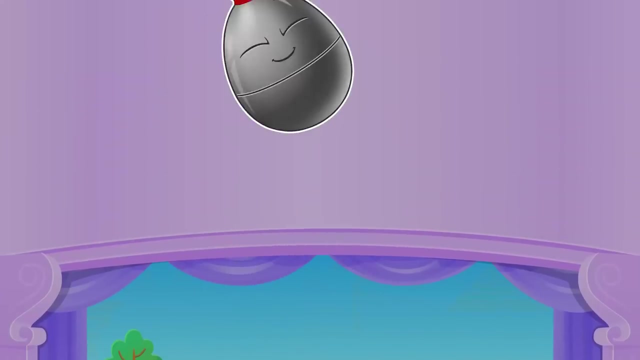 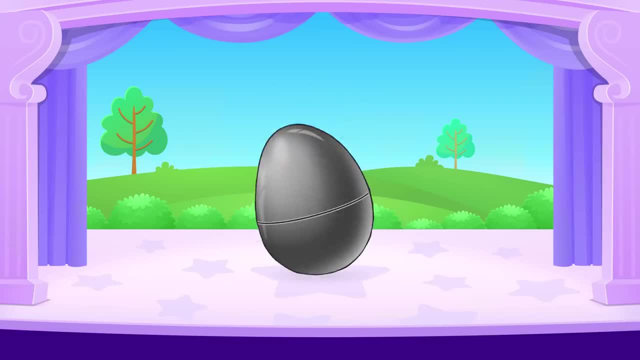 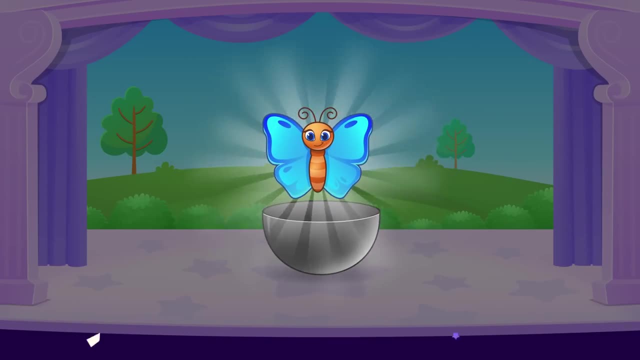 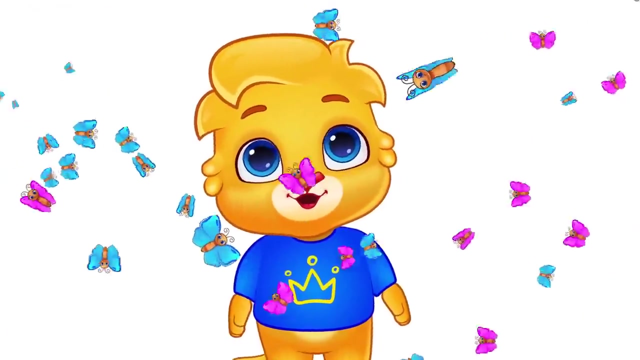 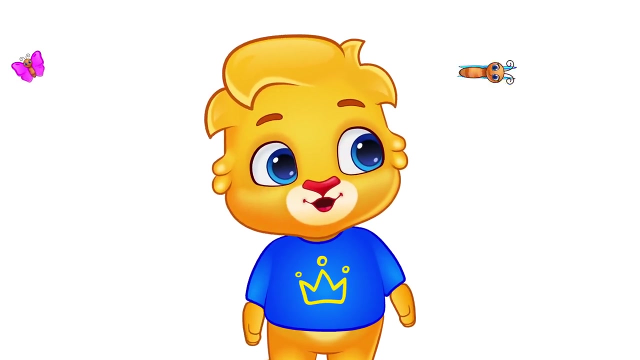 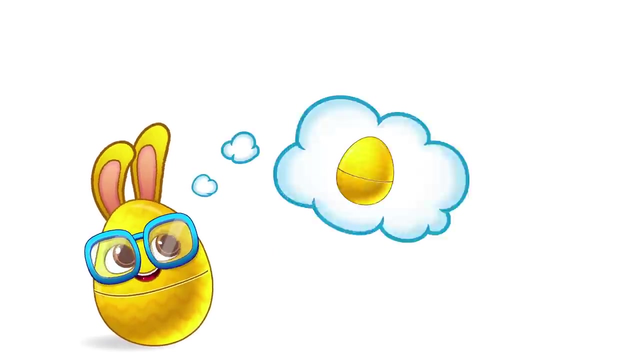 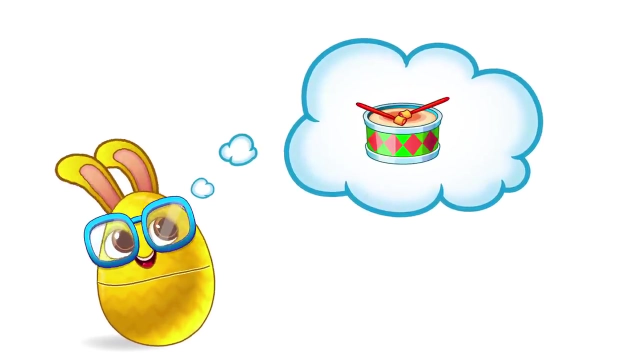 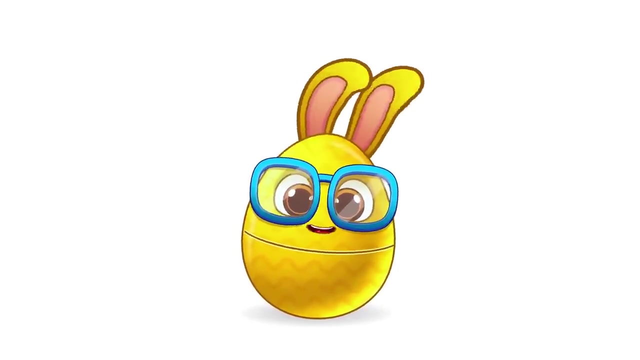 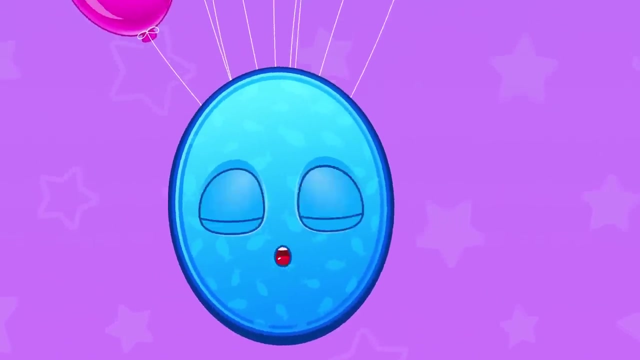 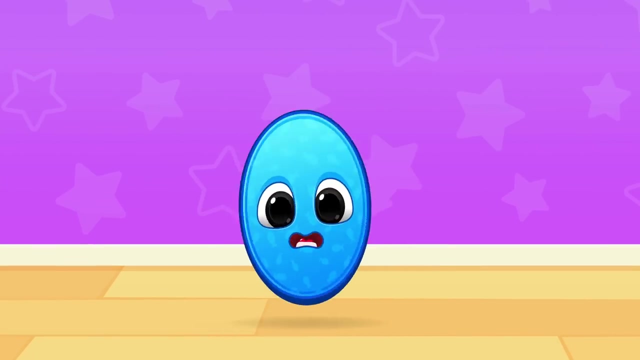 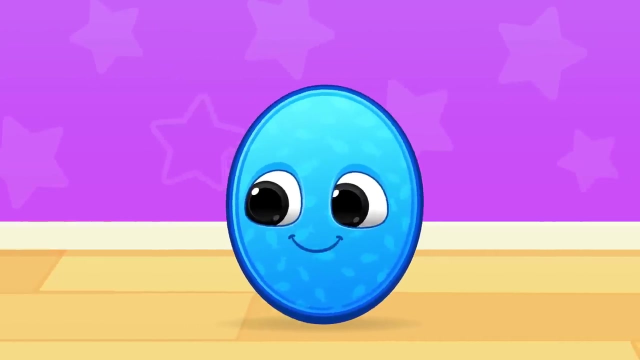 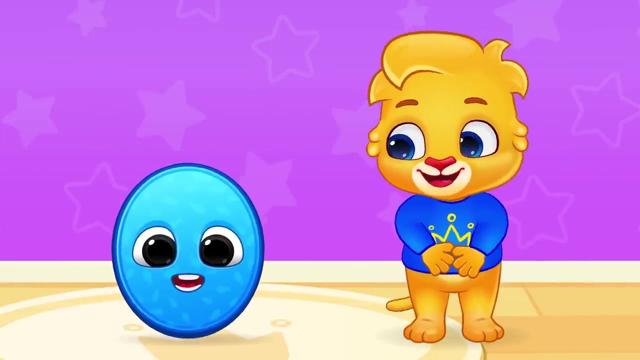 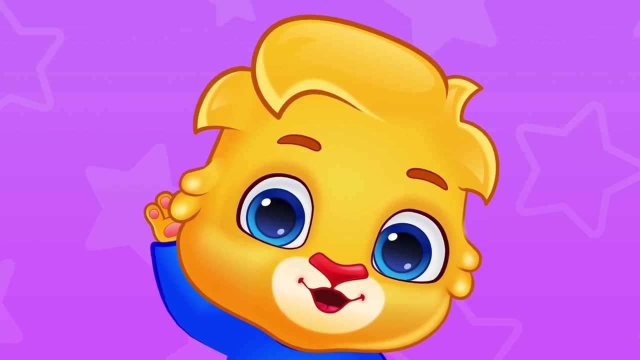 Huh, Huh, Yeah, Oh my God, Oh, Aha, Come on, pick me so that you can have one of these and have fun with it. Do you know what shape is this? Hmm, Oval, Yeah. 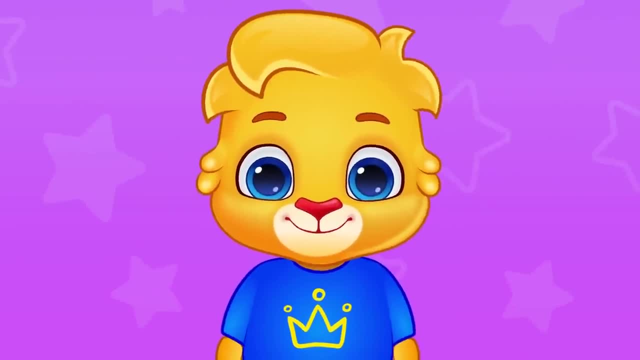 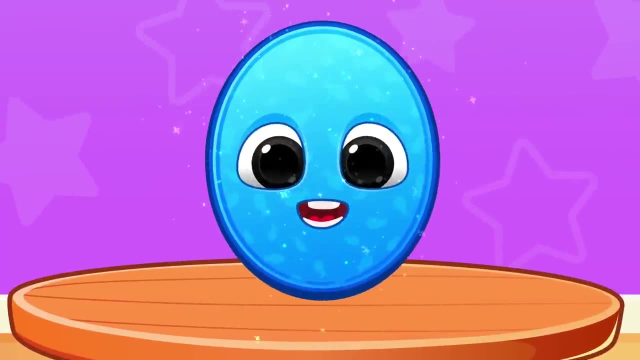 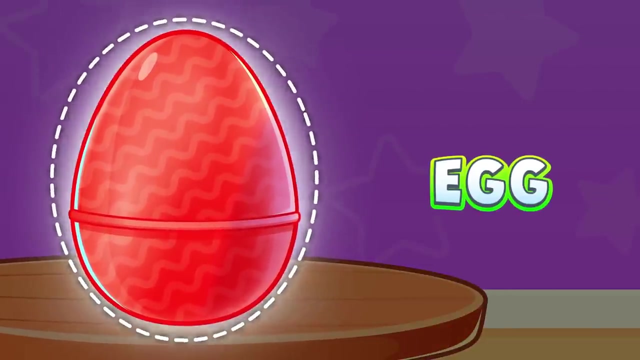 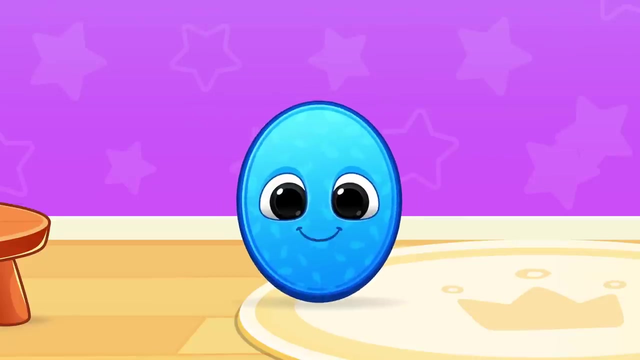 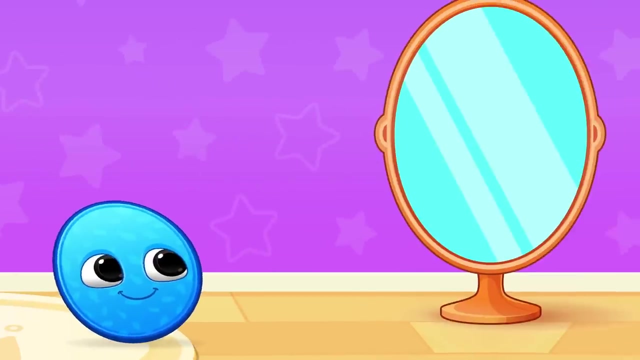 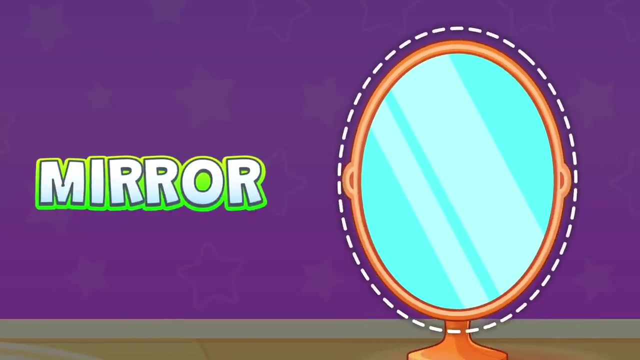 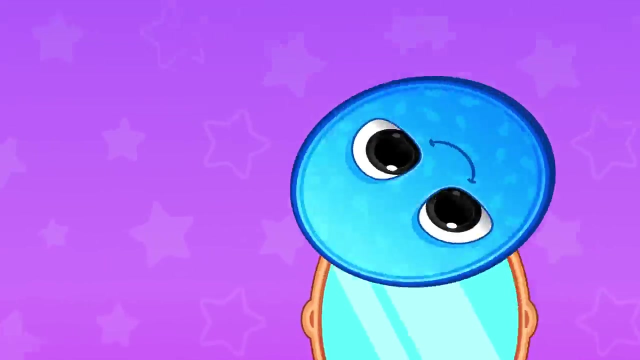 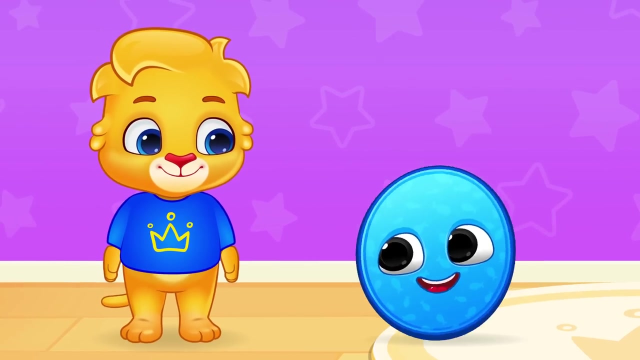 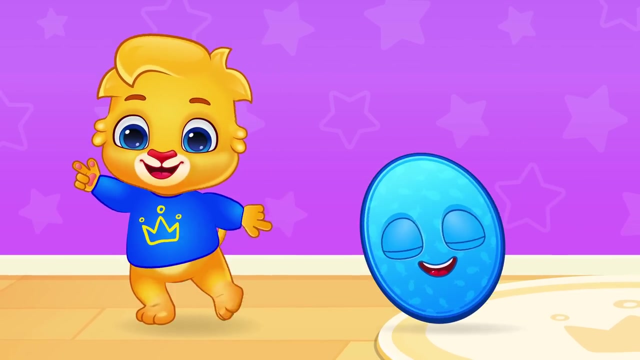 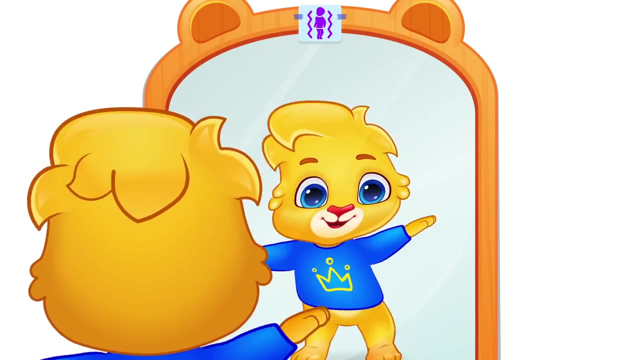 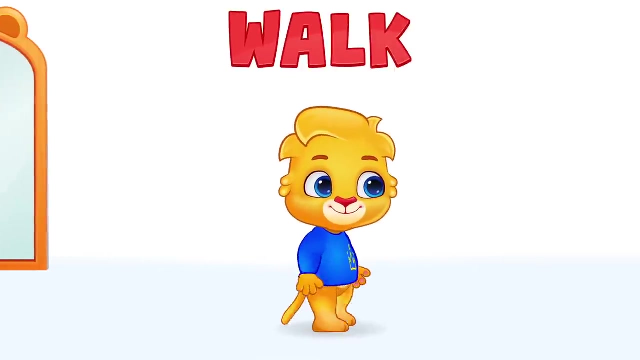 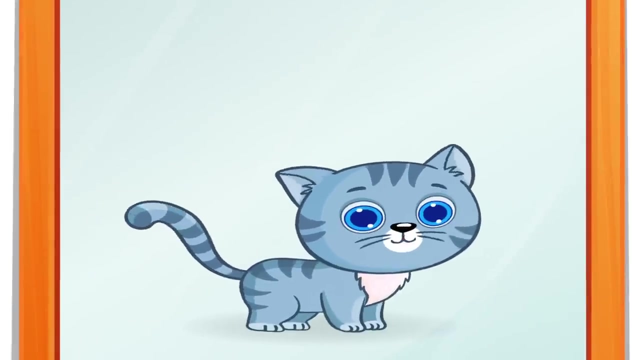 Yes, you are right, my friend. An egg is oval, Yay, A mirror is oval, Yay, Yay, Yay, Walk, Walk Wow, Meow, Meow, Meow, meow meow. 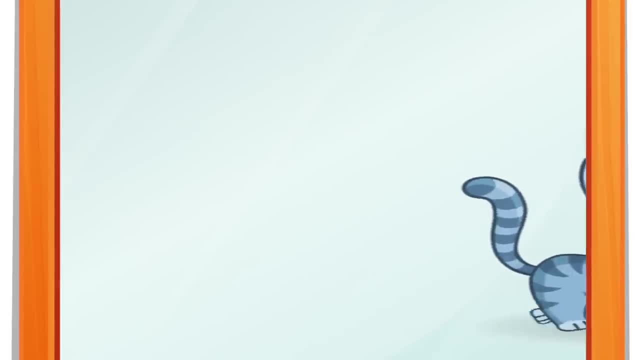 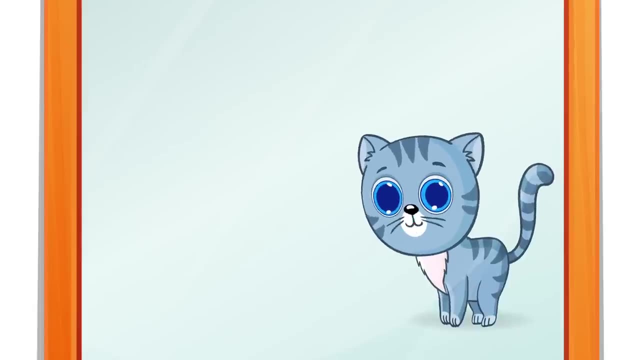 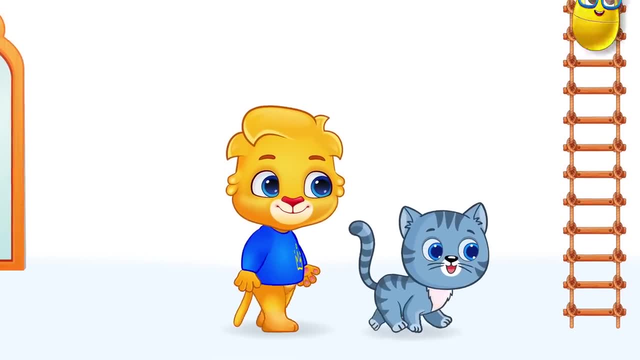 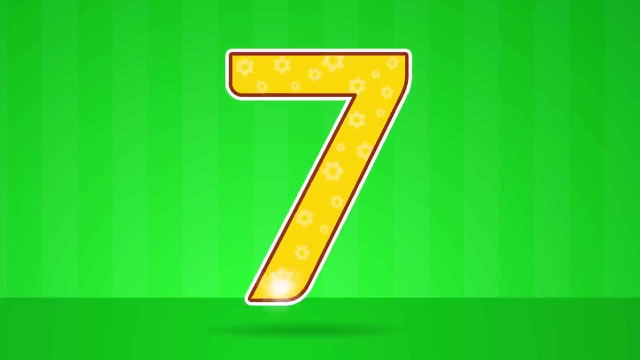 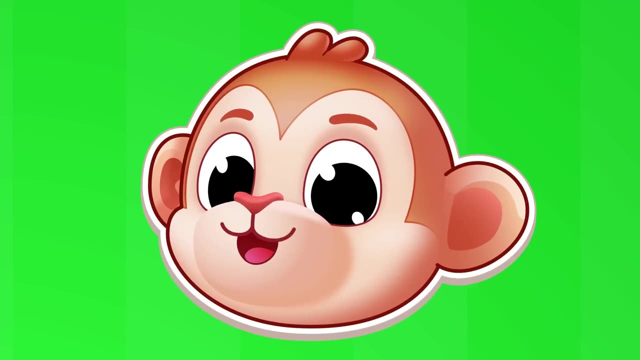 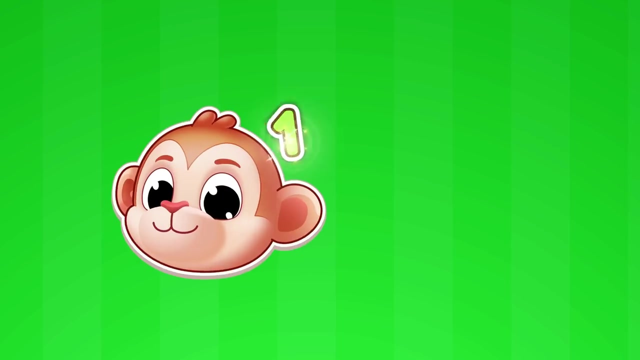 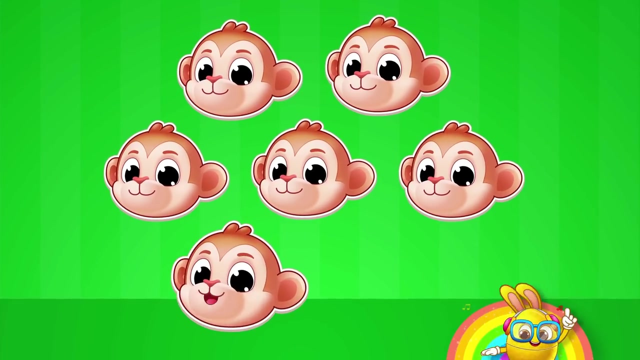 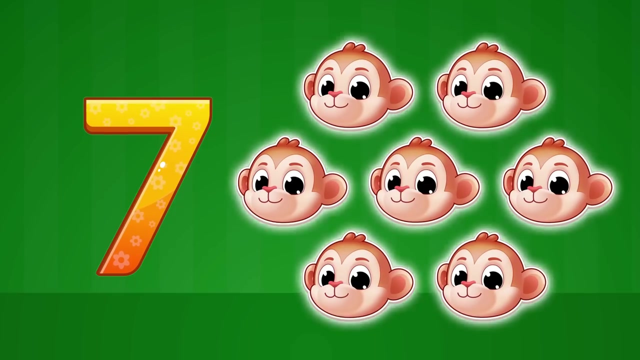 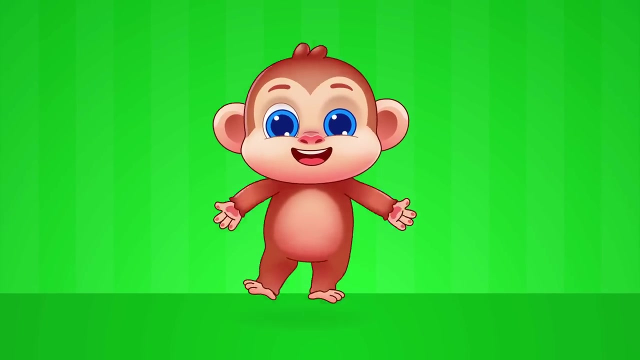 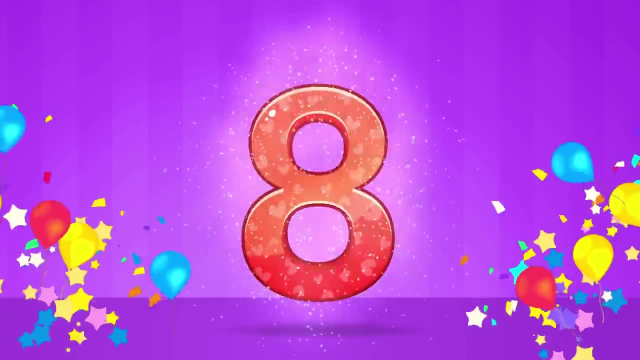 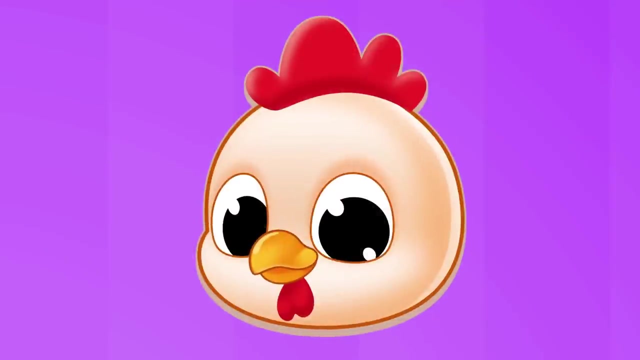 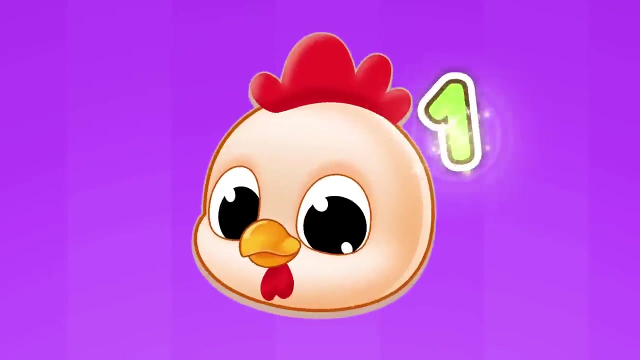 Yeah, Yeah, Yeah, Seven Monkeys. Seven Monkeys. One, two, three, Four, five, six, Six And seven. Seven monkeys, Yeah, Eight Hens. Eight Hens: One, two, three, four. 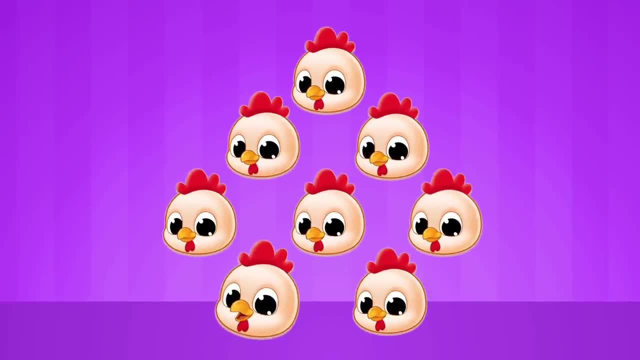 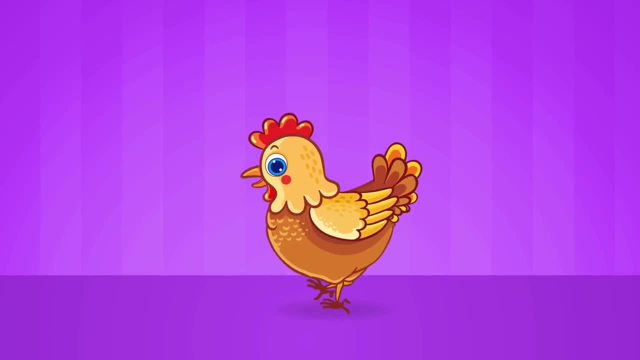 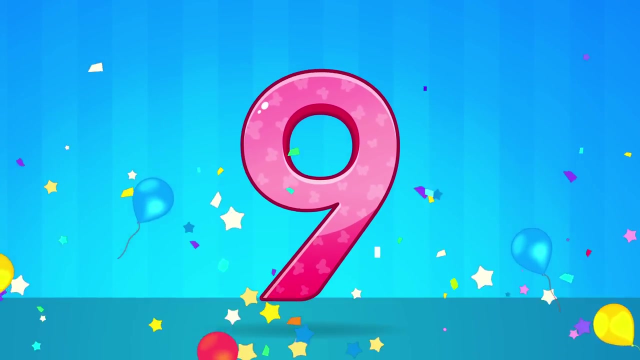 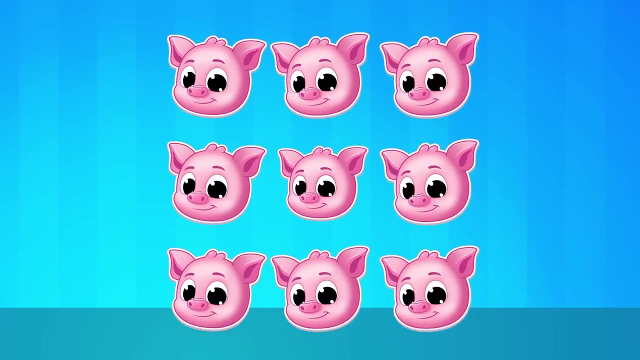 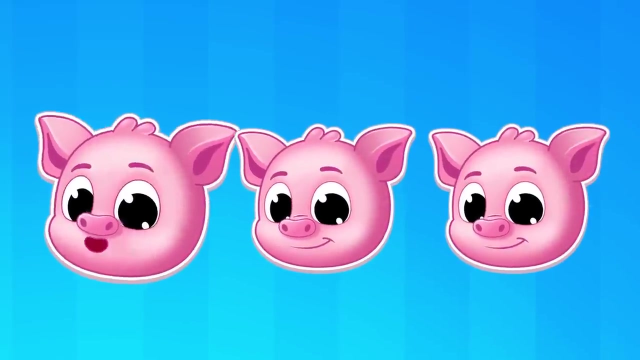 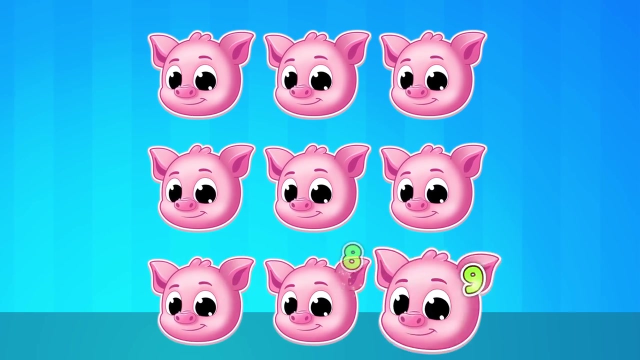 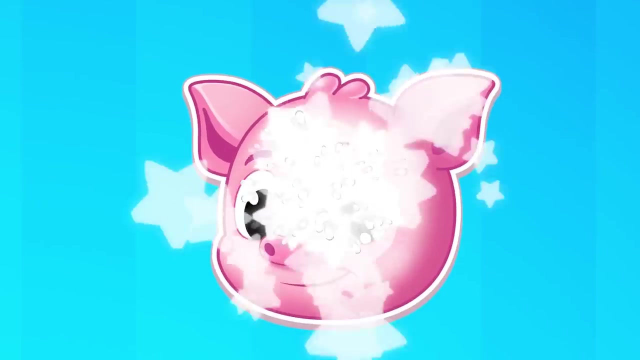 Five, six, seven, eight, Eight Hens. Yeah, Yeah, Nine Pigs. Nine pigs: One, two, three, Four, five, six, Seven, eight, nine. Nine pigs. One, two, three, four. 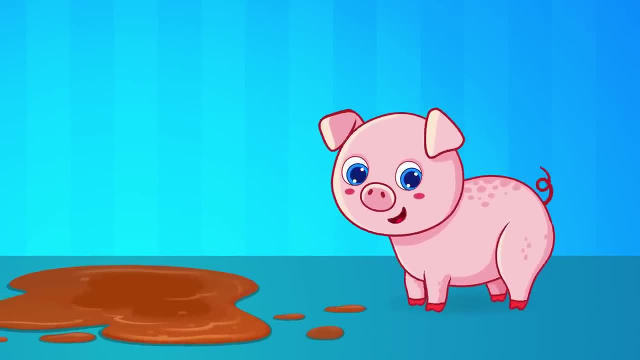 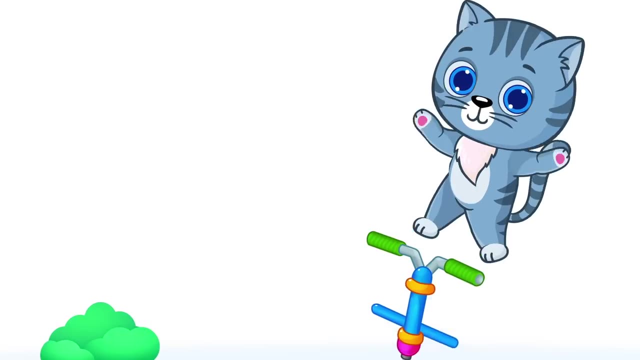 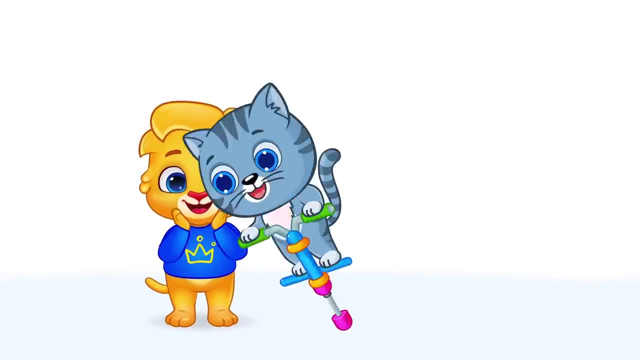 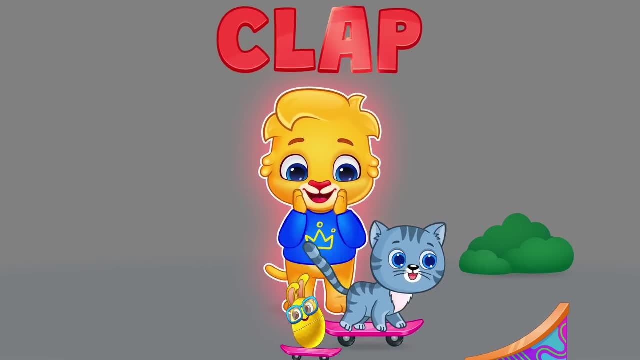 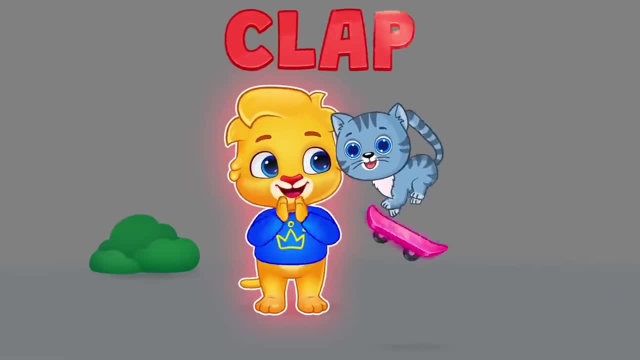 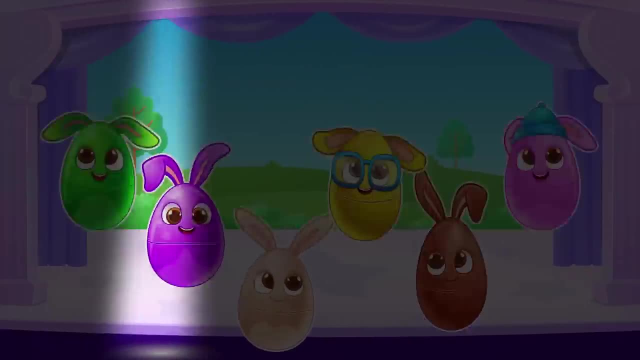 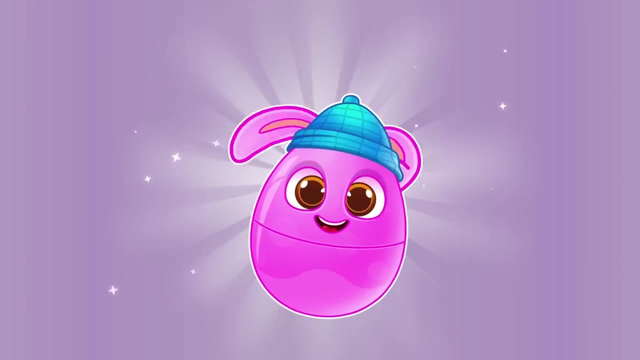 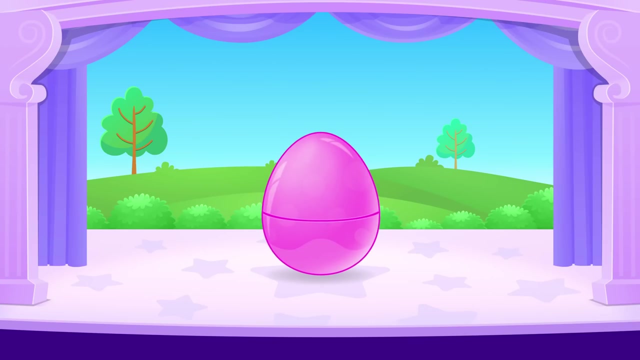 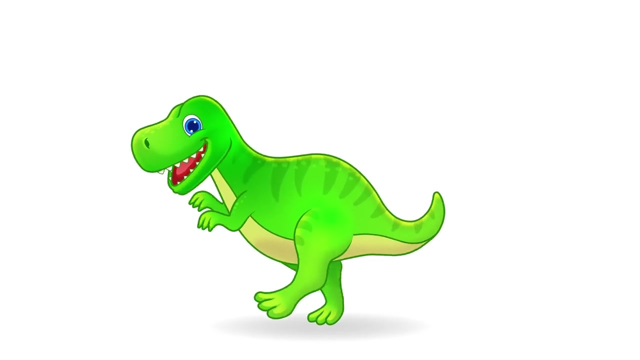 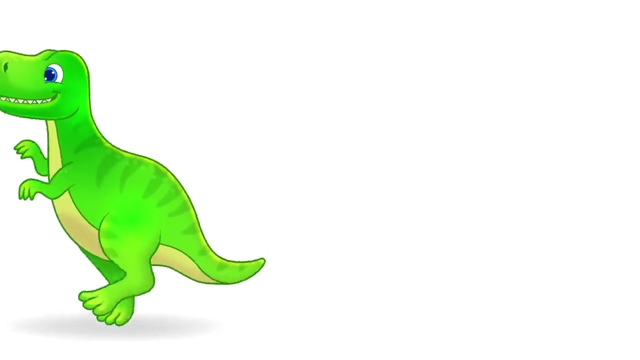 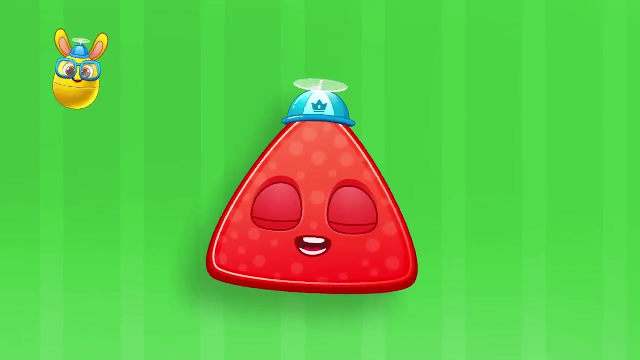 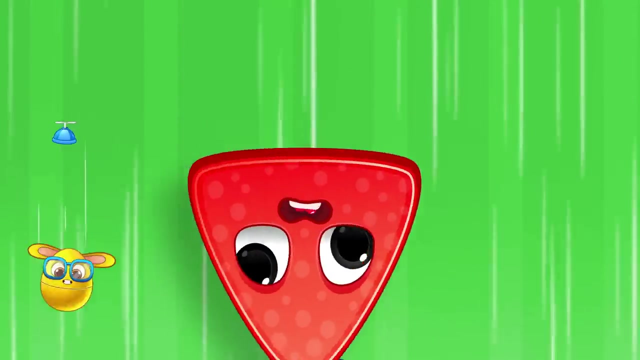 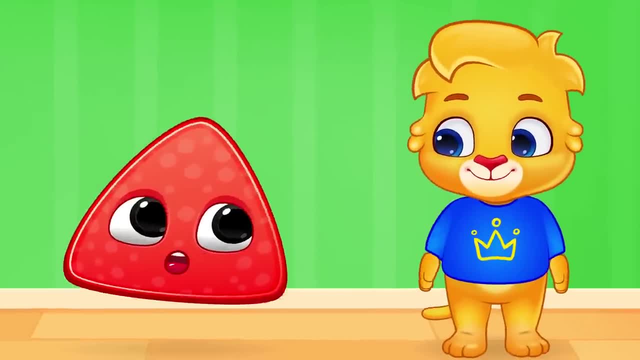 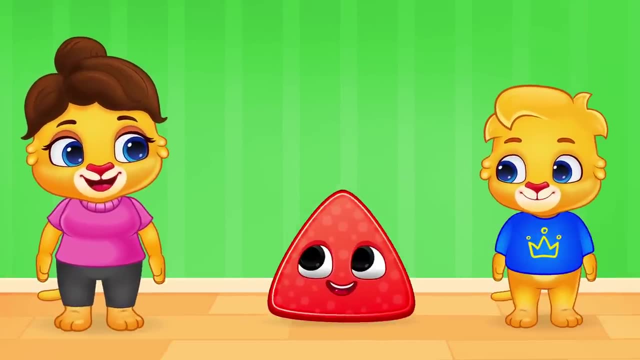 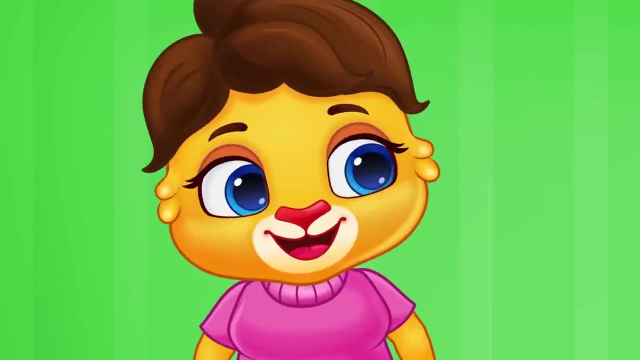 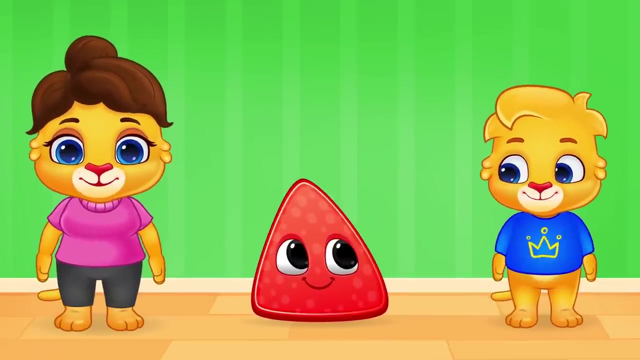 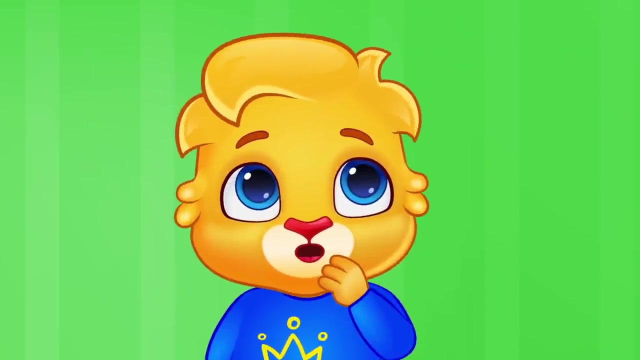 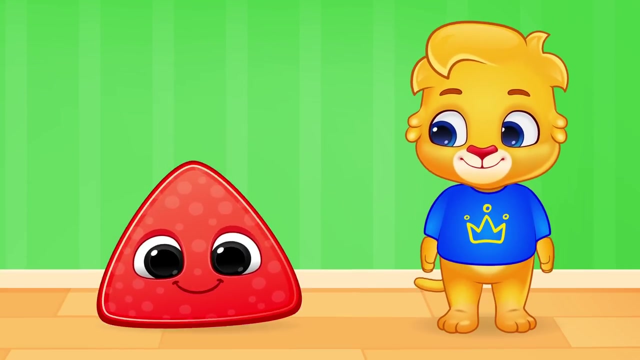 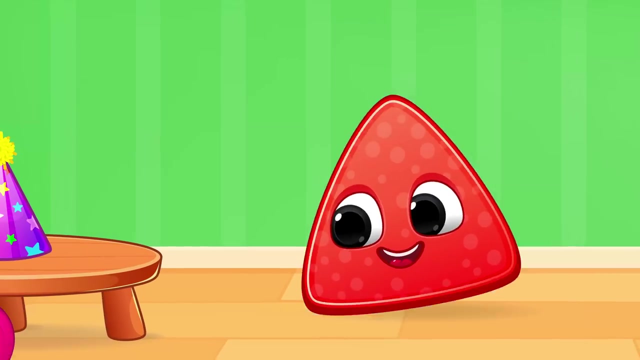 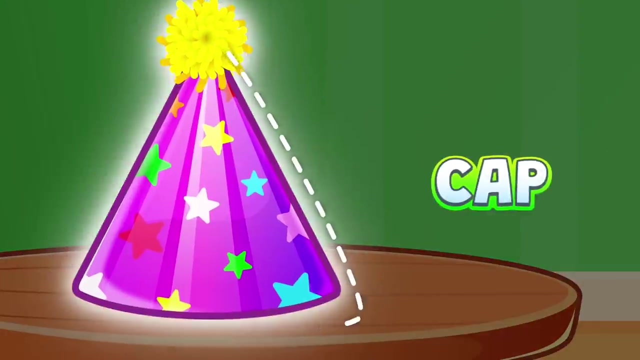 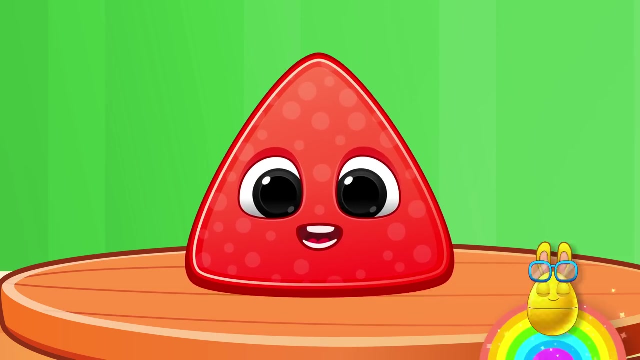 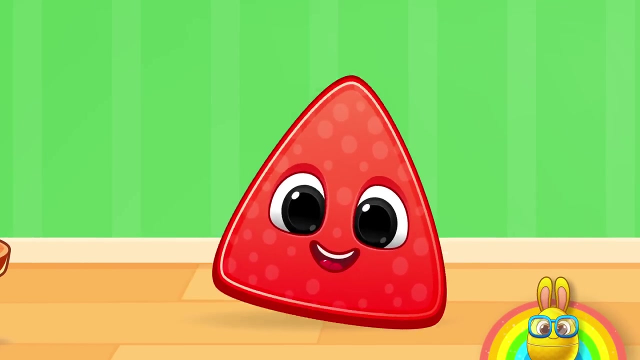 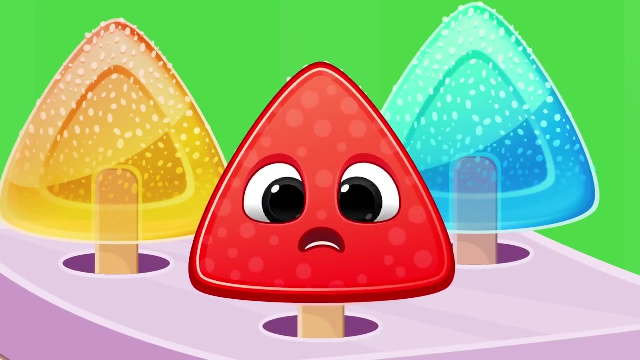 um, uh-huh, let's say hi to my mom. hey, mom, hi, i'm the mom. Oh, what shape is this? Hmm, will you help me please? Triangle, Yeah, Huh, Huh, Triangle. A cap is triangle, A candy is triangle. 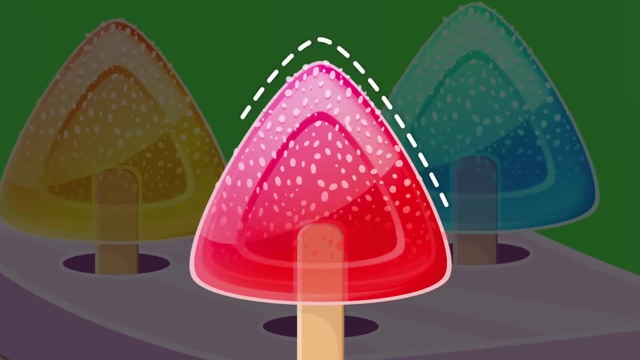 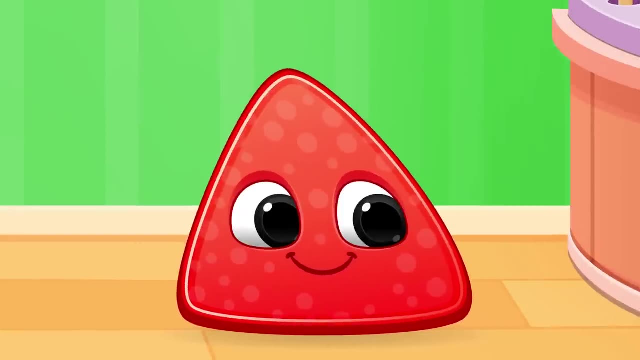 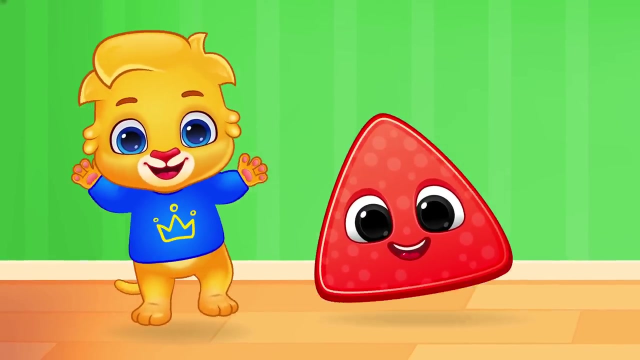 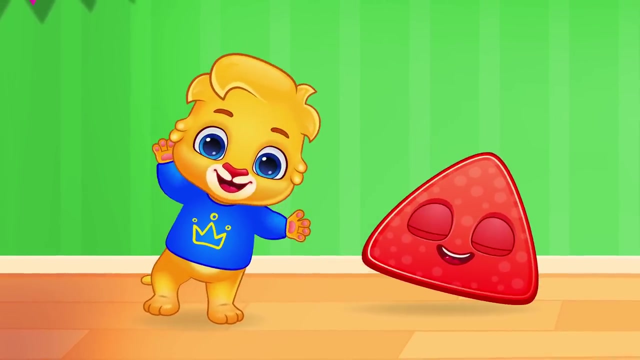 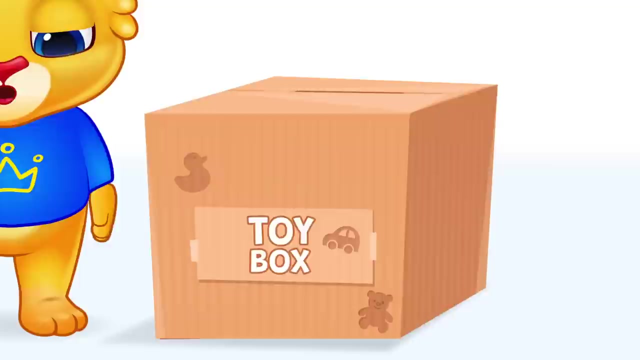 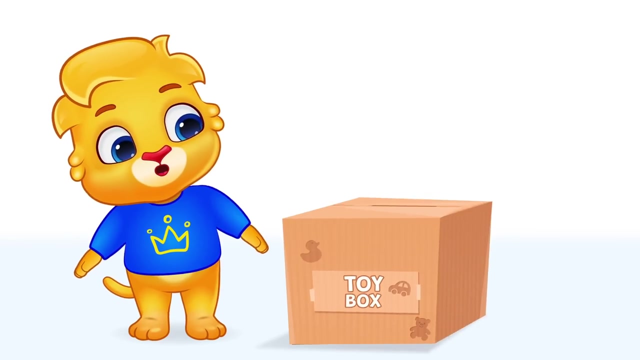 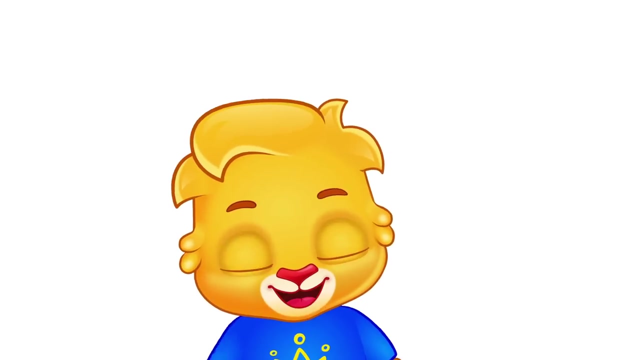 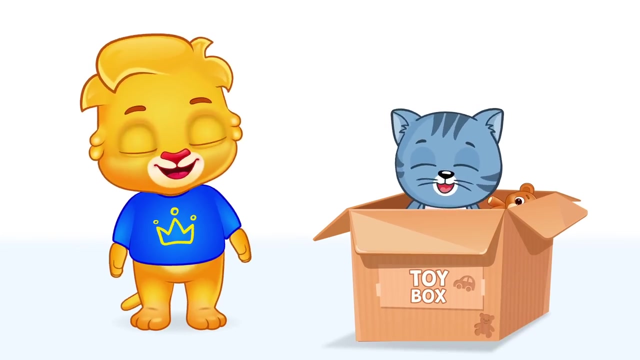 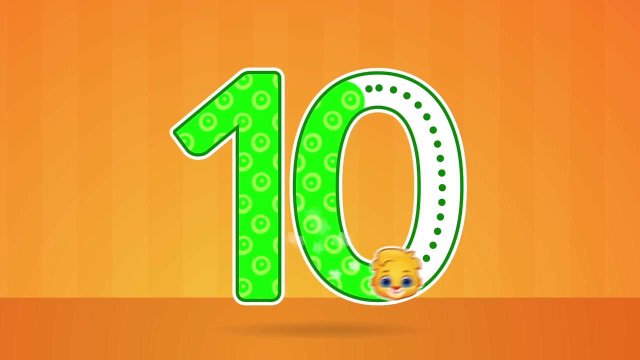 A candy is triangle, Triangle, Huh, Yay, Yeah, Woohoo, Woohoo, Woohoo, Woohoo, Wave, Wave, Meow, meow, meow Wave. Yeah, Yeah, Yeah Yeah. 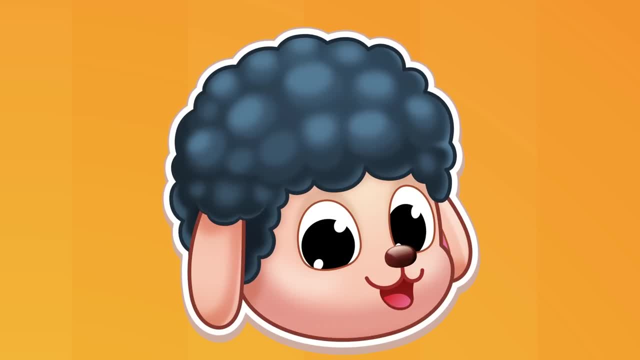 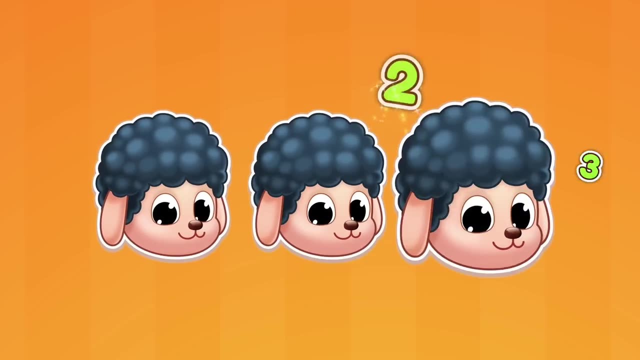 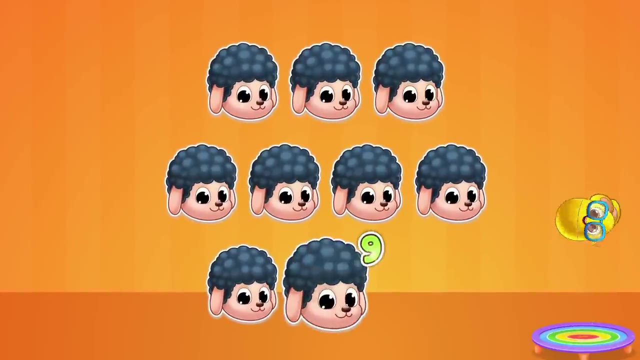 Yes, Sheeps, Oh Sheeps. One, Two, Three, Four, Roar Roar Five, Six, Seven, Eight Roar Roar Roar, Nine And ten Roar Roar Roar. 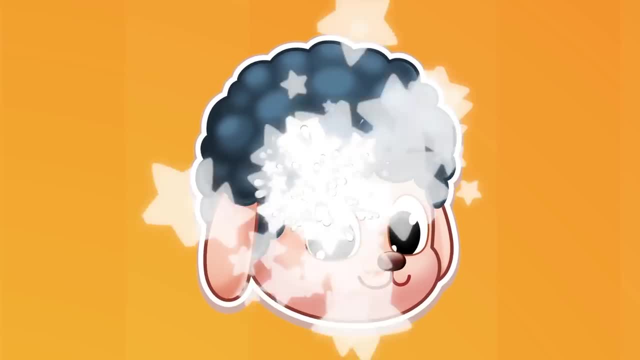 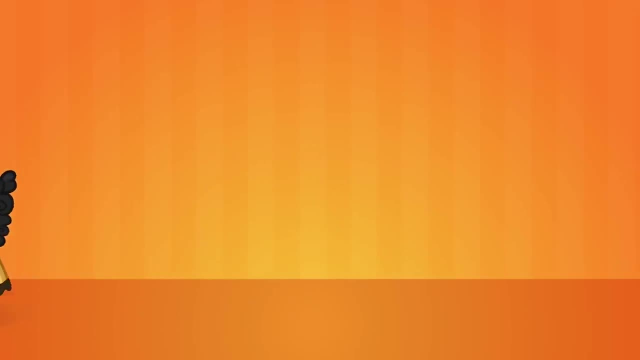 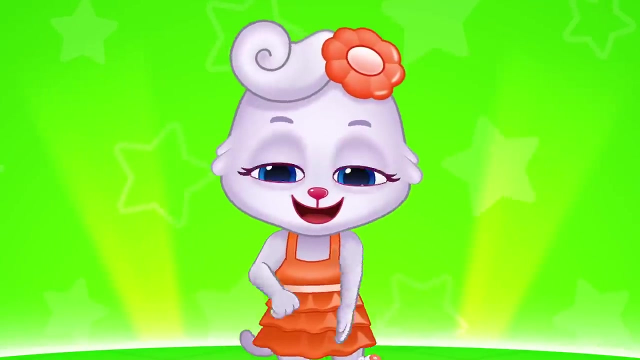 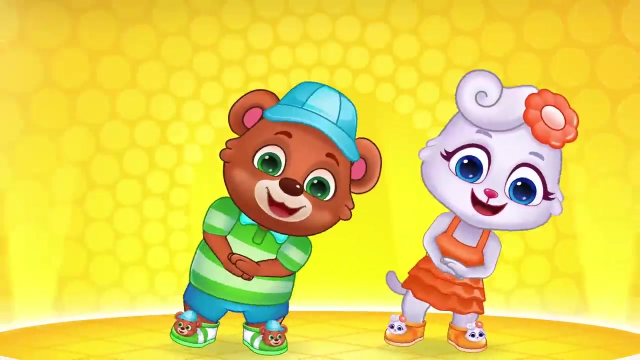 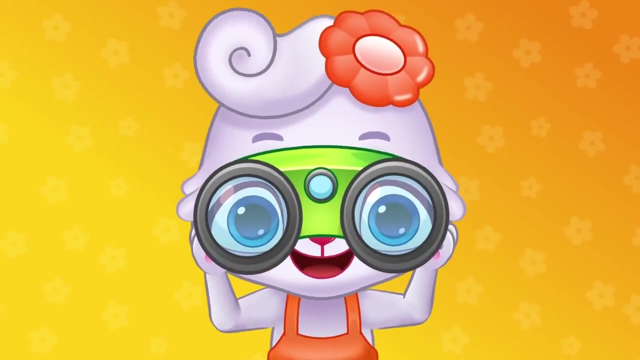 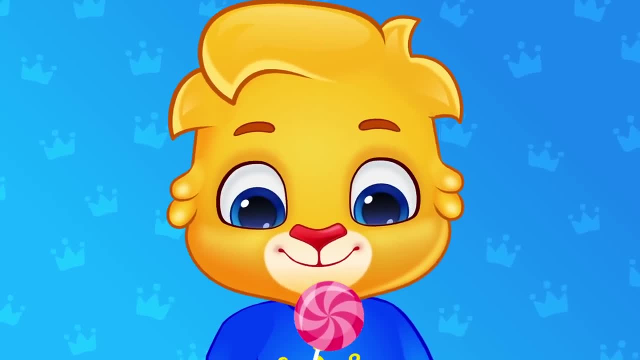 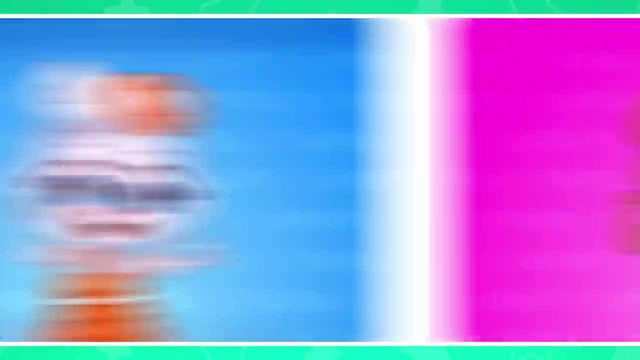 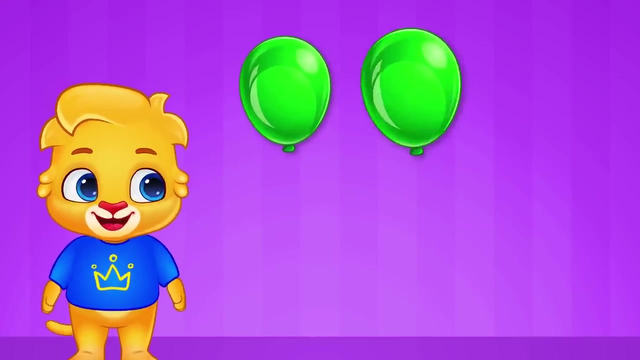 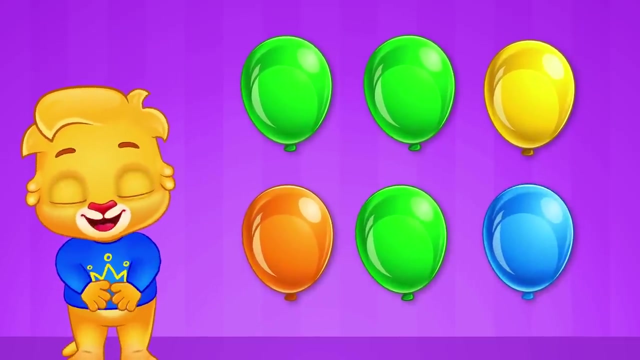 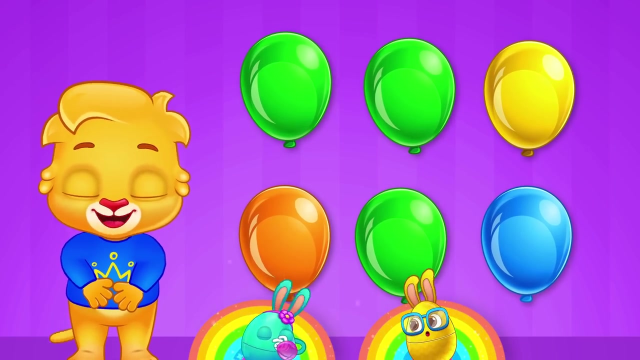 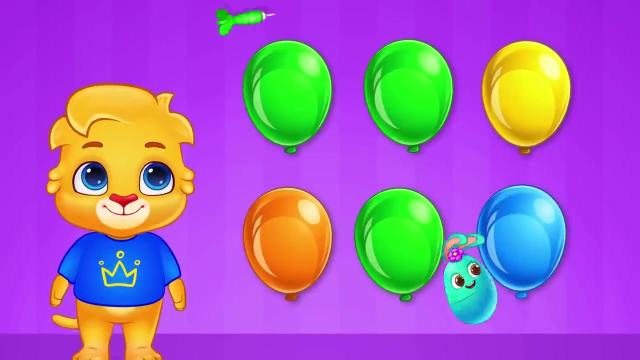 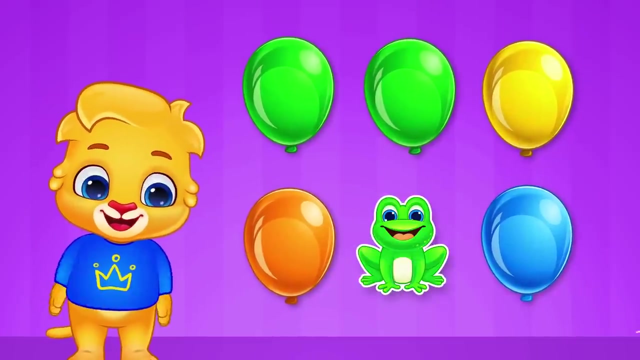 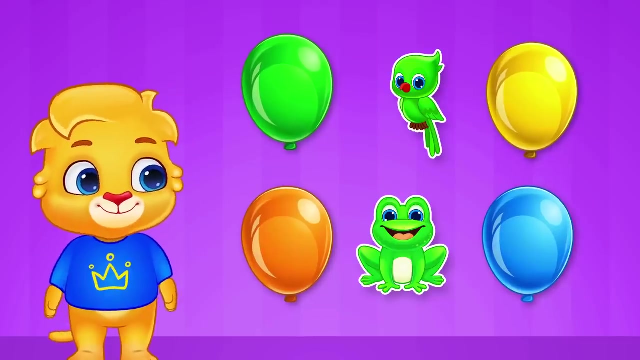 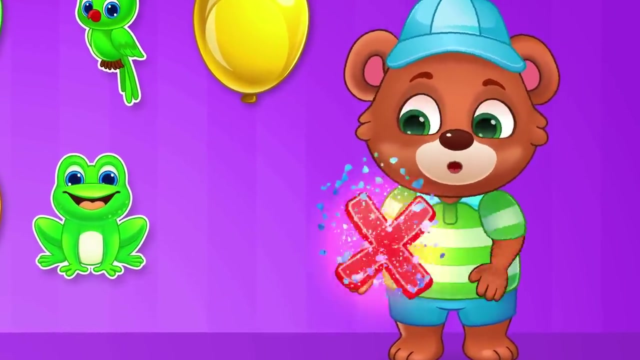 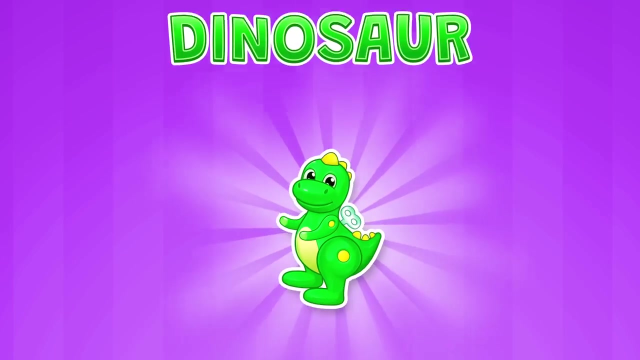 This is my mouth and I love my mouth. Look Balloons, I love balloons. Are you ready to pop balloons with the color green? Green Frog is green. Green Parrot is green. Green Dinosaur is green. Are you ready to roar like a dinosaur with me? 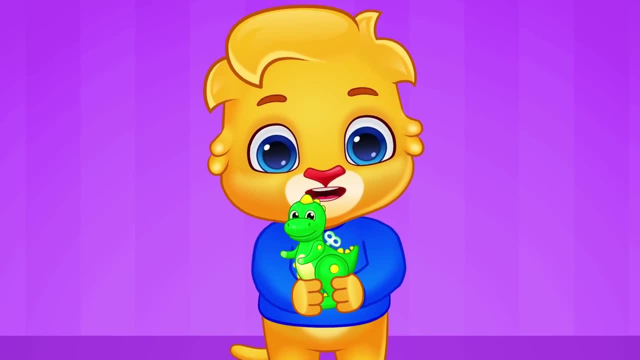 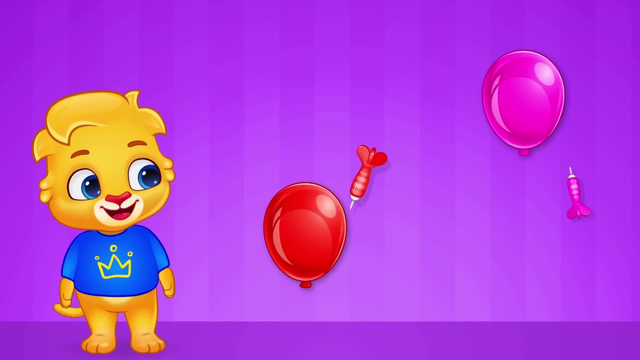 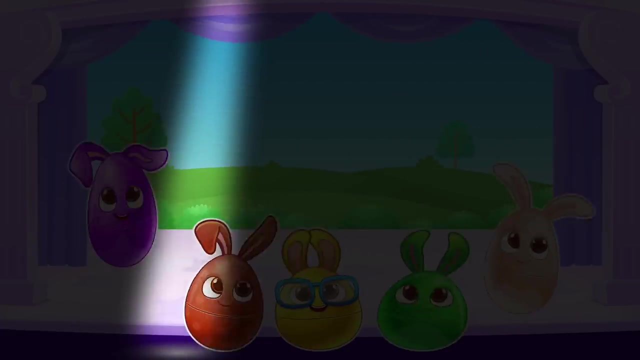 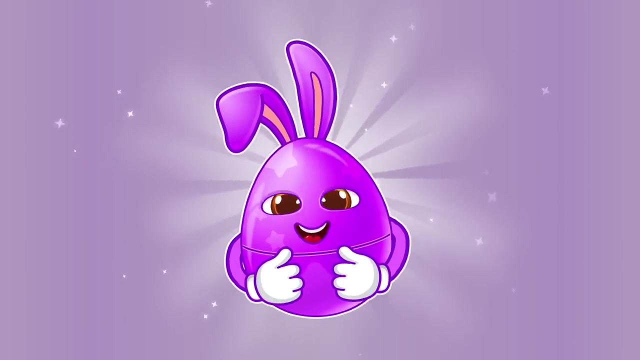 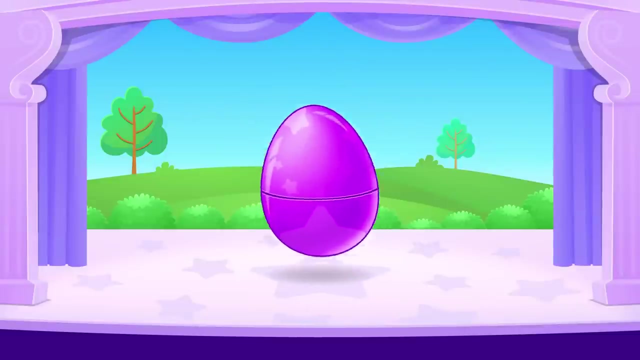 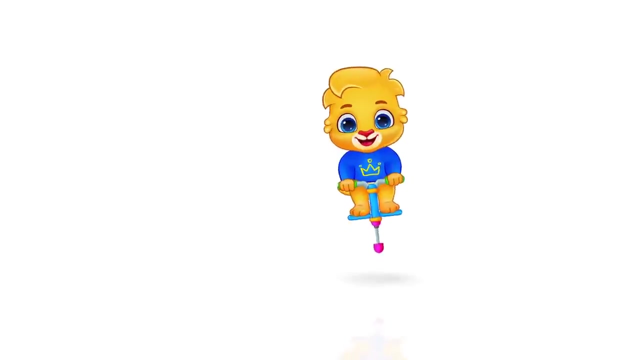 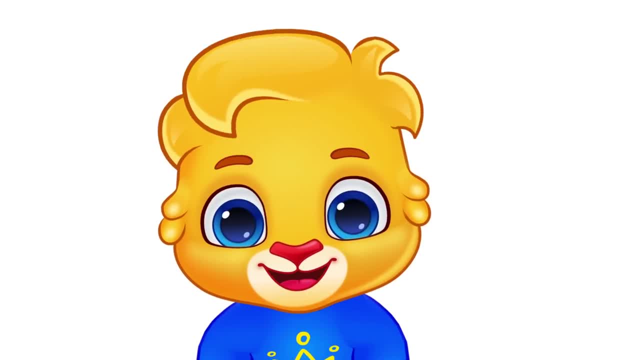 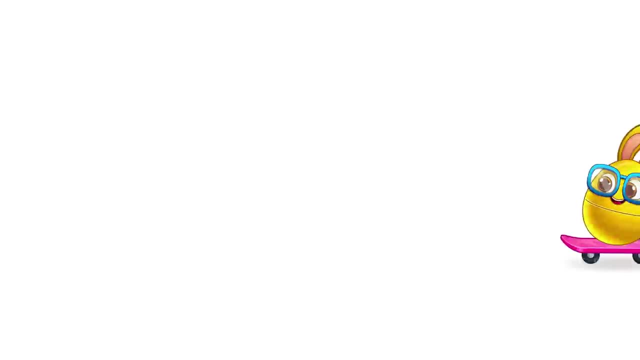 Me, Me, Me, Me, Me, Me Mew. Nice, Huh, Huh, Huh. Please Can you choose me next Meow? Jump, Yeah, Jump Meow. Are you ready Jump? 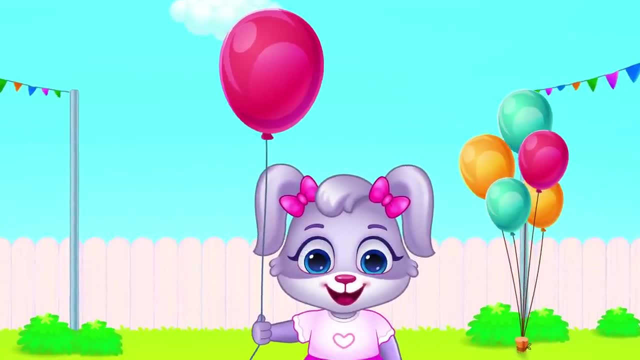 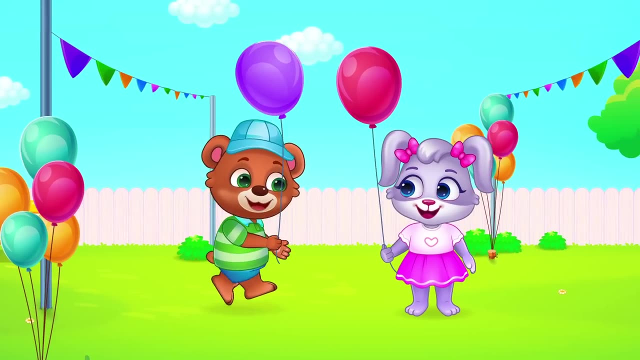 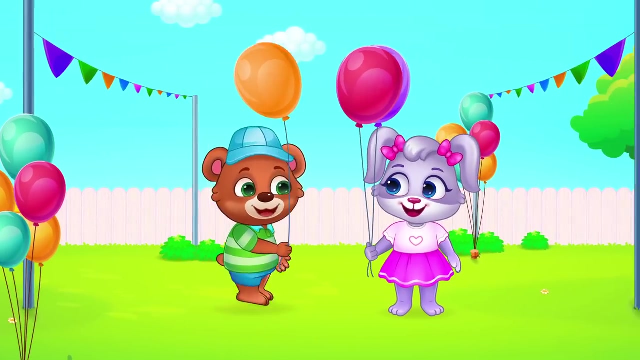 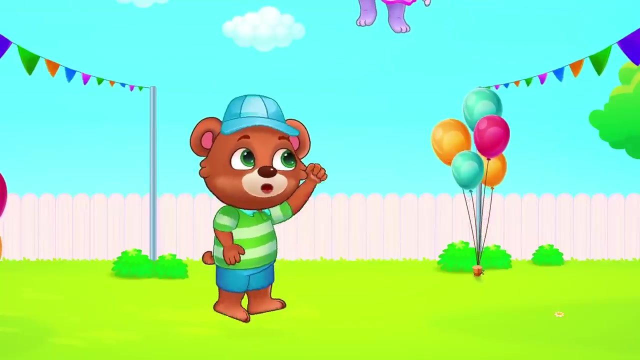 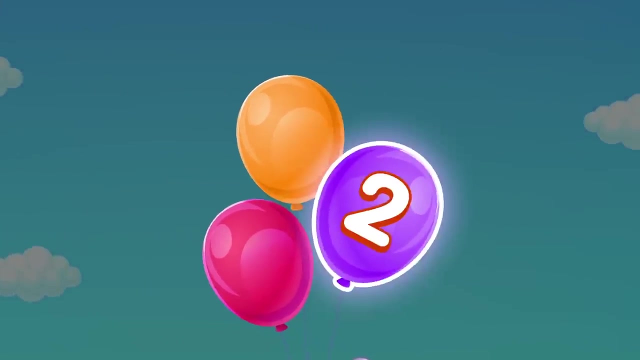 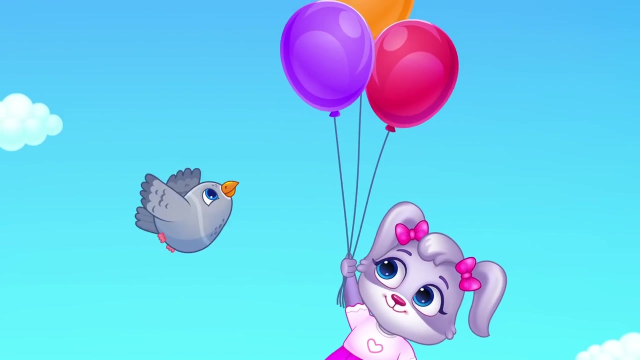 Aha, Eep, Eep, Eep, Eeyo, Aha, Woohoo, Eeyo, Aha, Whoa, Whoa. Three balloons: One, two, three, Whoa, Oh, Whoa. 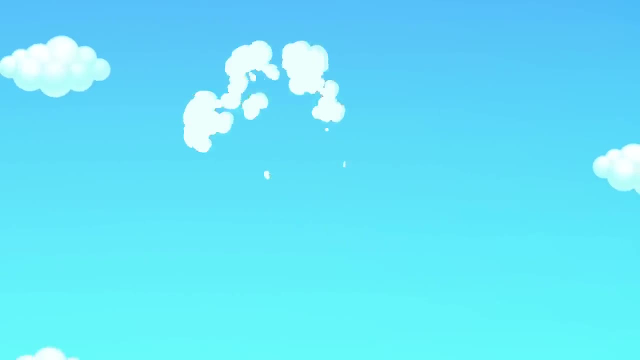 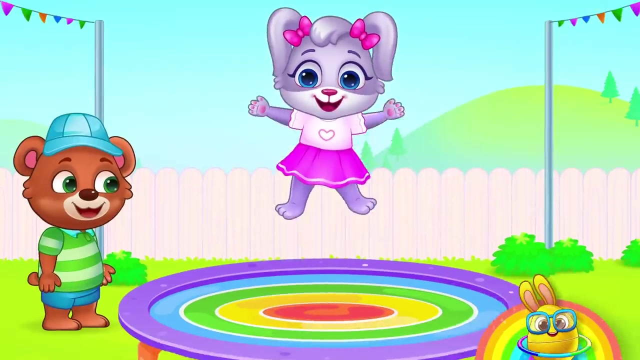 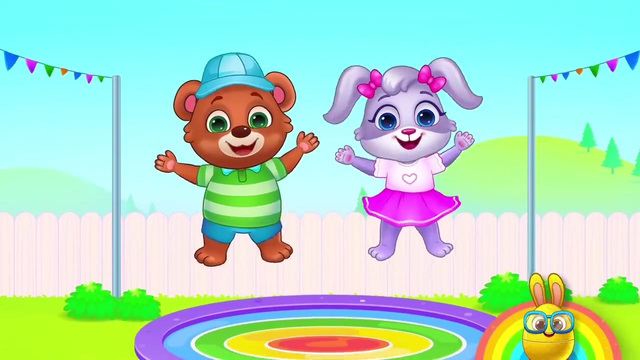 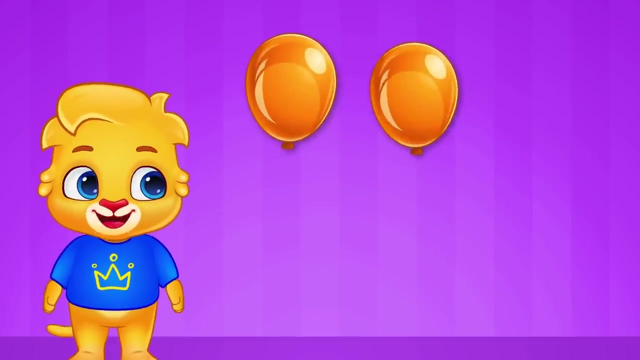 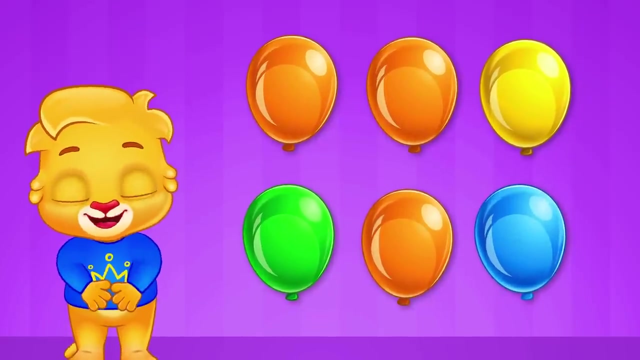 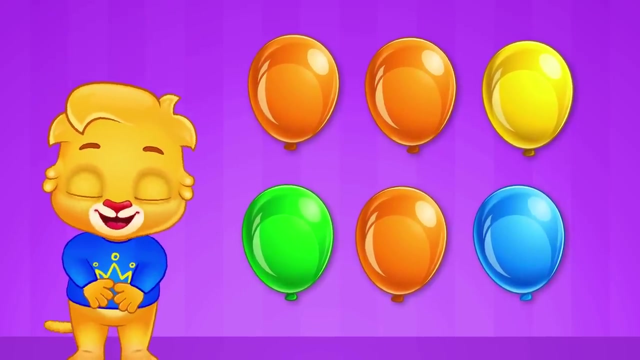 Oh, no, Oh, Oh, Whoa. Woohoo, Ruby is jumping on the trampoline. Woohoo, Yeah, Yeah, Yeah. Look Balloons. I love balloons. Are you ready to pop balloons with the color orange? 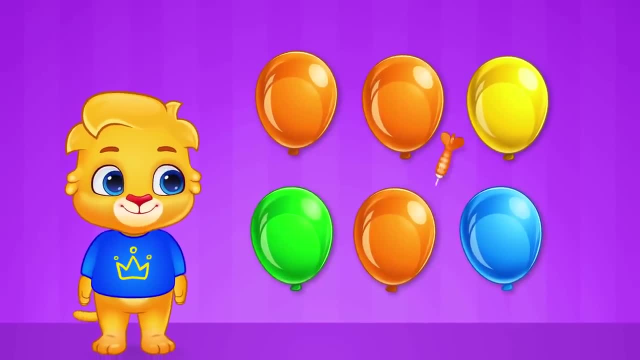 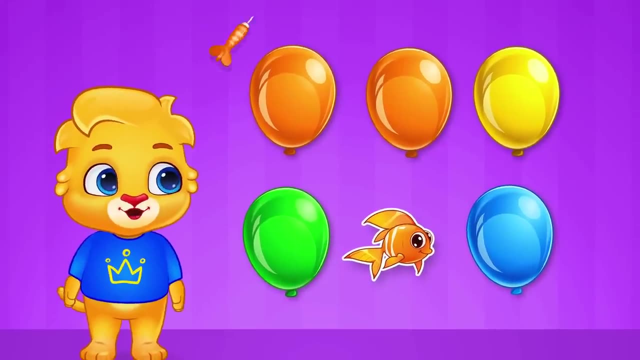 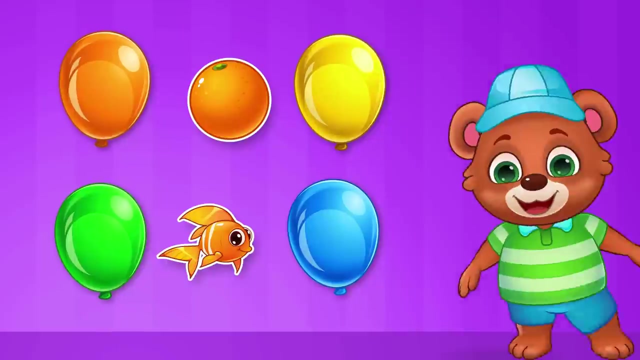 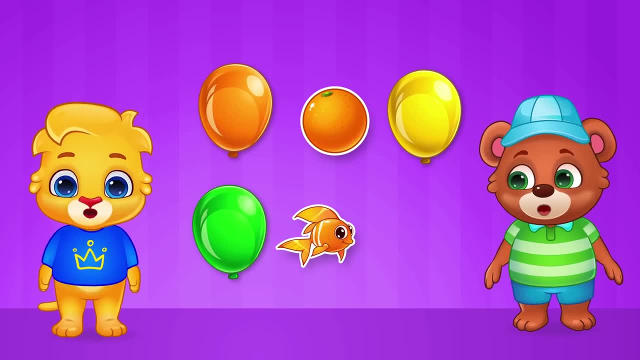 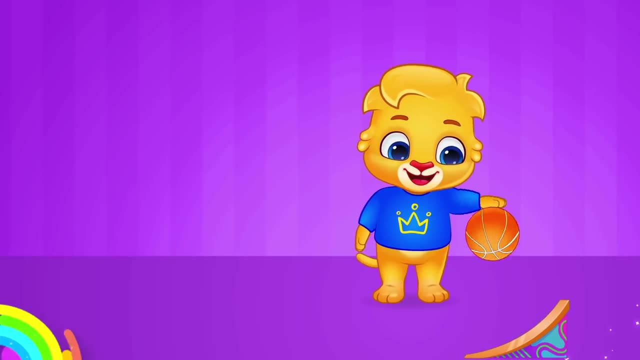 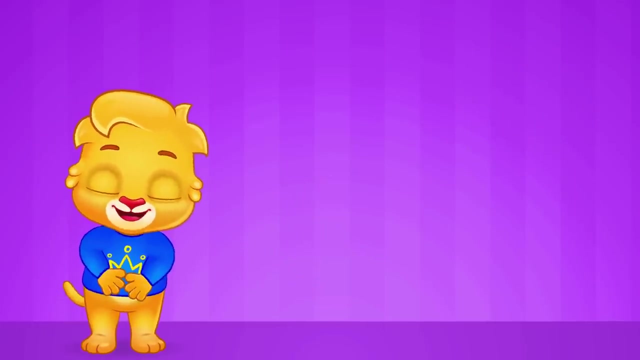 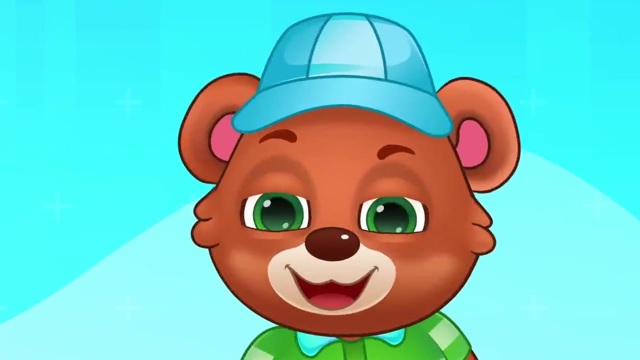 Yeah, Ah-ha, No, No, No, No, No. Orange, Yeah, Ball is orange. Yeah, Yeah, Yeah, Eeeeew. One, two, three, Whoa, Whoa, Oh, Oh, oh, ow. 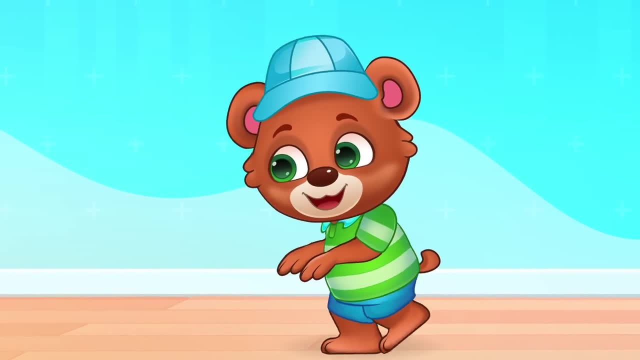 Oh, oh, oh, Wow. Awesome 是不是? Oh-ha-ha, Oh-ha-ha, Oh-ha-ha, Oh-ha-ha, Oh-ha-ha-ha, Wee-wee-wee-wee-wee-wee, Uh-huh. 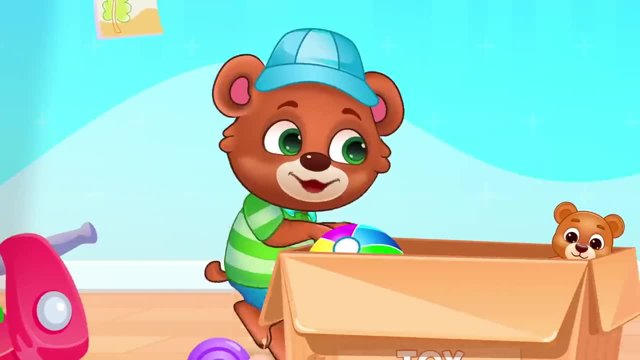 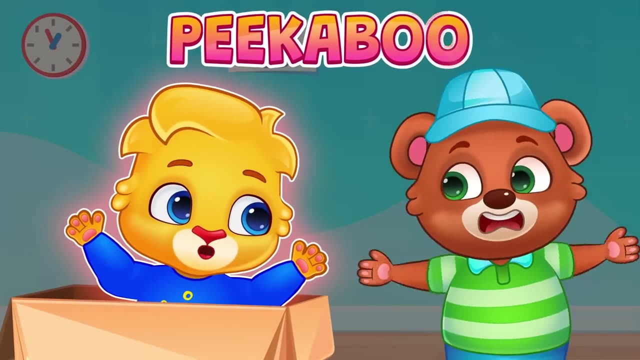 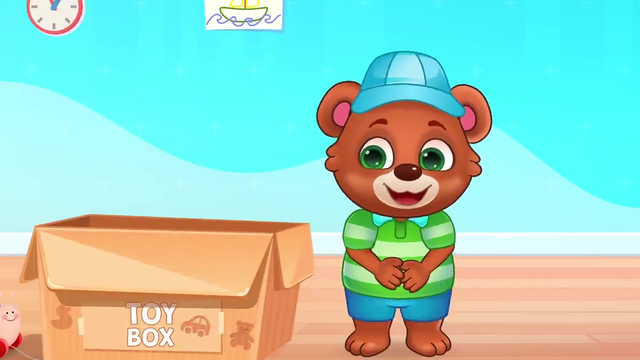 Oh-ha-ha-ha, Oh-ha-ha-ha, Oh-ha-ha-ha, Oh-oh-oh, Peek-a-boo. Lucas is playing peek-a-boo with Brody Whoa, Hmm. 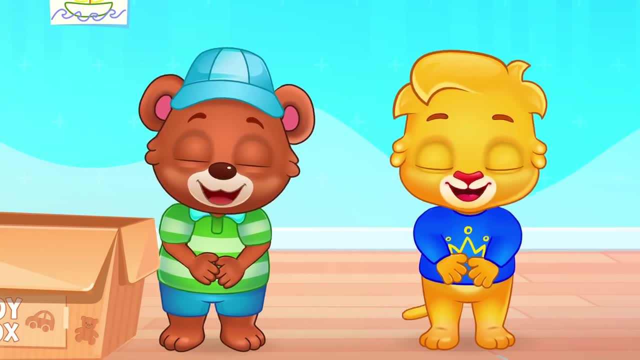 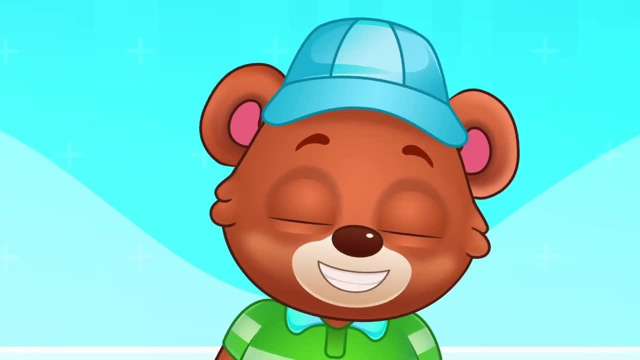 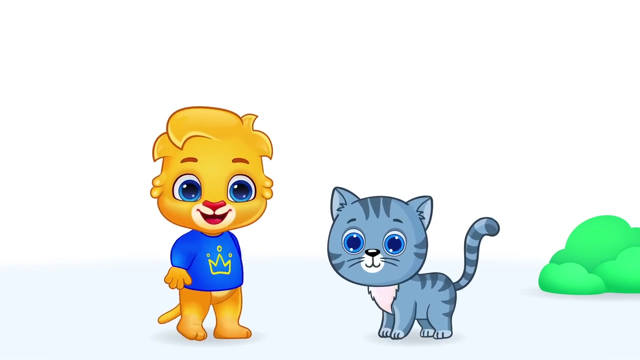 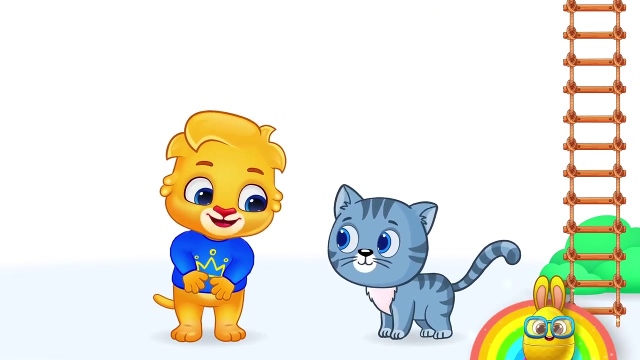 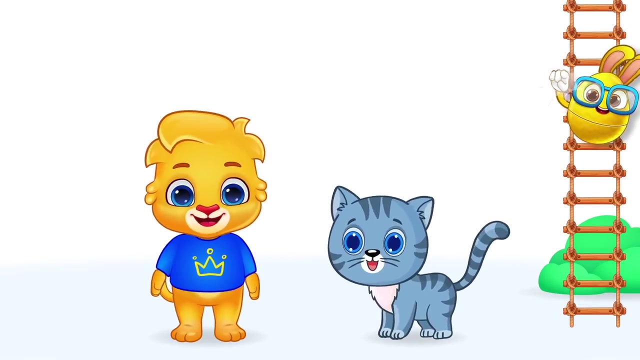 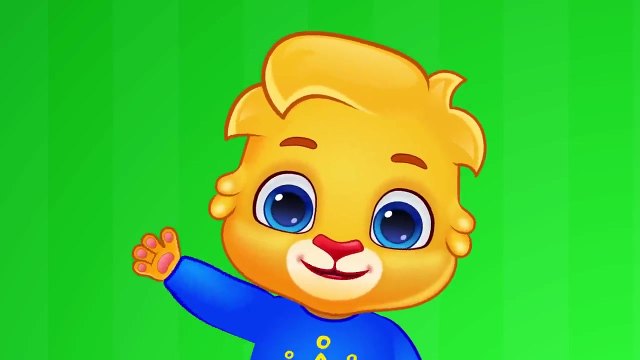 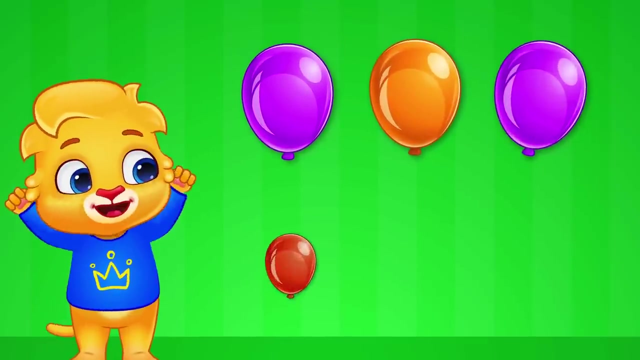 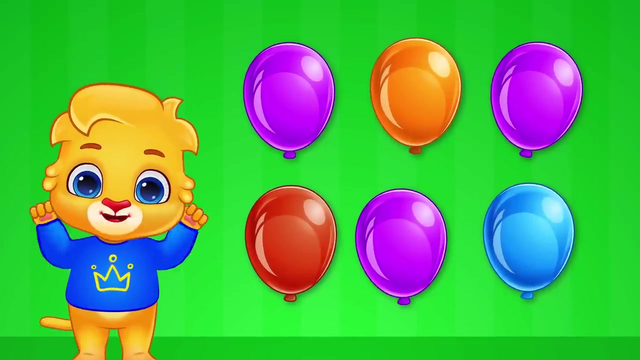 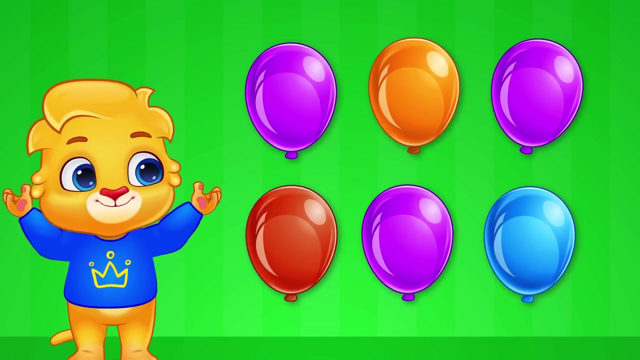 Hmm, Peek-a-boo. Yeah, Laugh Laugh, Meow, Meow Laugh. Hi friends, Look Balloons. Hey friends, Purple Balloons. Who's ready to pop them? Whoa? 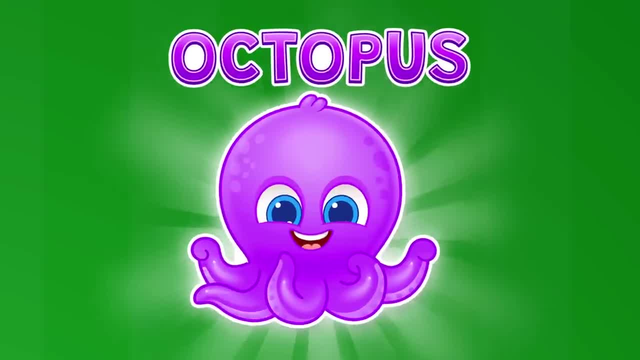 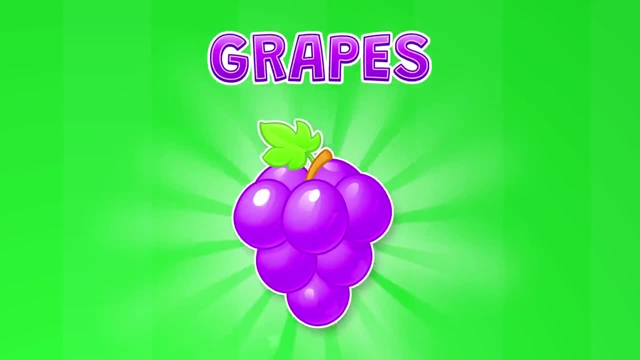 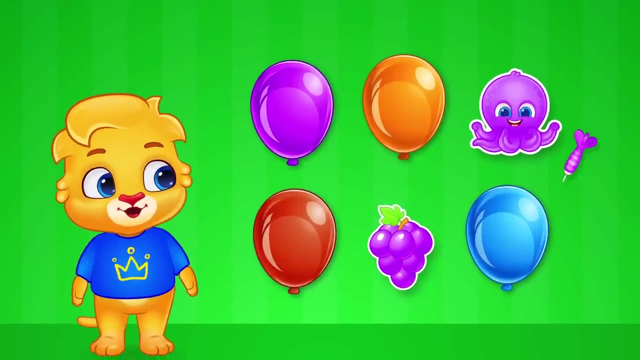 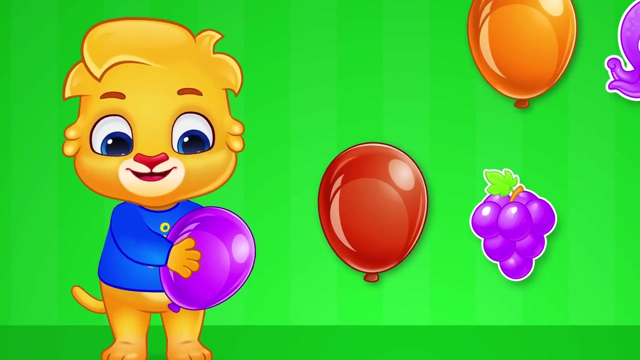 Purple Octopus is purple, Ha-ha-ha-ha. Purple Grapes are purple, Ha-ha-ha-ha. Whoa, No, no, no, no, no, no. Purple Gift box Is purple. 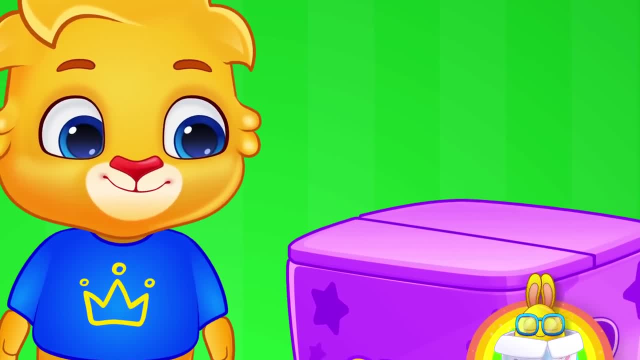 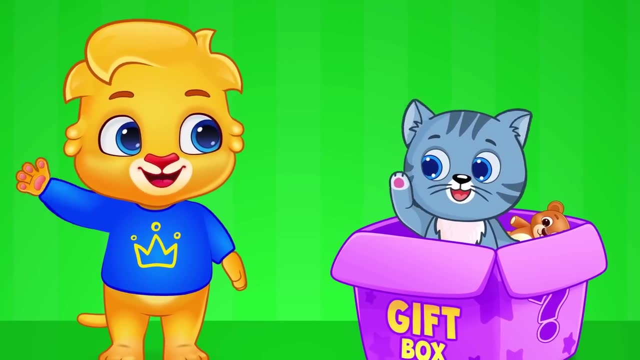 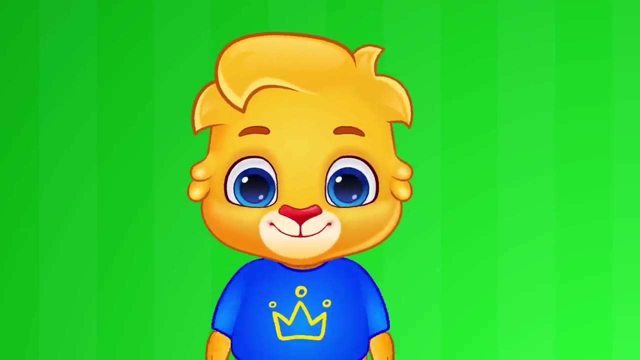 Oh, Hmm, Whoa Ha Ha-ha-ha-ha, Hey, Ha-ha-ha-ha, Ha-ha-ha-ha-ha, Ha-ha-ha-ha-ha, Ha-ha-ha-ha-ha. 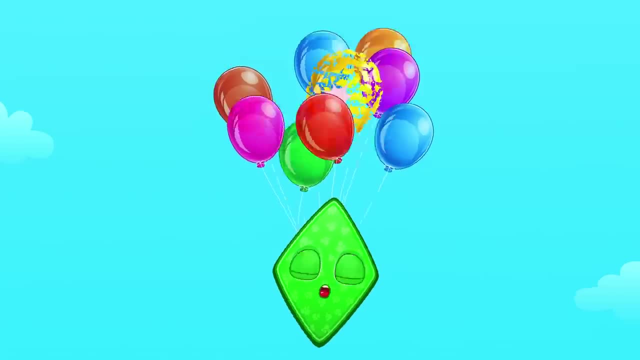 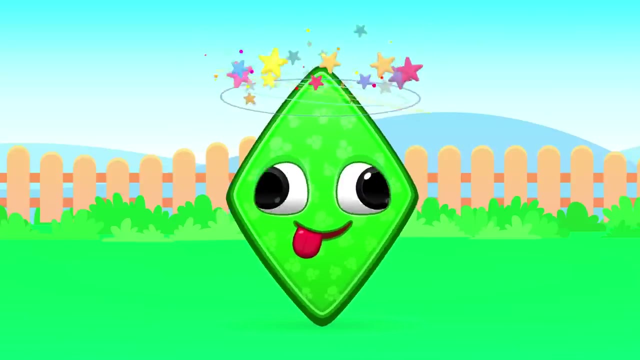 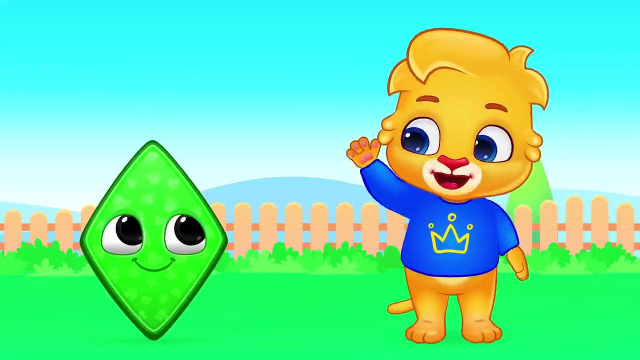 Touch it twice at once: Ha-ha-ha-ha, Huh, Ha, Ha, Ha, Ha-ha-ha-ha, Ha-ha-ha-ha, Huh, Huh, Huh, Hello, Hello. 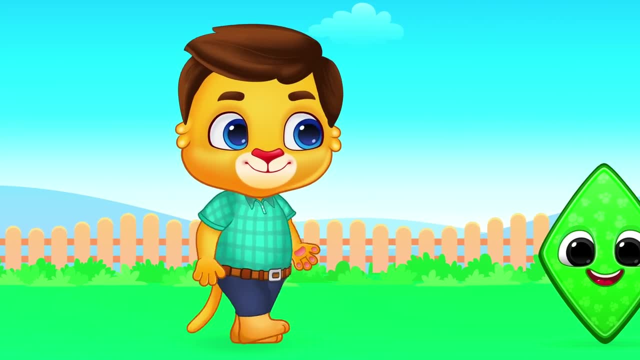 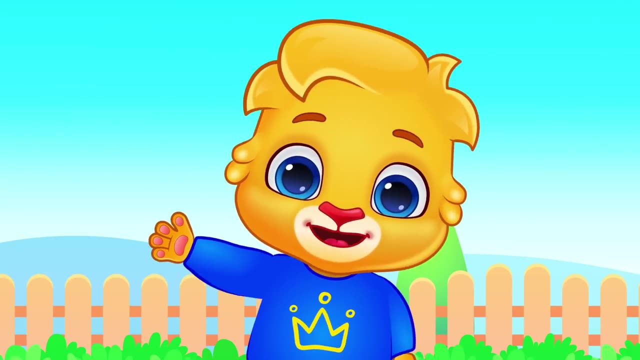 Ha-ha-ha-ha-ha, Ha-ha-ha-ha-ha, Ha-ha-ha-ha-ha, Ha-ha-ha-ha-ha, He is my dad. Can you say hi to my dad? 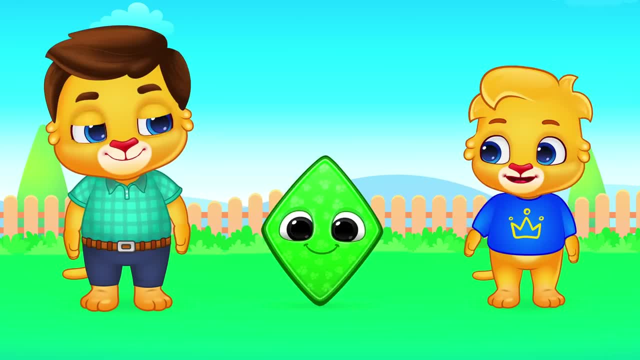 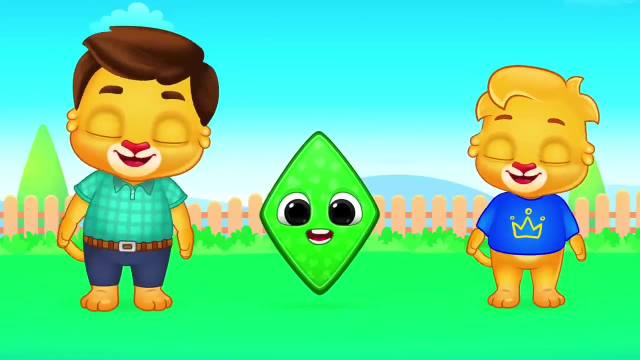 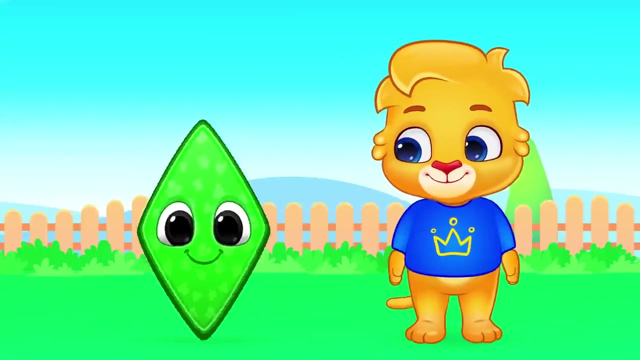 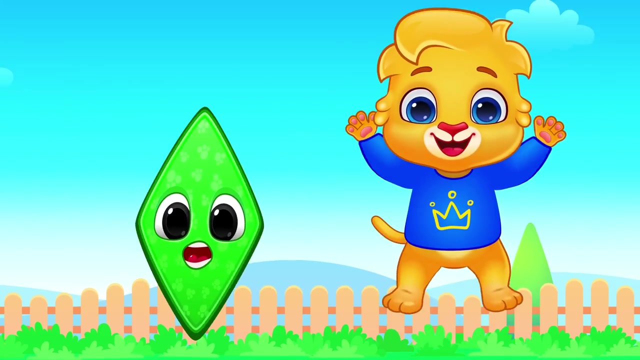 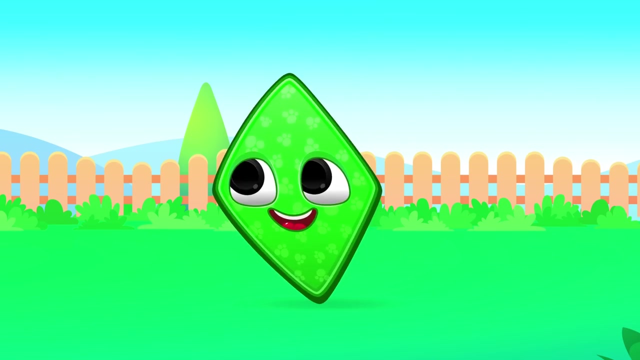 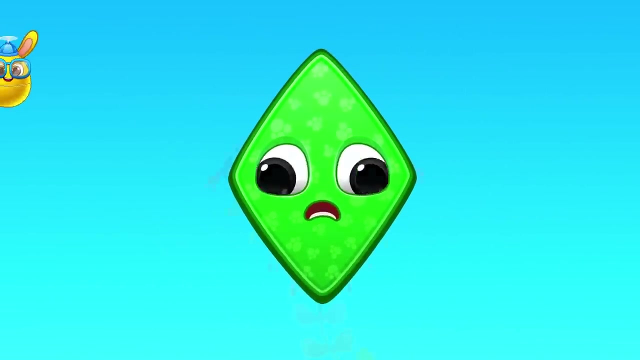 Yay, Hello Dad. Hi, I'm the Dad. Huh Huh, Huh. Do you know what shape is this? Hmm, Rhombus. Yeah, Yes, You are right, my friend, A kite is rhombus. 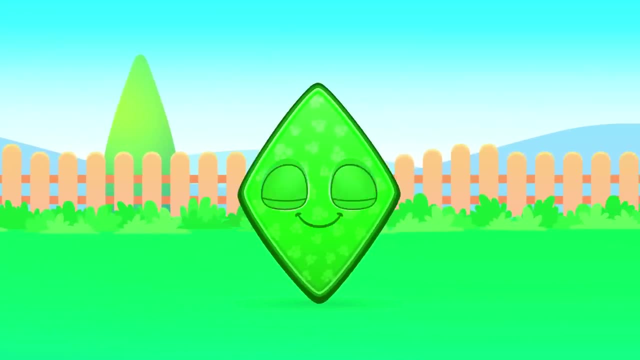 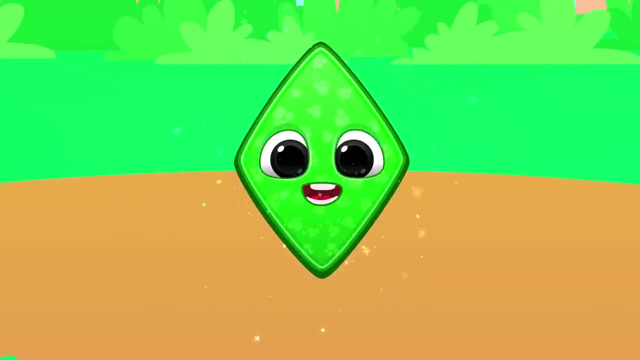 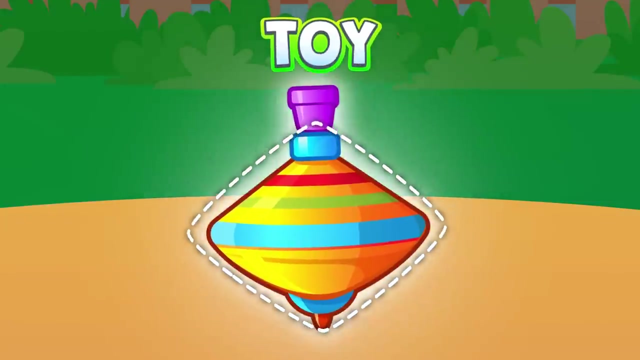 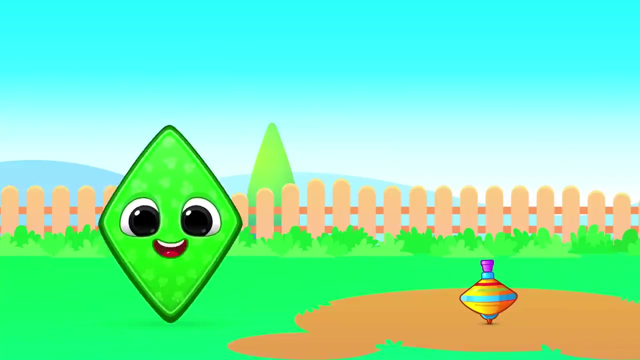 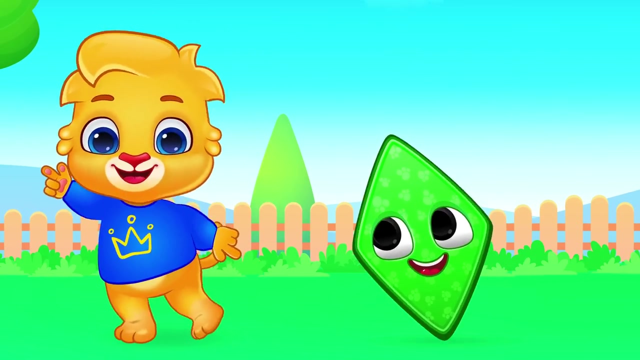 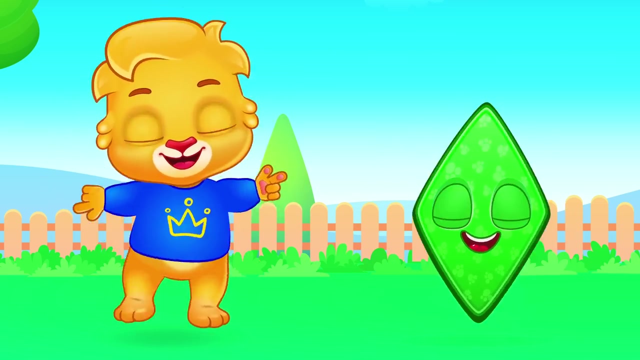 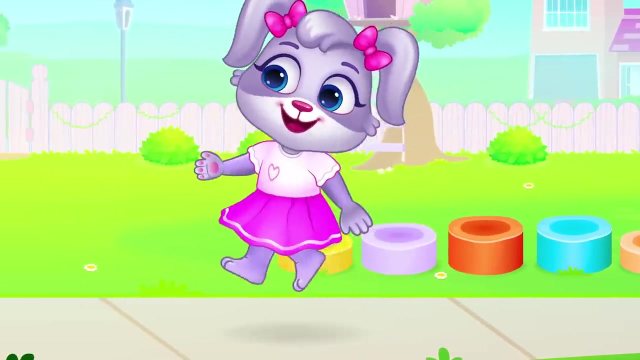 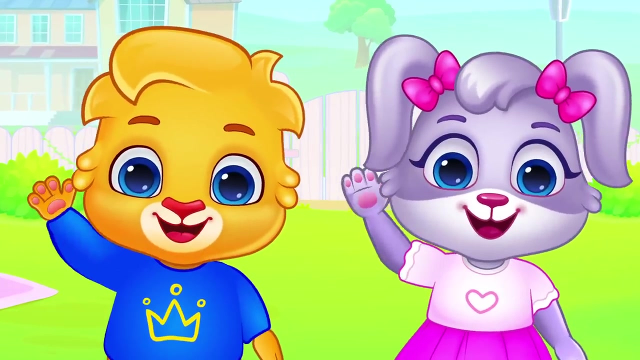 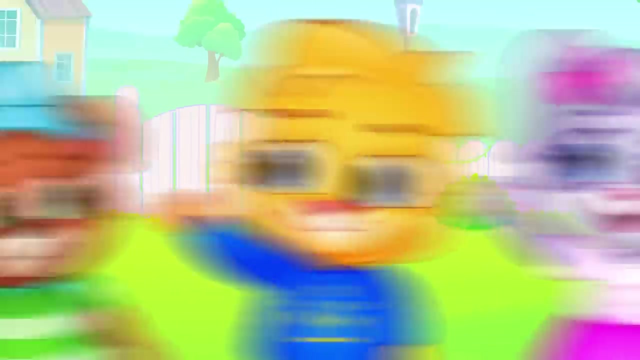 Yay, A toy is rhombus. Huh, Yay, When you meet someone, you say hello, Say hello, Say hello. When you meet someone, you say hello. That's how you greet a friend. Yeah, Hello, Hello, Hello. 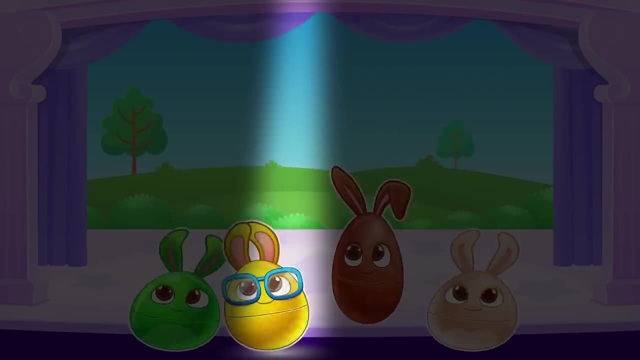 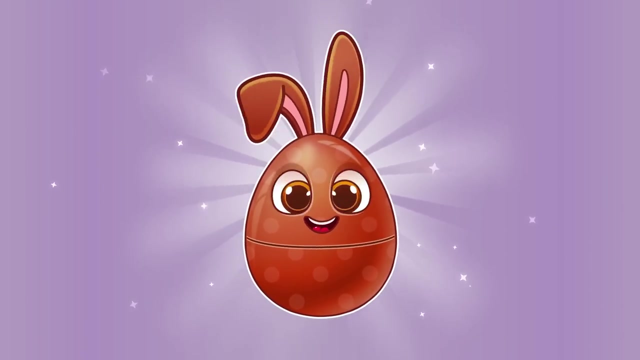 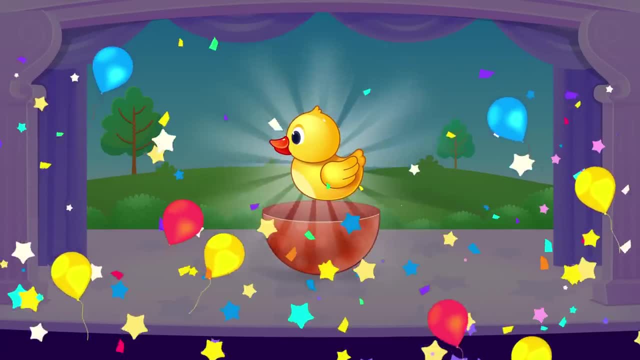 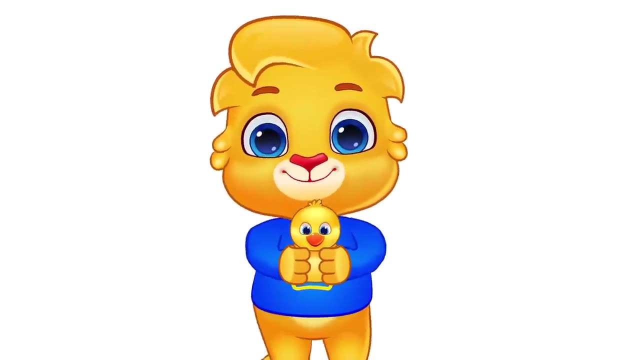 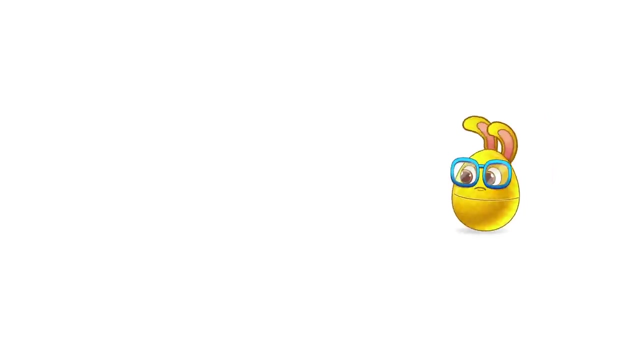 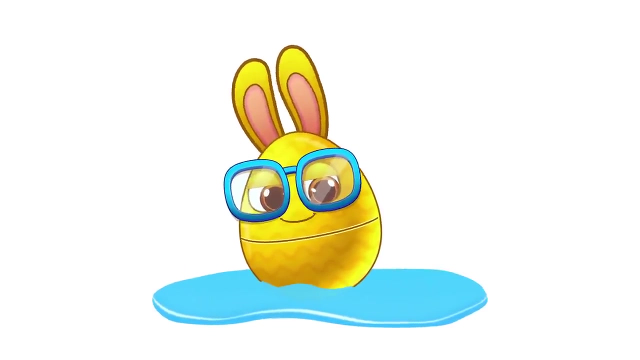 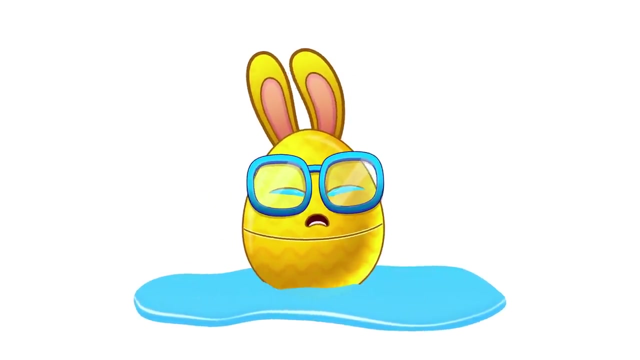 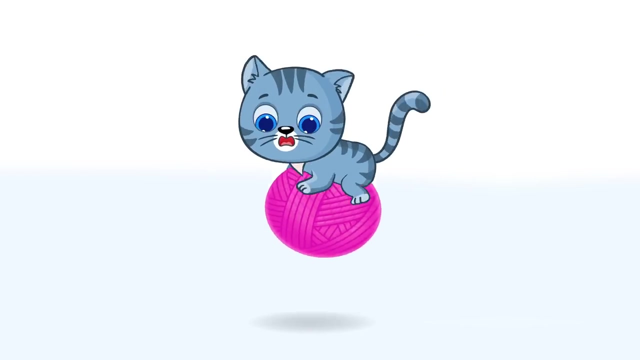 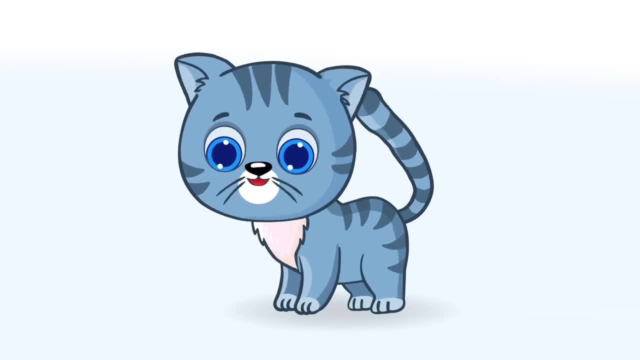 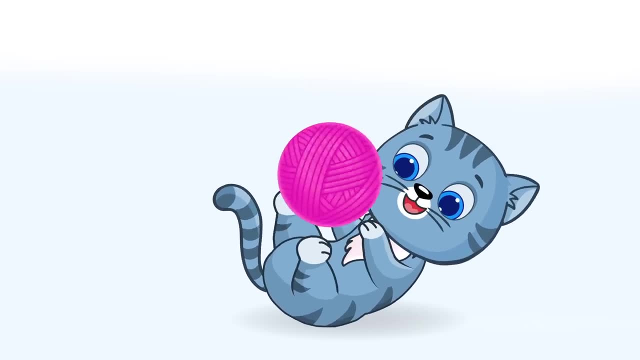 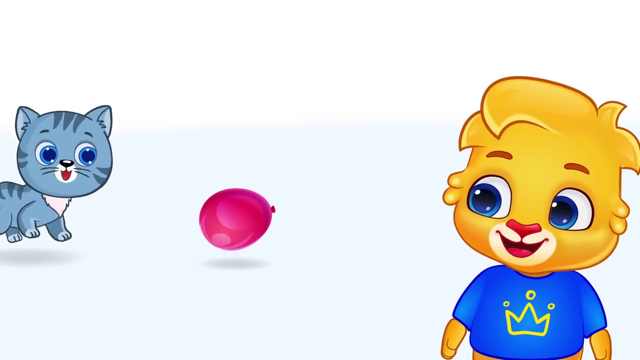 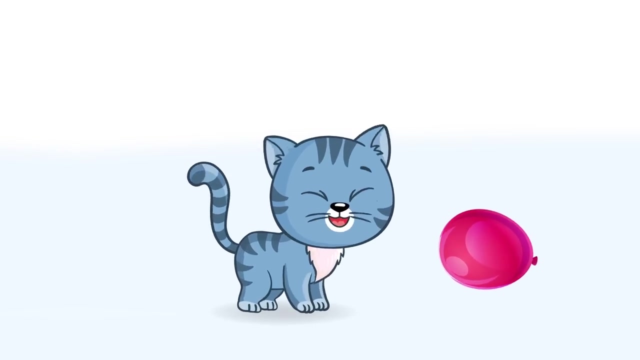 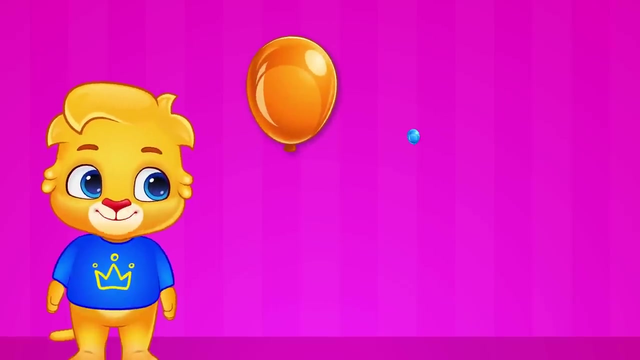 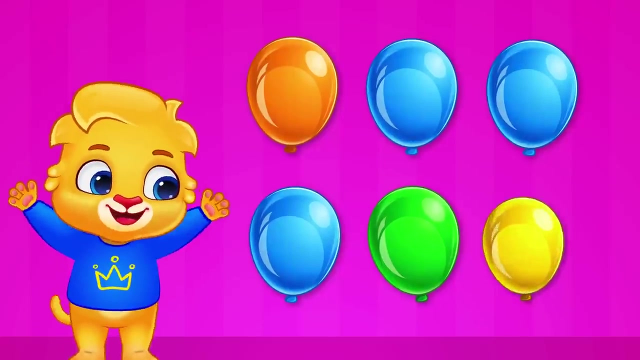 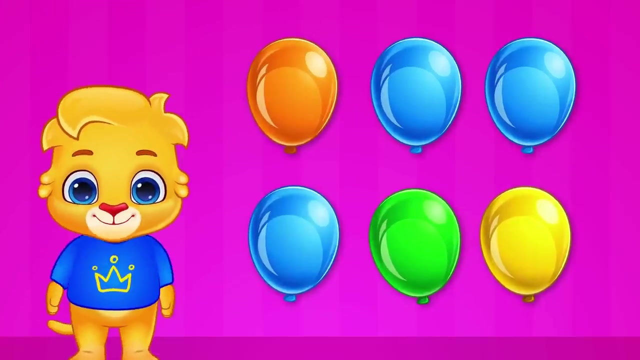 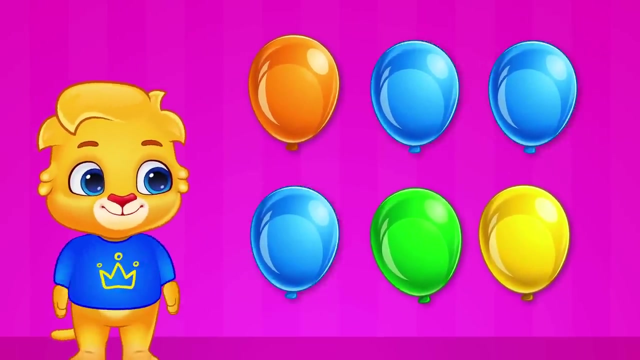 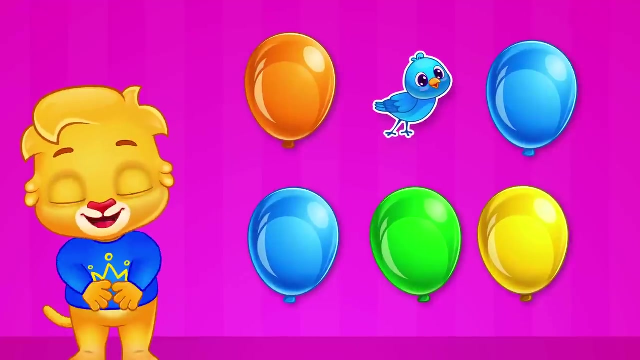 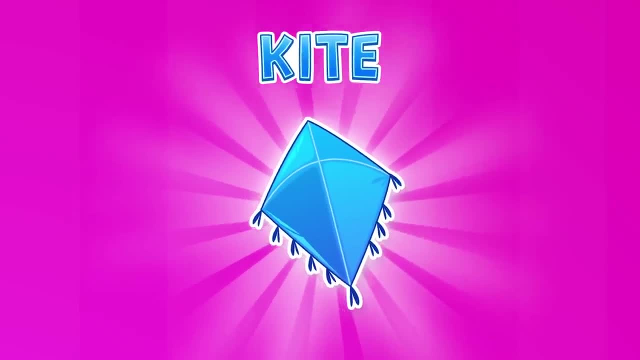 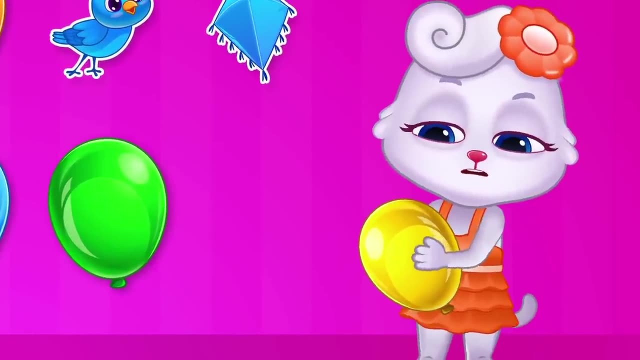 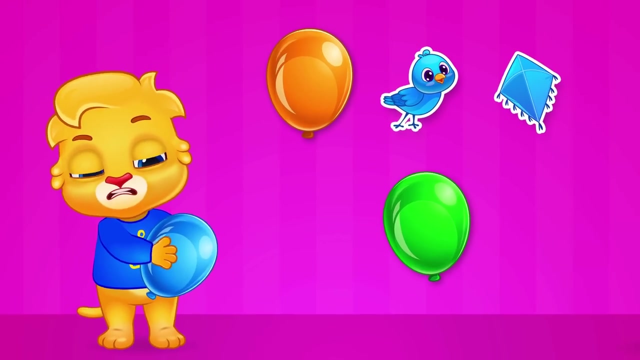 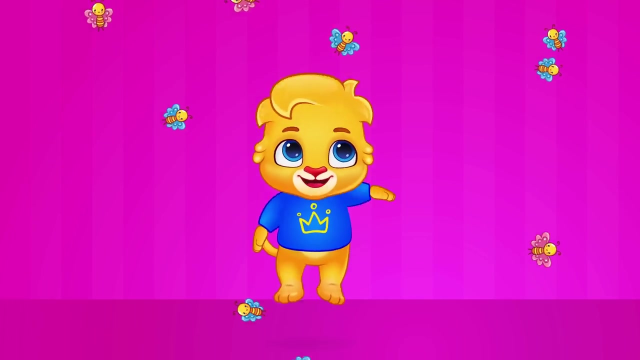 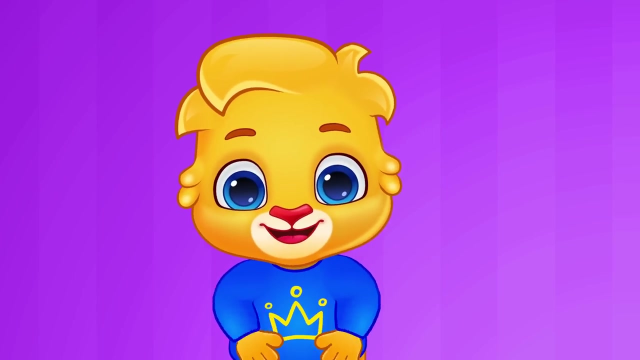 Blue Kite is blue. Oh Yeah, Yeah, No, no, no, no, Blue, Yeah, Butterfly is blue. Yeah, Woo-hoo, Woo-hoo, Woo-hoo, Ha-ha, Ha-ha-ha. 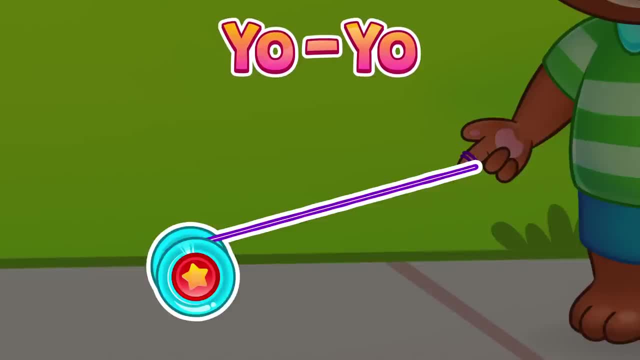 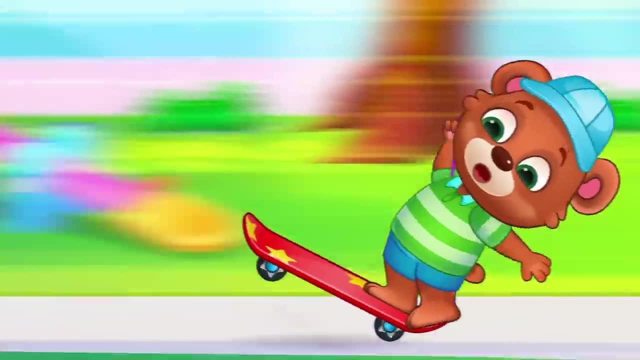 Yo-yo Y is for yo-yo Brody is walking with a yo-yo Ha-ha-ha, Ha-ha-ha, Woo-hoo, Woo-hoo, Woo-hoo, Woo-hoo, Woo-hoo. 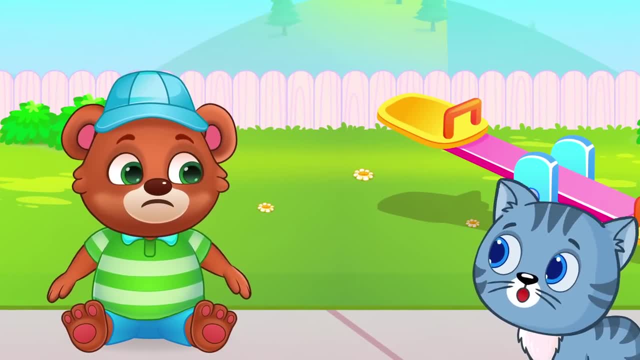 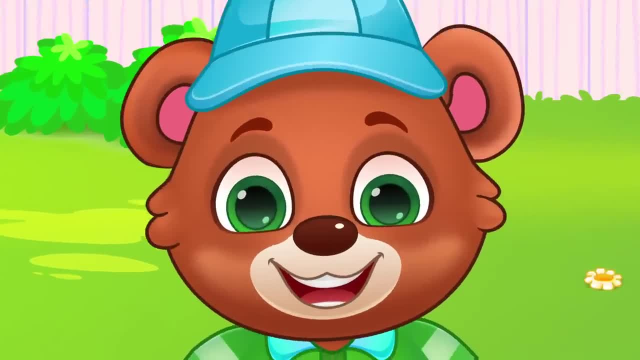 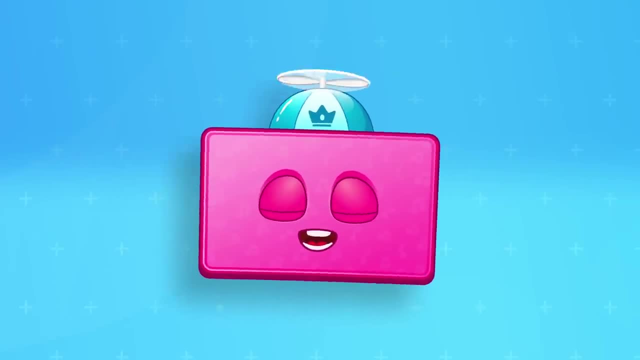 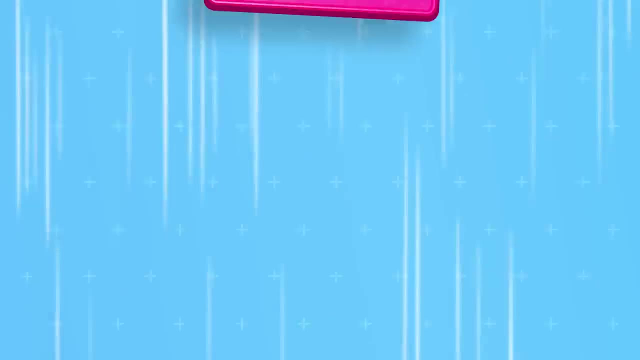 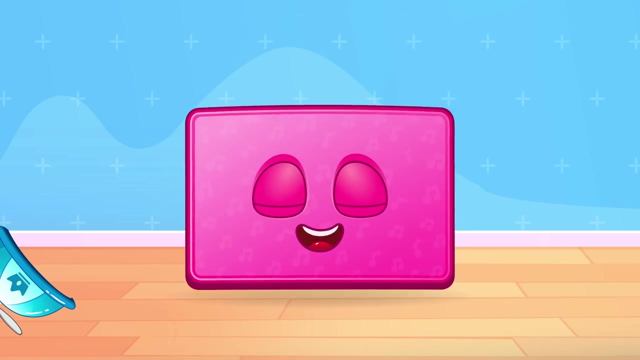 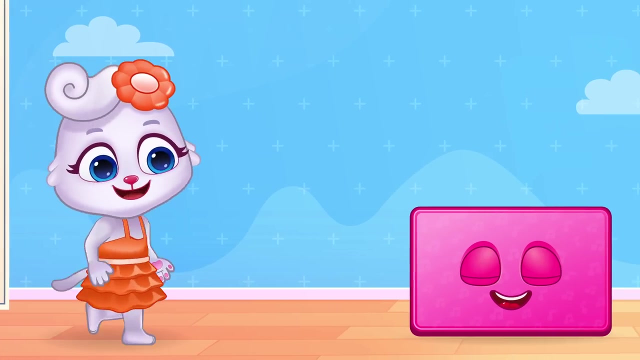 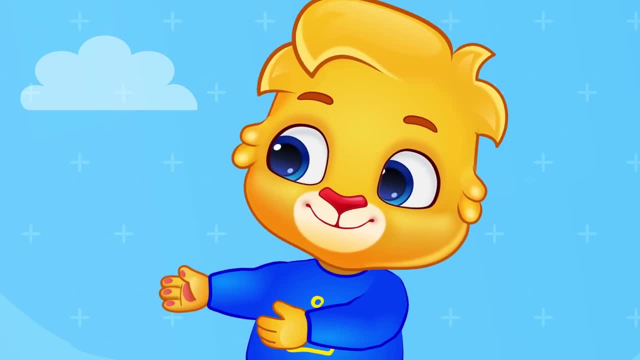 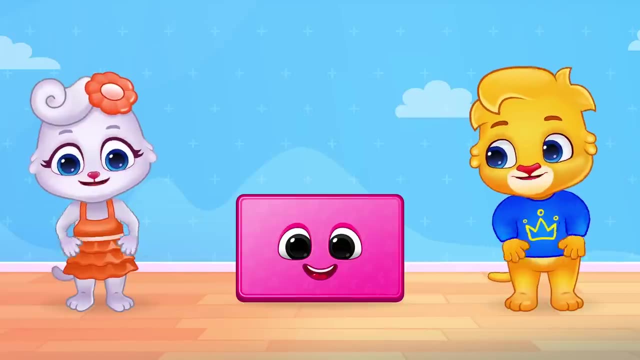 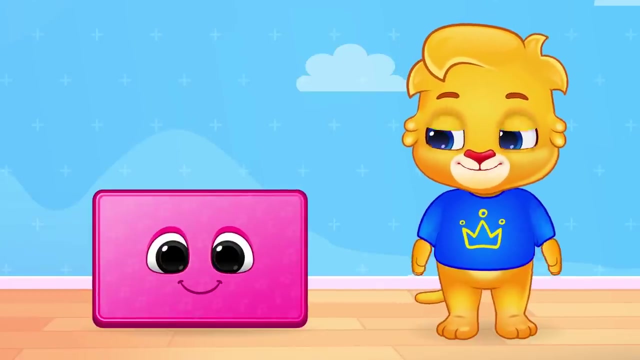 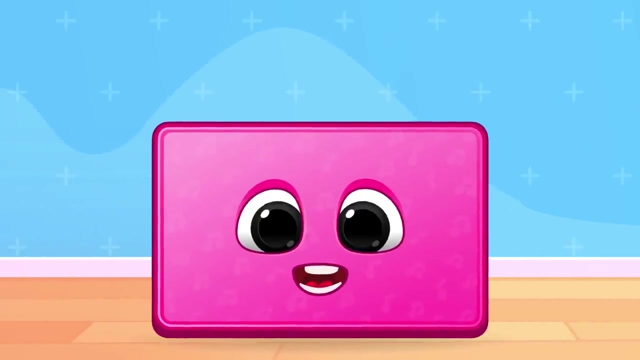 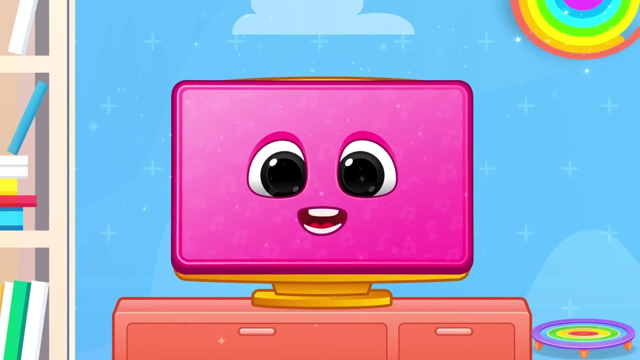 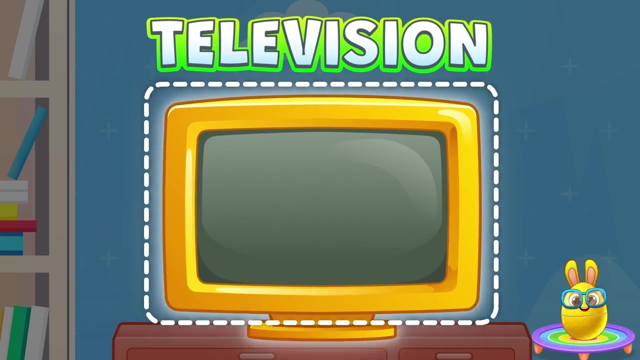 Aha, Let's say hi to my friend Lily. Hey Lily, Hello, Hi, I'm Lily. What shape is this? Will you help me please? Rectangle. Yeah, Huh, Huh. A television is rectangle. 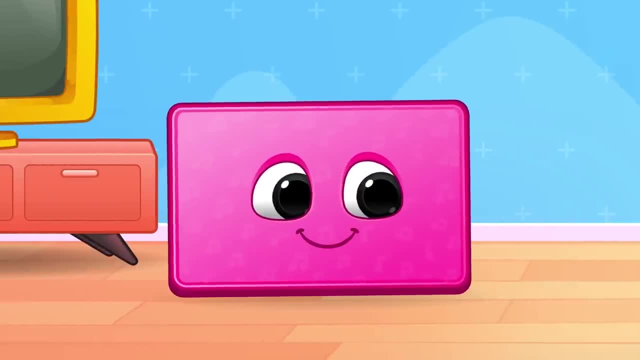 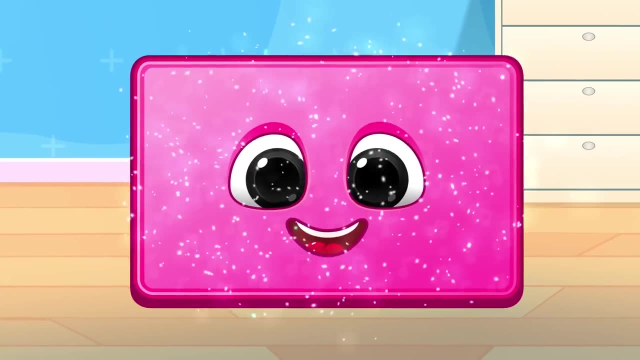 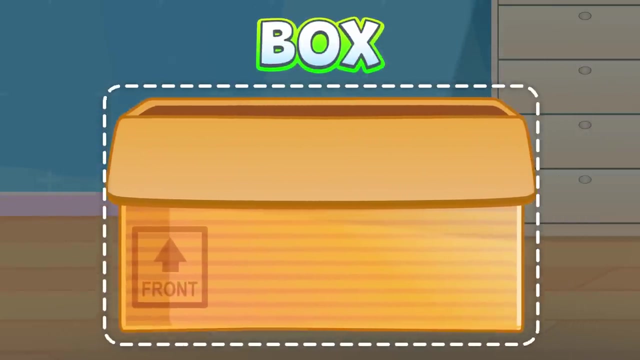 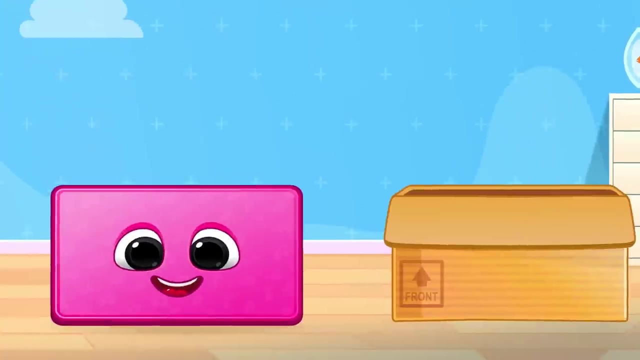 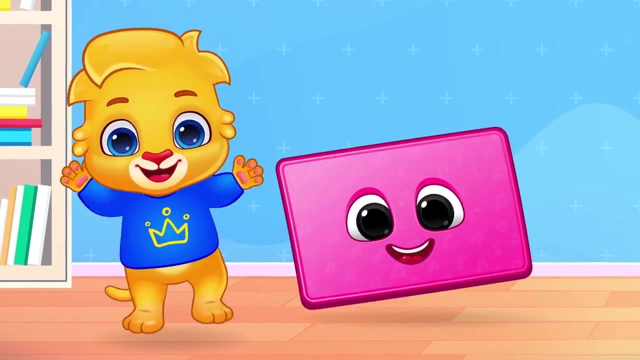 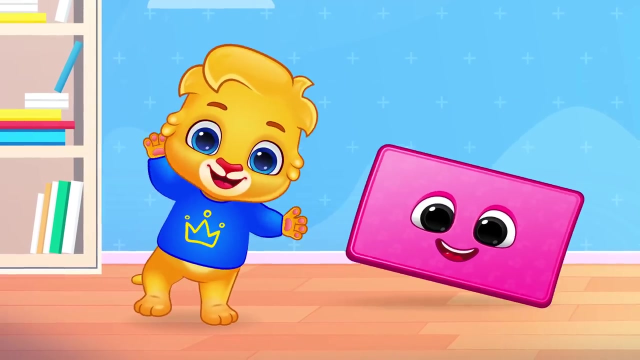 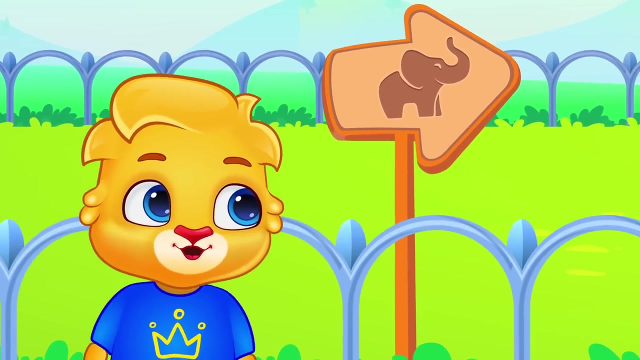 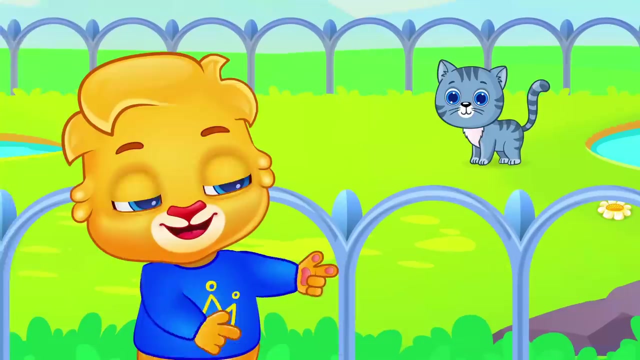 Yay, A box is rectangle. Huh, Yay, Yeah, Yeah, Woohoo, Woohoo, Hi Woo, Let's go. Uh-huh, Yeah, Oh, Meow, Meow, Whoa. 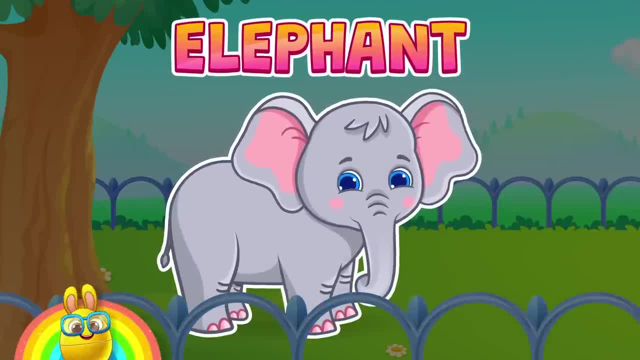 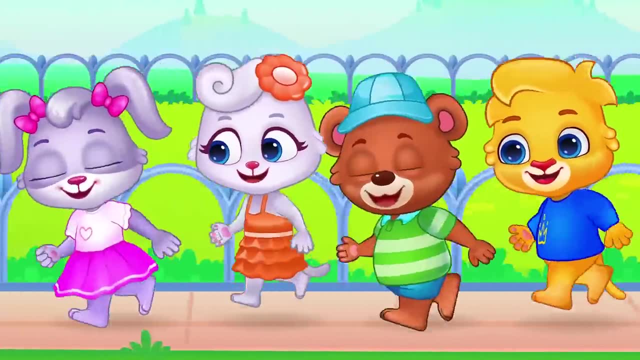 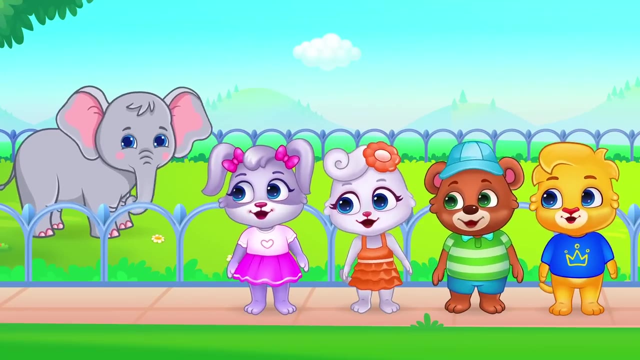 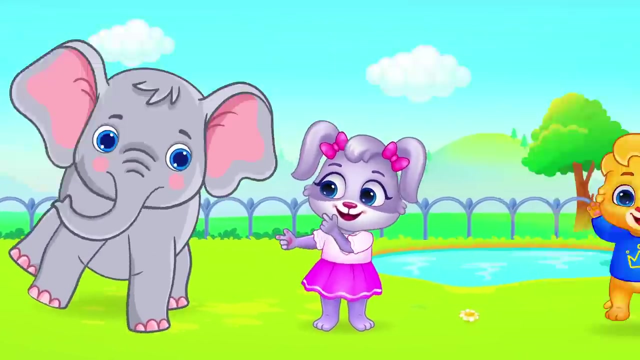 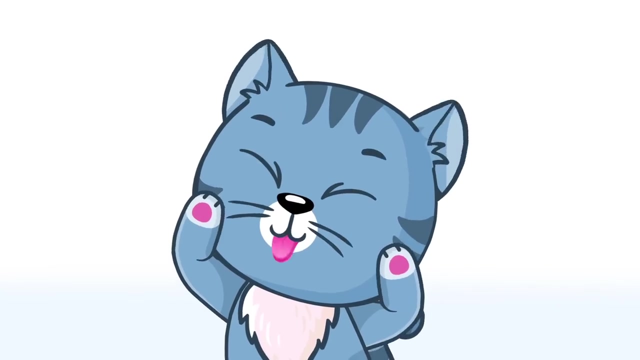 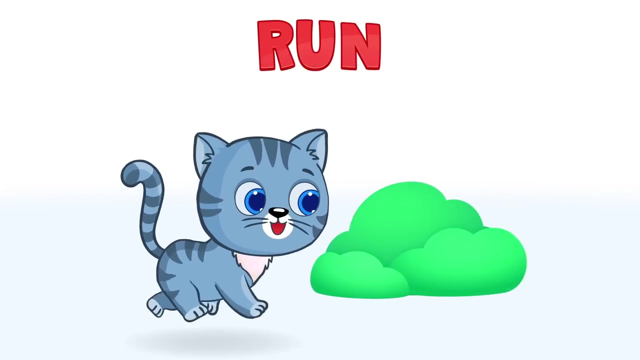 Elephant. E is for elephant. Hey, Ruby points out an elephant. Yay, Yay, Yay, Yay, Meow Meow, Oh, Meow, meow meow, Woo Run, Run Yeah. 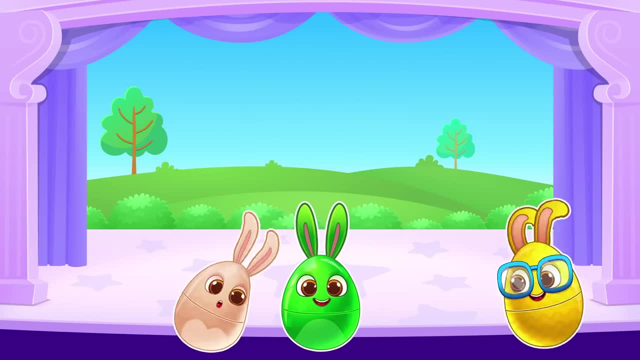 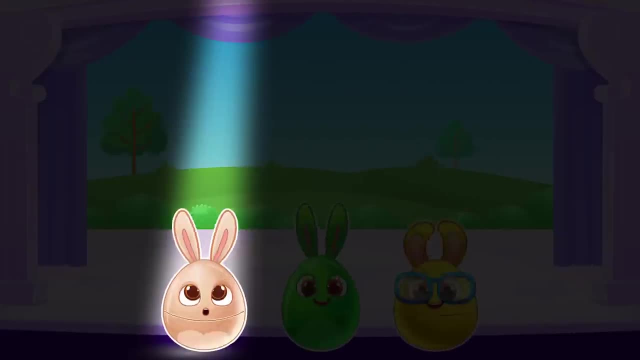 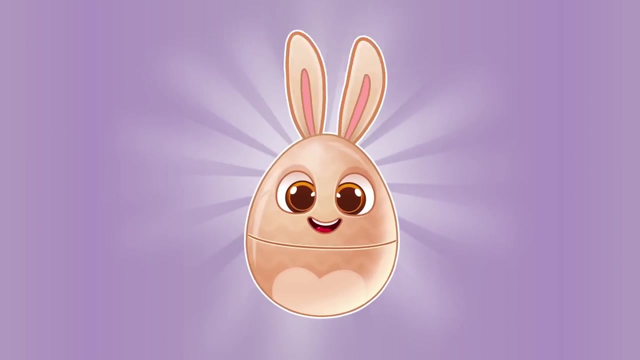 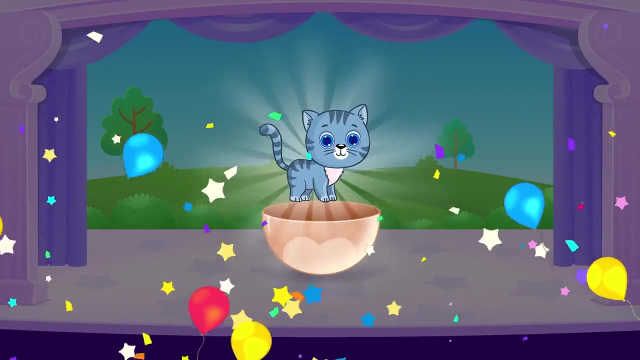 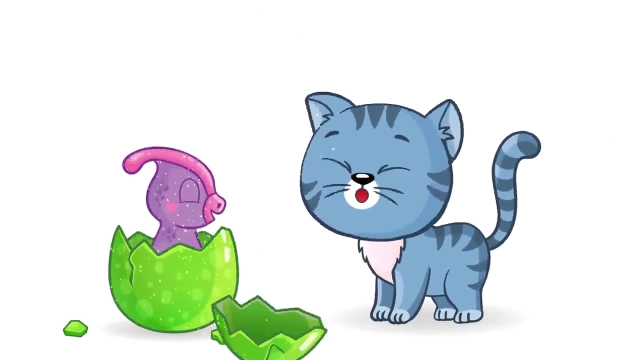 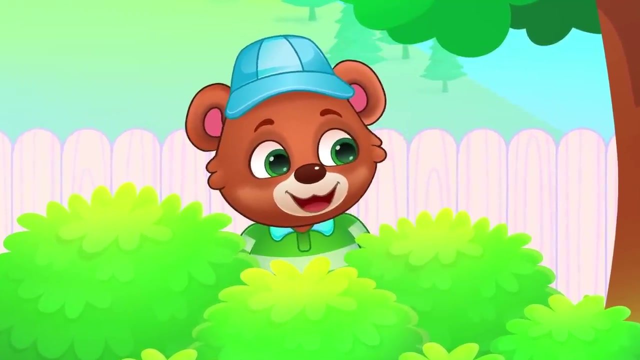 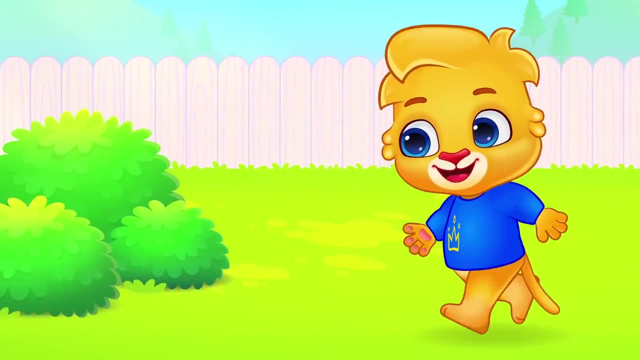 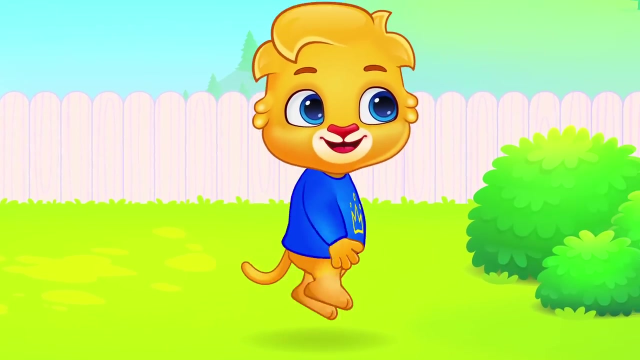 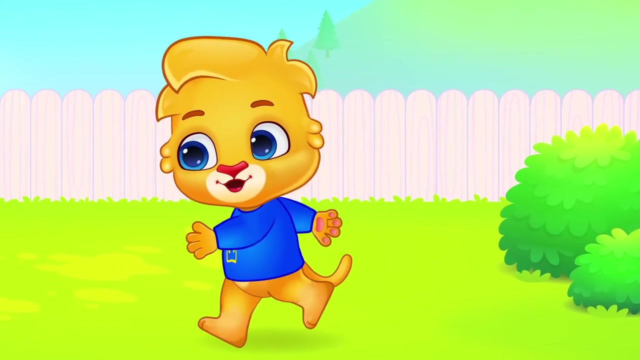 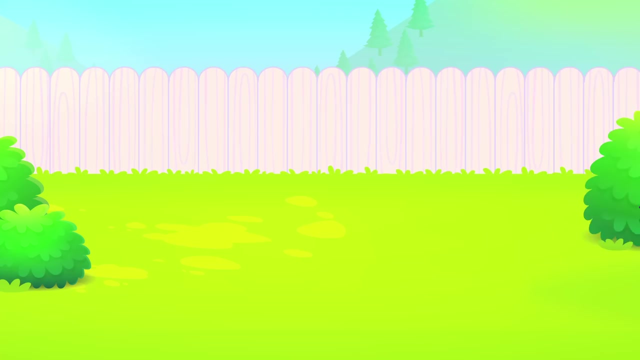 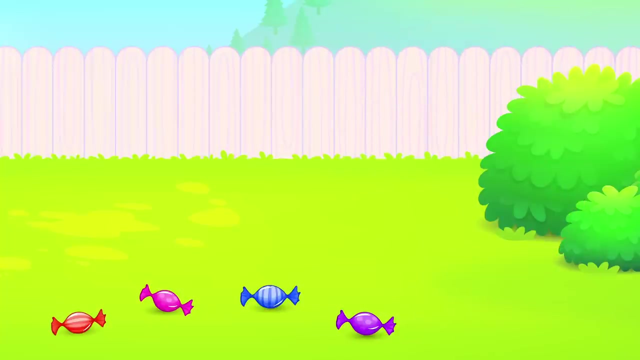 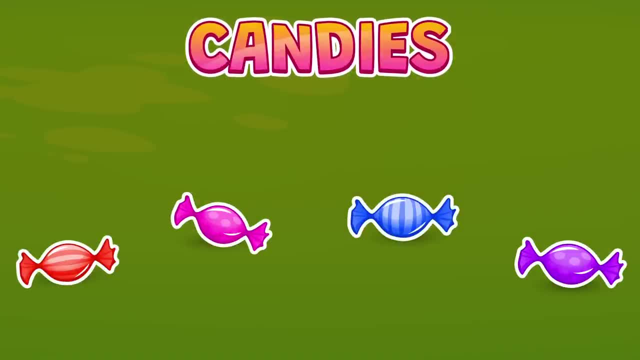 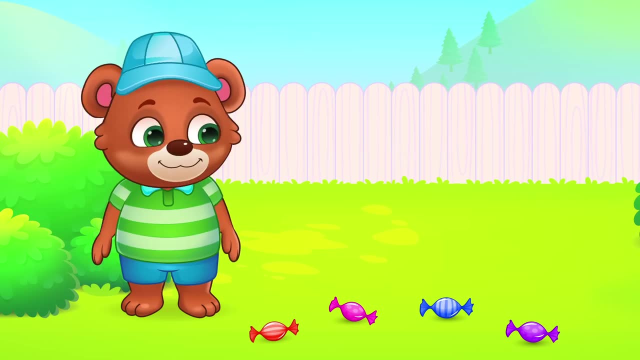 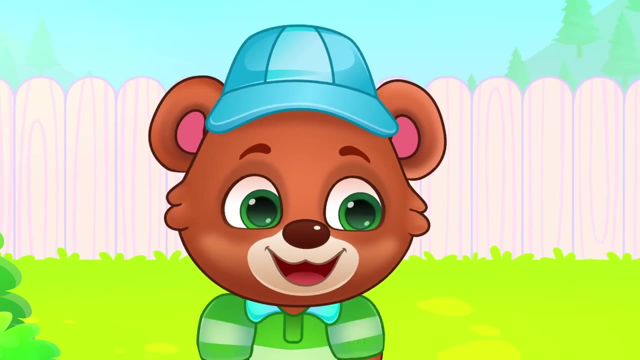 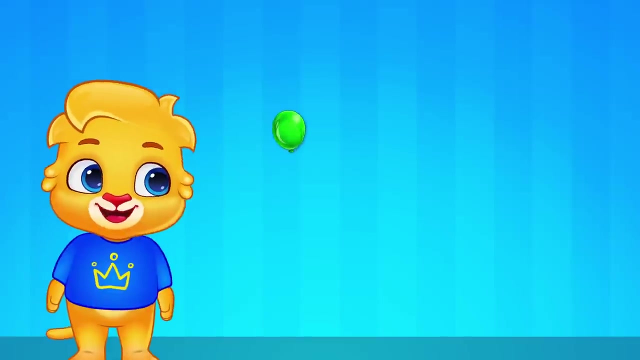 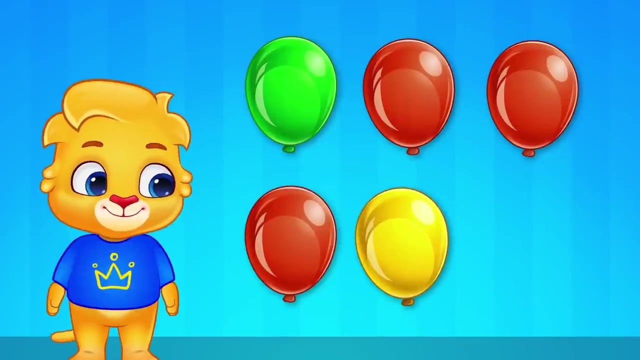 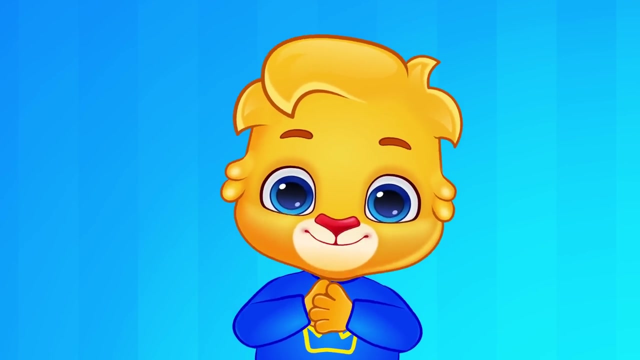 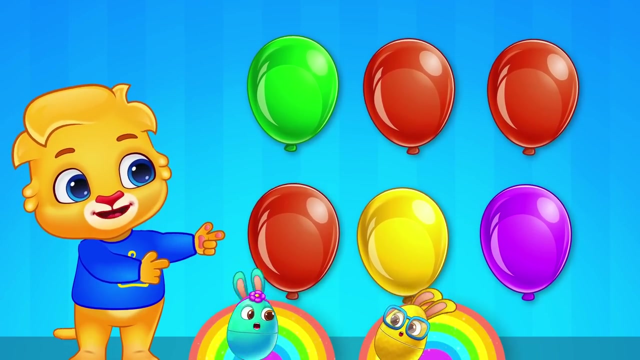 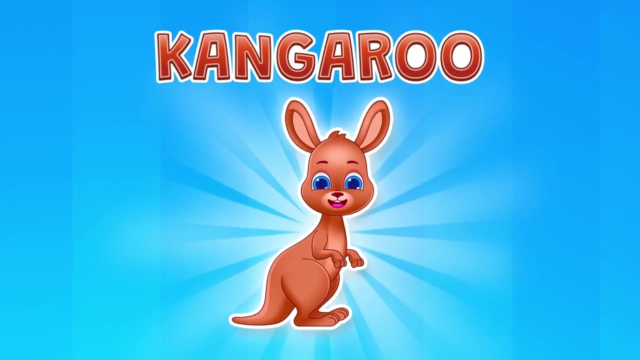 Candies- C is for candies. Oppa, Yummy, Oh, I caught you. Woo, Woo, Yeah, Yeah, Look Balloon. I love balloons. Are you ready to pop balloons with the color brown? Brown Kangaroo is brown. 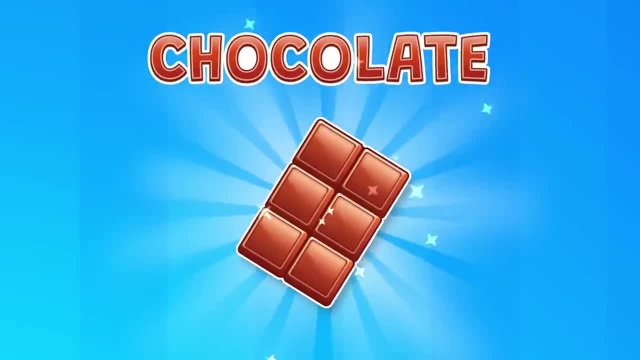 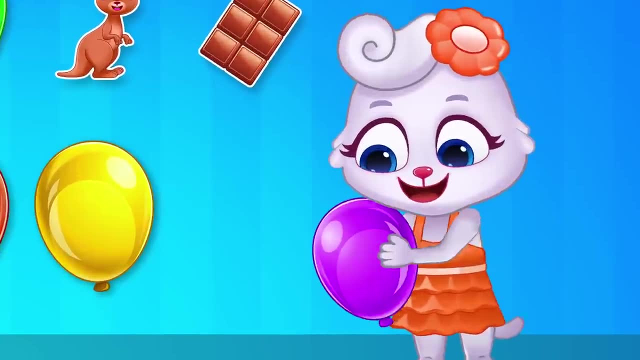 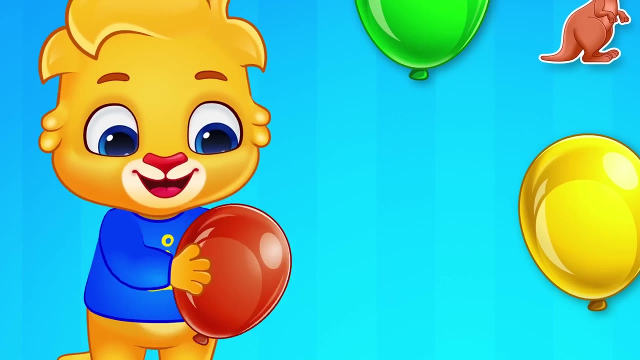 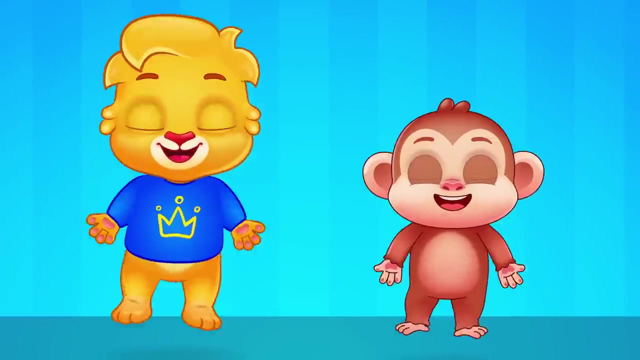 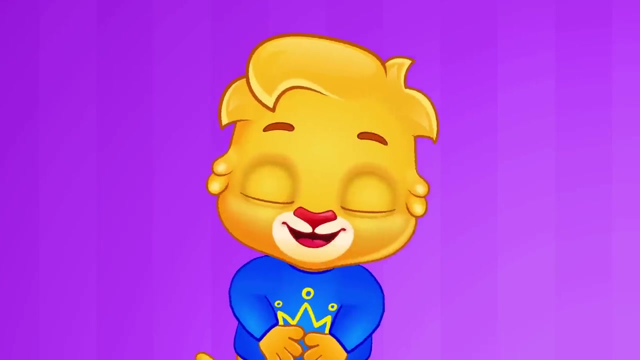 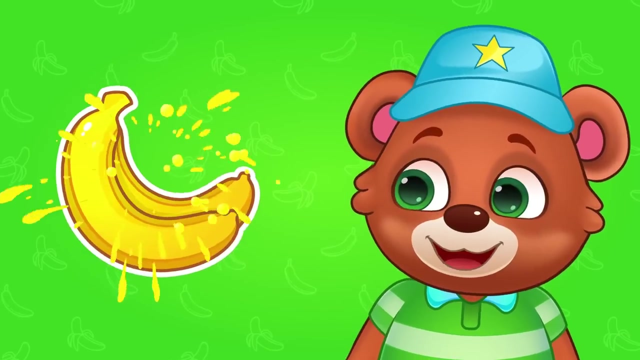 Oh, Brown Chocolate is brown. Oh Yeah, Yeah, Yeah, No, No, No, No, No, No. Brown Monkey is brown. Woo, Yeah, Hi, Yeah, Uh-huh, Yeah, Ew. 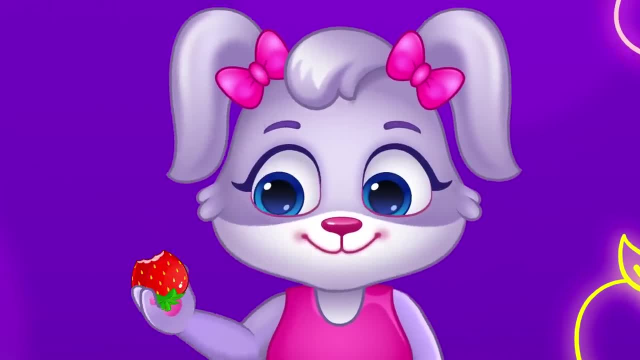 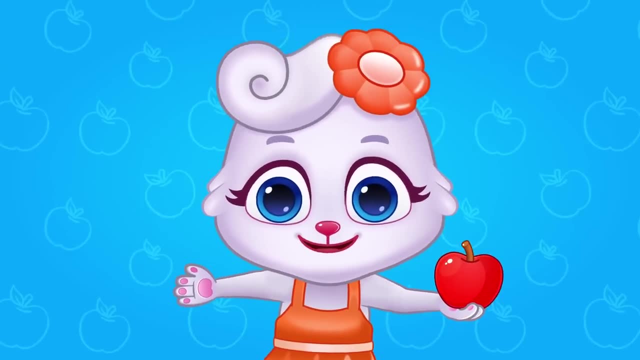 Mm, I eat my fruits every day. Yummy, Yummy, Yummy, Fruits, Fruits. That's so healthy, It's tasty. That's how we eat your fruits every day. Yeah, Every day, Yeah. 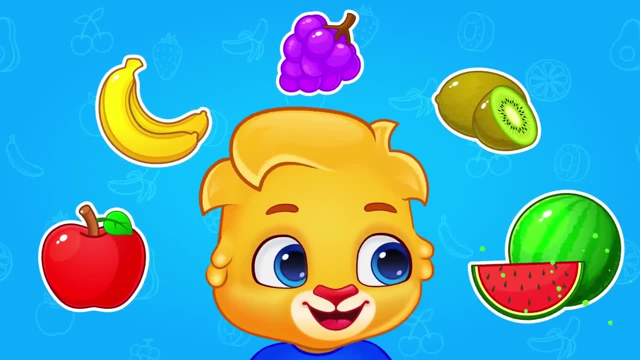 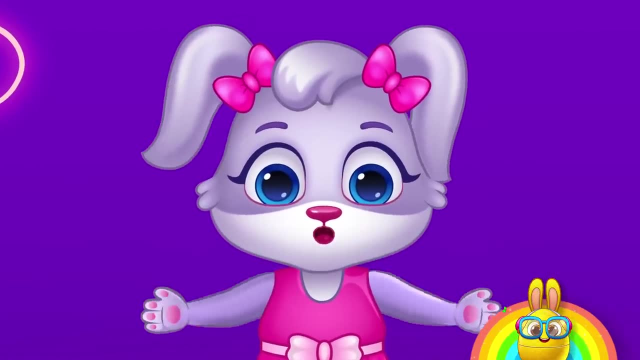 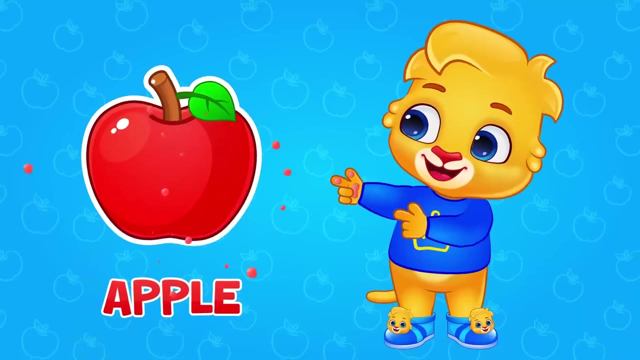 Apples, bananas, grapes, kiwi, watermelon, strawberry, orange, pineapple, cherry, avocado. That's so healthy. Yummy, Yummy, Yummy, Yummy. fruits, Yummy. Yeah, Apples are my favorite. 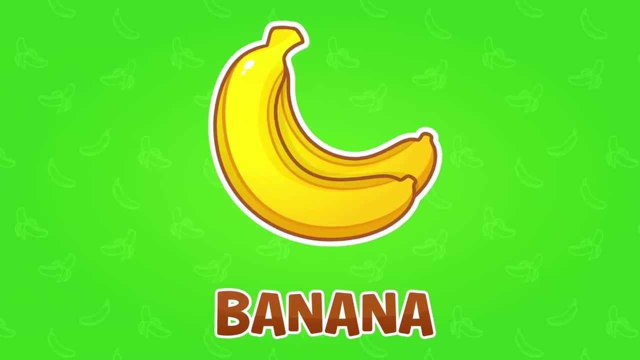 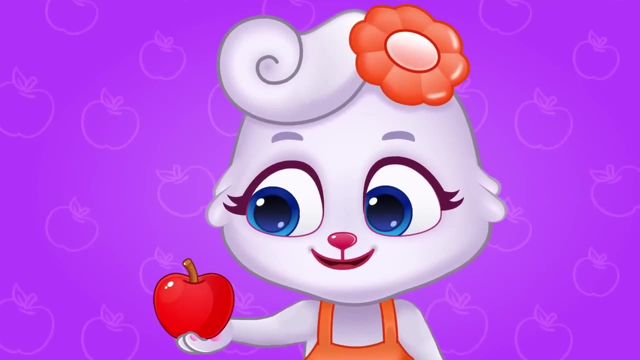 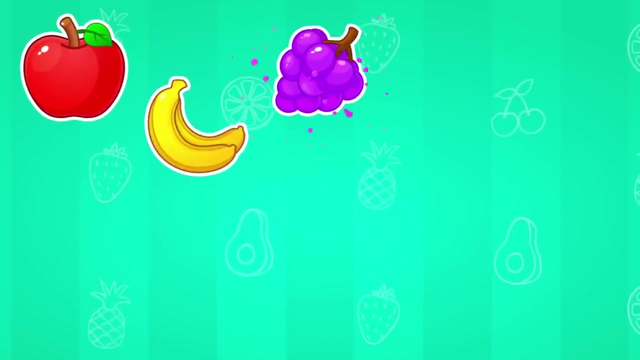 Juicy, juicy red apples. Yeah, Apples are my favorite, Yummy, Yummy, Yummy. Hey Lucas, what fruit is this? It is a red apple. Yay, Apples, bananas, grapes, cherry, watermelon, strawberry, orange, pineapple, cherry, avocado. 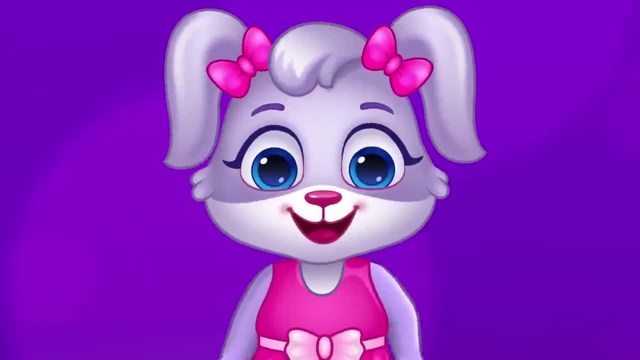 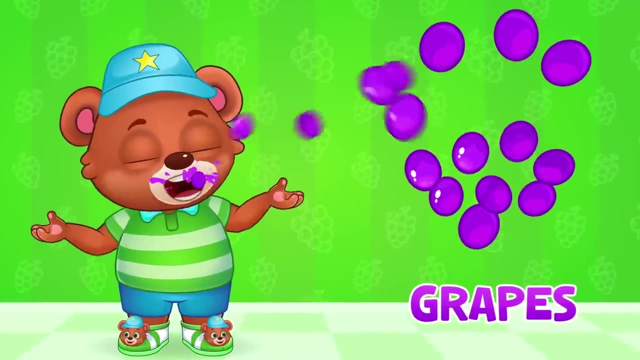 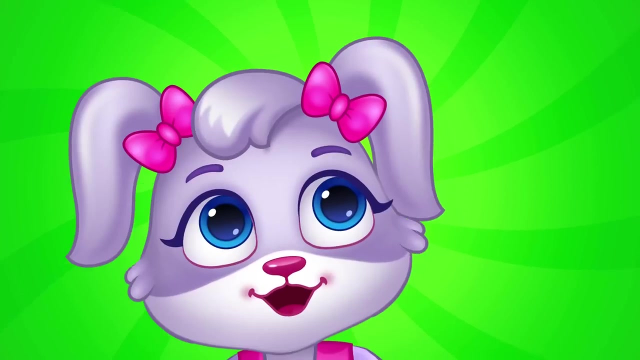 Yummy, Grapes are my favorite. Juicy, juicy purple grapes. Watermelons are my favorite: Yummy, yummy green watermelons. Hey Ruby, can you guess what fruit this is? It is my favorite watermelon. 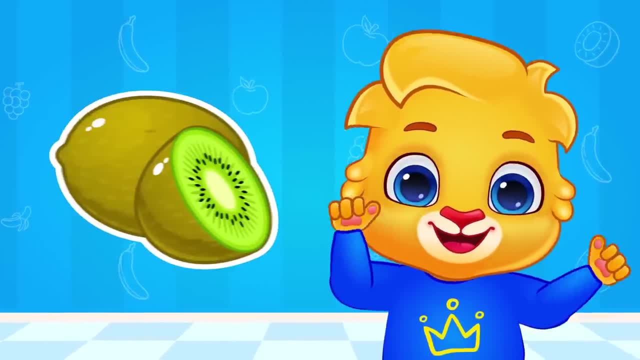 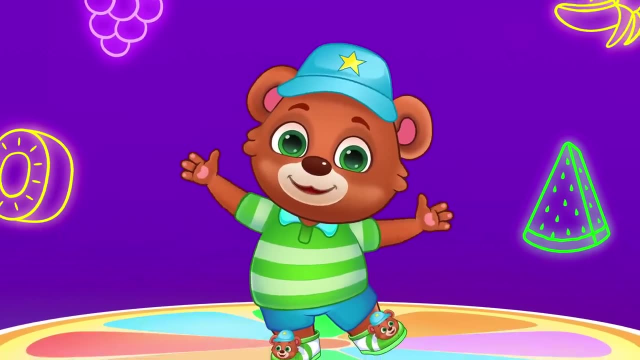 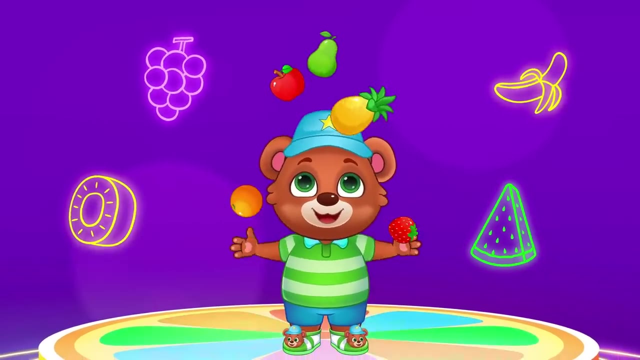 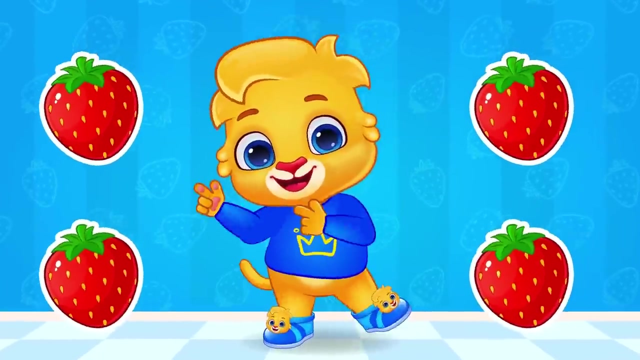 Apples, bananas, grapes, cherry, watermelon, strawberry, orange, pineapple, cherry, avocado. Yummy, yummy, yummy fruit. Orange is my favorite. Juicy, juicy, round orange Strawberries are my favorite, Yummy, yummy red strawberries. 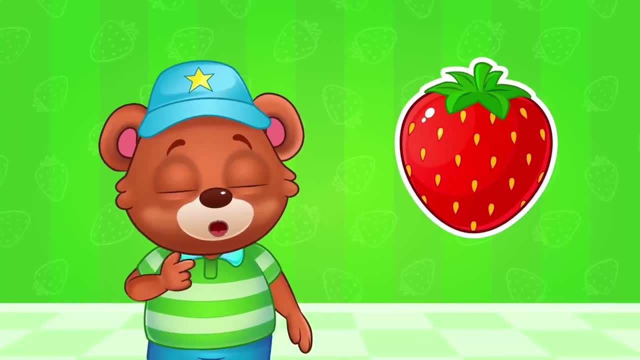 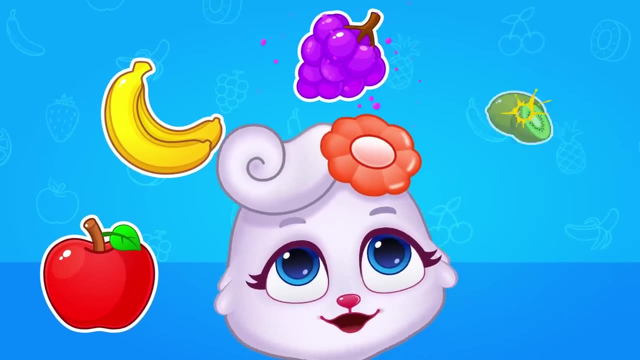 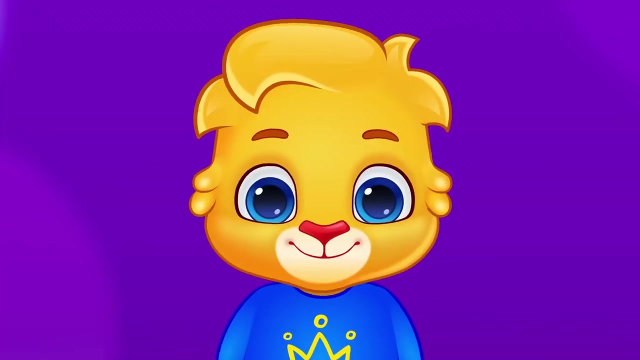 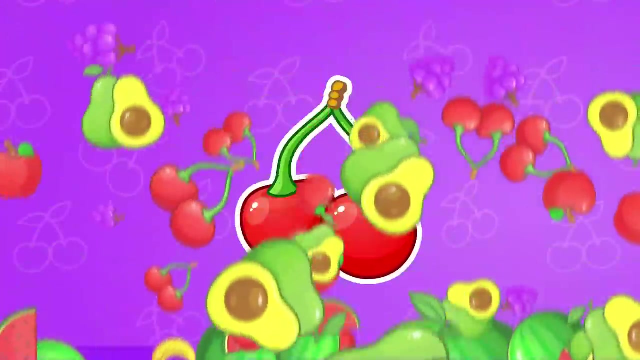 Hey Rudy, what fruit is this? It is a red strawberry. Yay, Apples, bananas, grapes, cherry, watermelon, strawberry, orange, pineapple, cherry, avocado. Yummy, Grapes are my favorite, Cherries are my favorite. 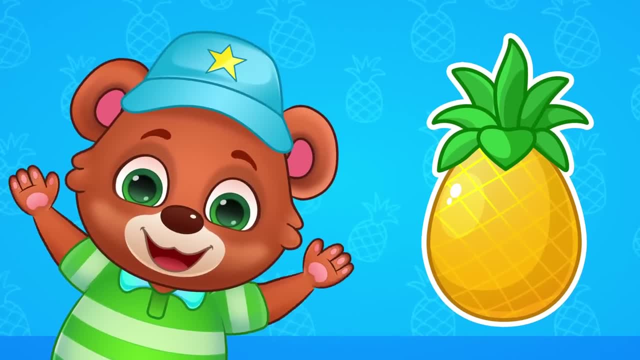 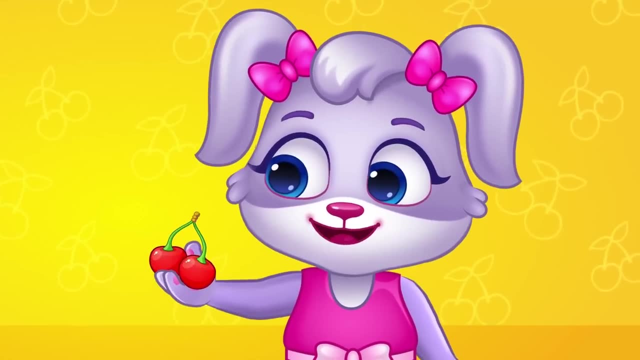 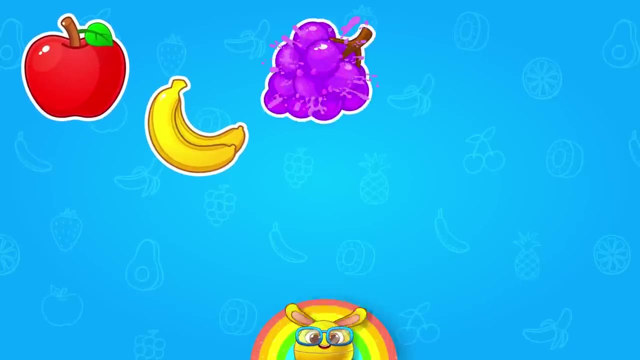 Juicy, juicy red cherries. Pineapple is my favorite, Yummy, yummy yellow pineapple. Hey Lily, can you guess what fruit this is? It is my favorite: cherry Apples, bananas, grapes, cherry, watermelon, strawberry, orange, pineapple, cherry avocado. 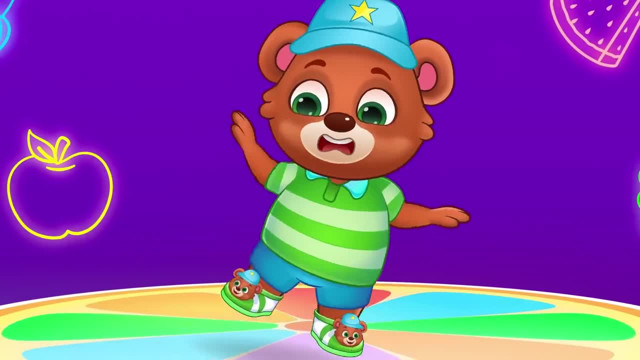 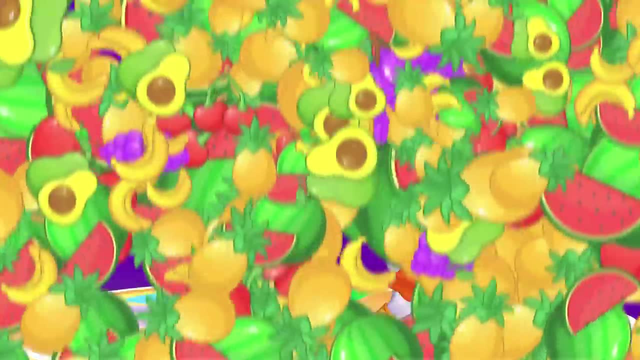 Whoa, Hello, Hello, Her, her, her, Her, her, her, Uh-huh. Kiwis are my favorite. Yummy yummy brown kiwis. Uh-huh, These are my favorite. Yummy yummy green avocados. 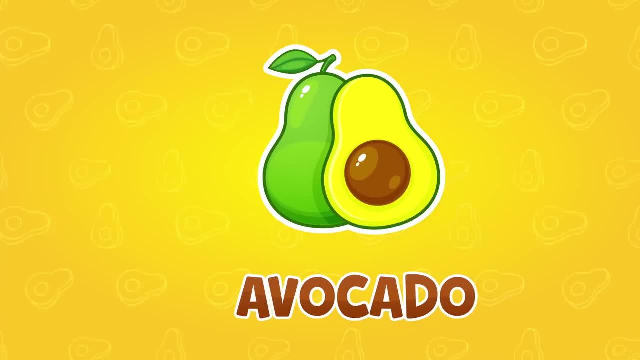 Yay, Apples, bananas, grapes, cherry, watermelon, strawberry, orange, pineapple, cherry, avocado, Tum-tum, Yeah, Eh, there are more. The best for me? Ah, there are many Ready. 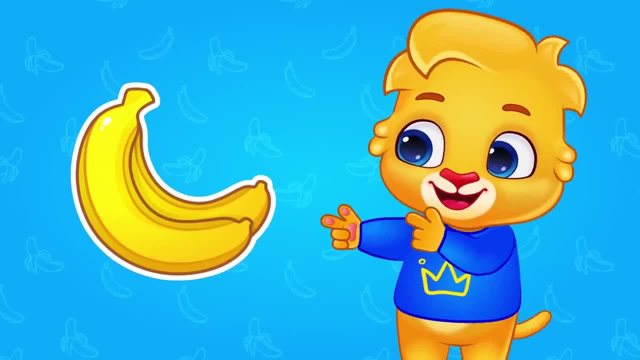 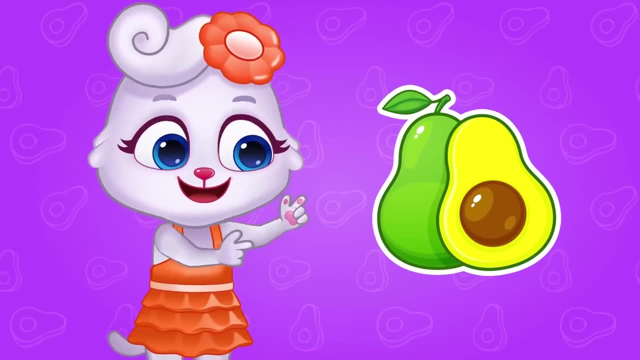 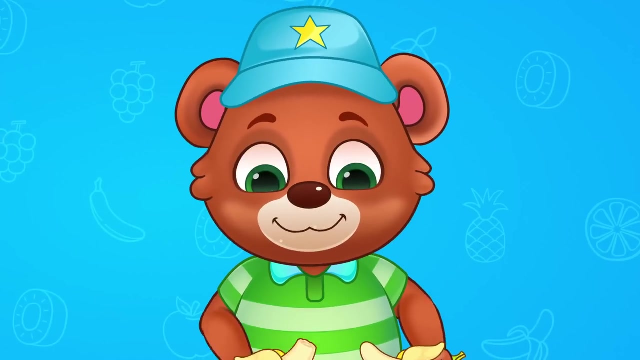 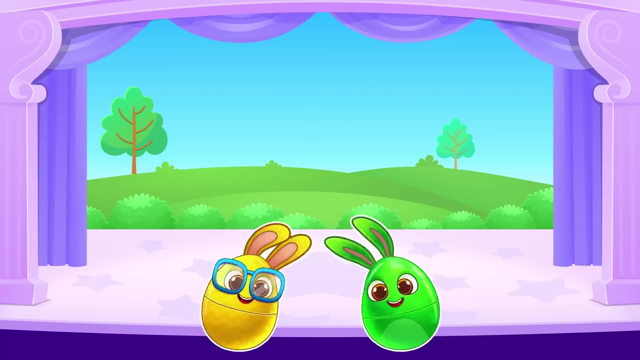 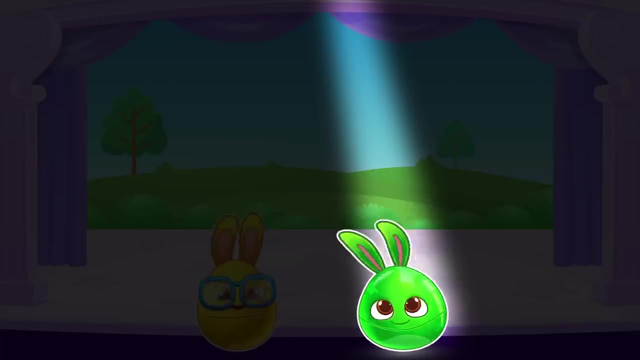 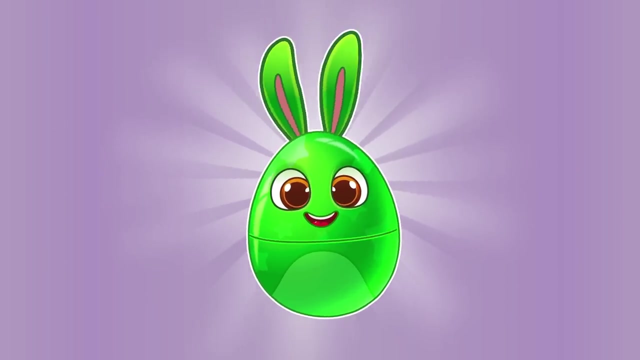 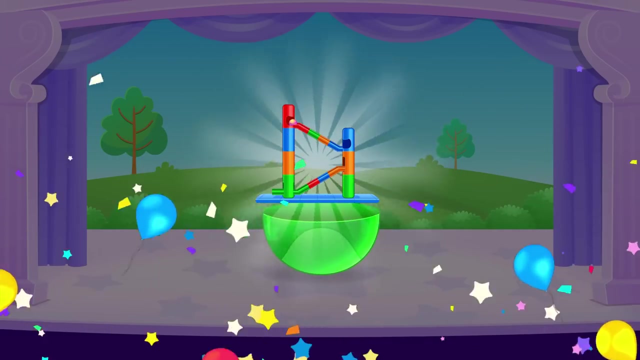 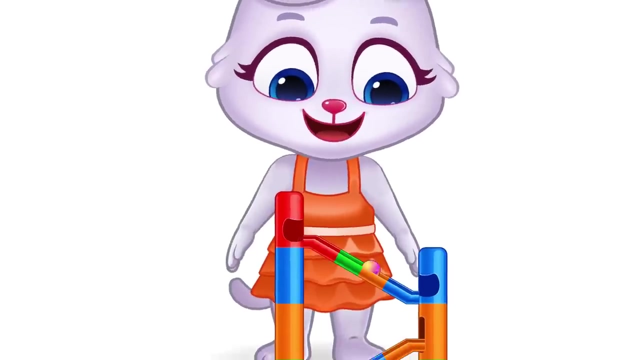 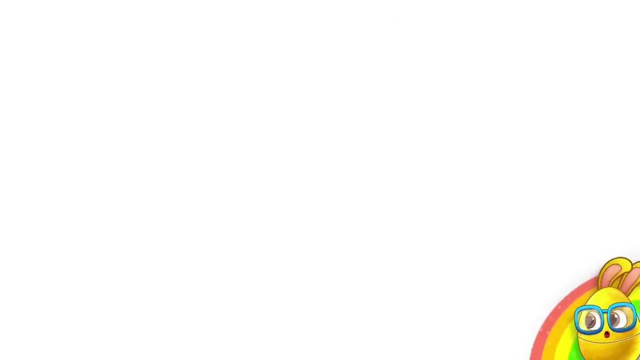 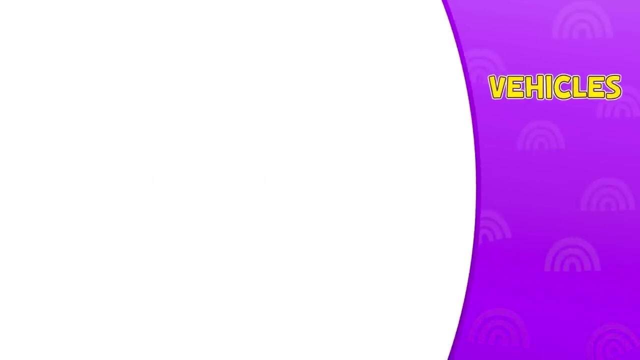 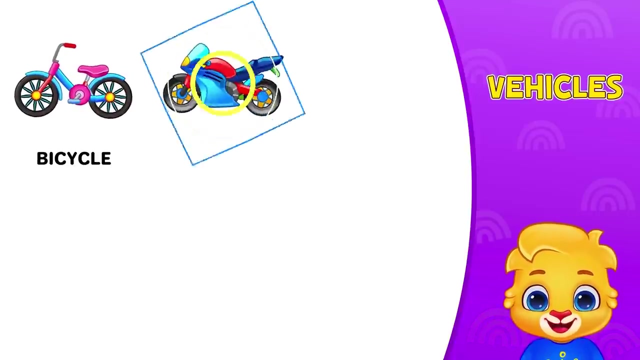 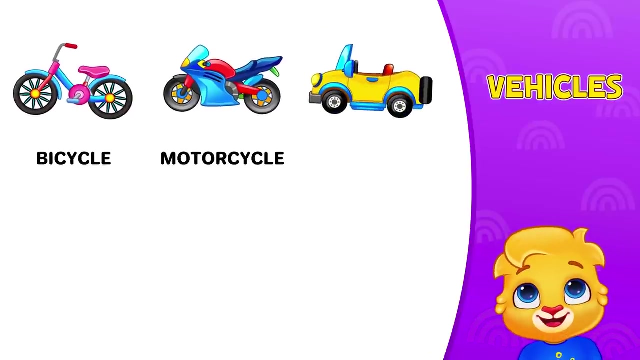 There are many troush, Ha, Thank you. Uh-huh, It is my favorite fruit, Excitement. Uh-huh, Oh, cherry avocado. Oh, Still not me, but I know I will be the next one. vehicles, Bicycle, Motorcycle, Car. 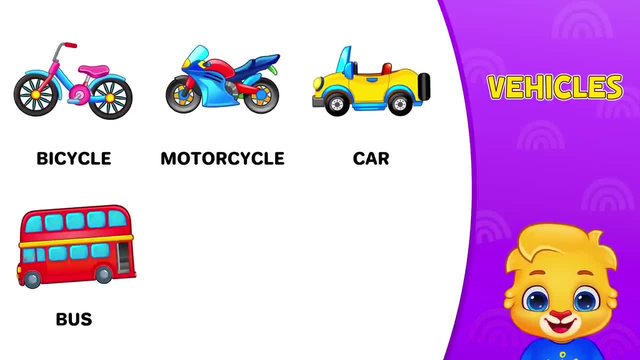 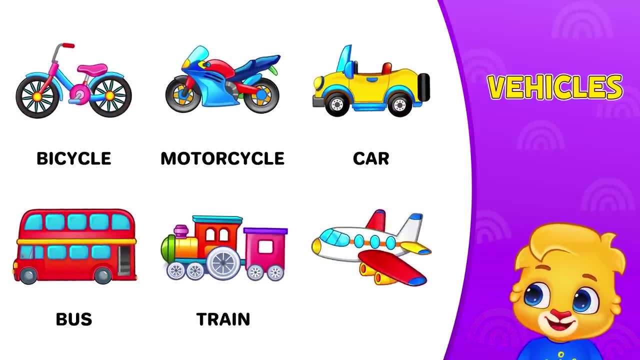 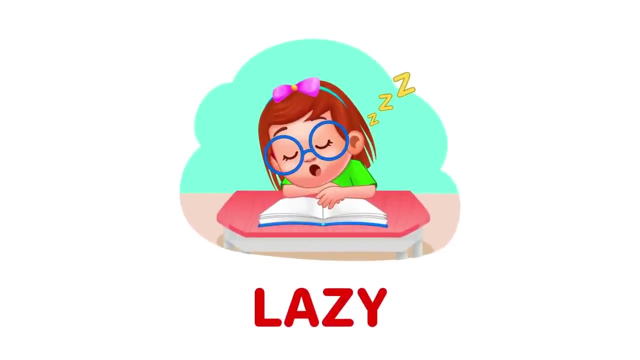 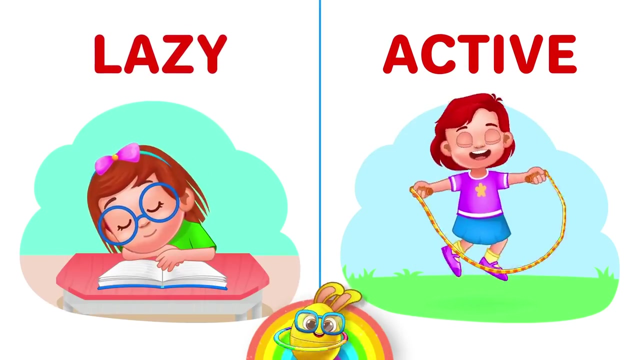 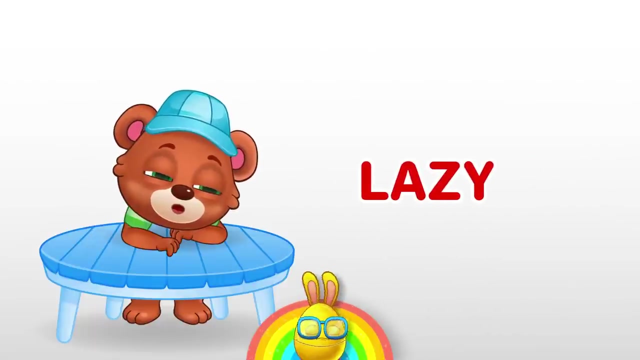 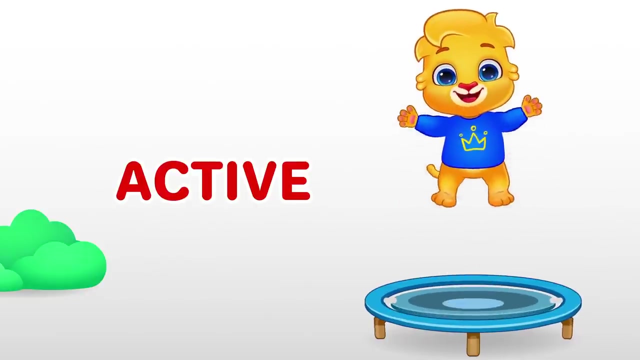 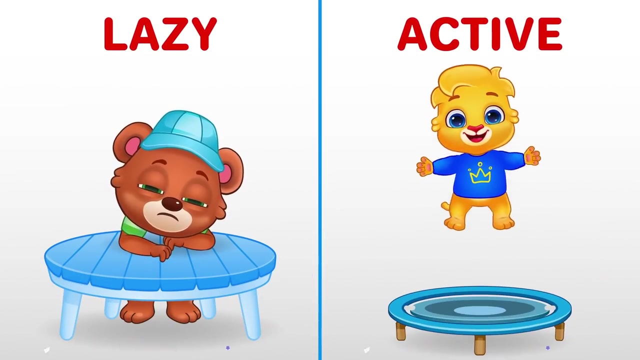 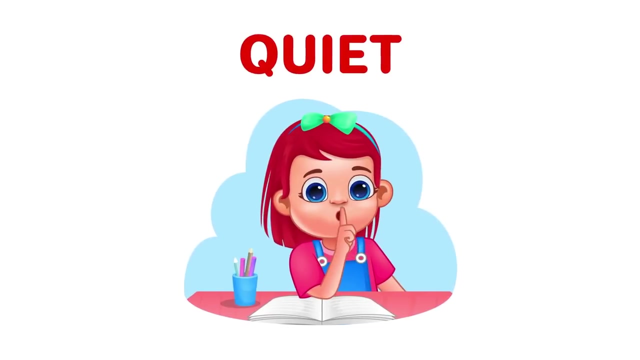 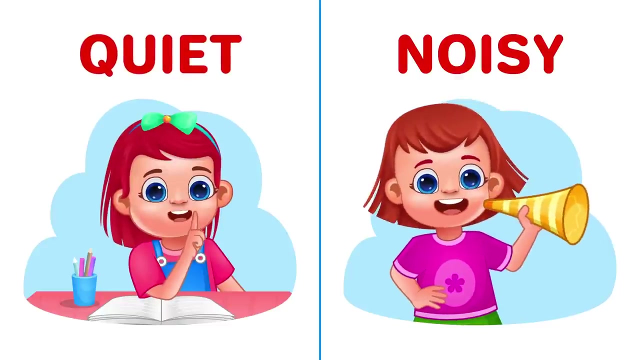 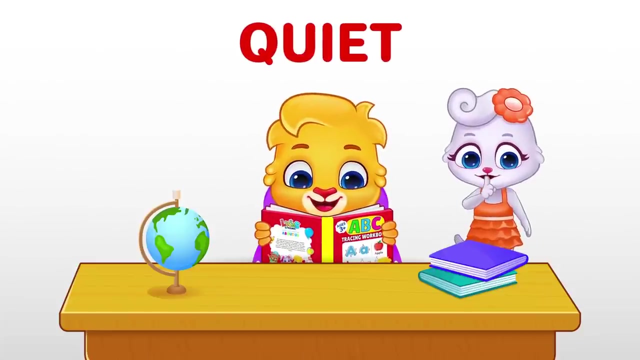 Bus Train Airplane: Lazy, active, lazy and active, lazy and active, lazy and active, lazy. Brody is lazy, active, Lucas is active, lazy and active. Quiet, noisy, Quiet and noisy Quiet and noisy, Quiet and noisy quiet. Lucas wants quiet, shh Noisy. Ruby's symbol is noisy. 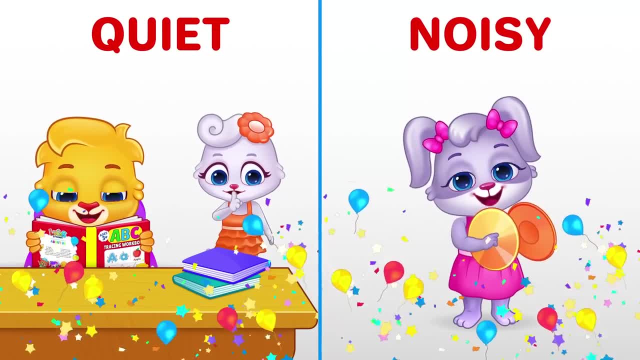 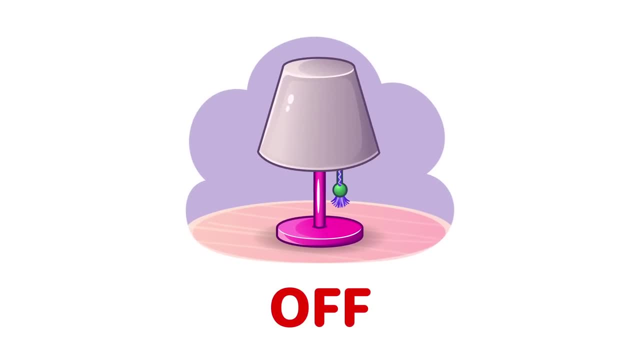 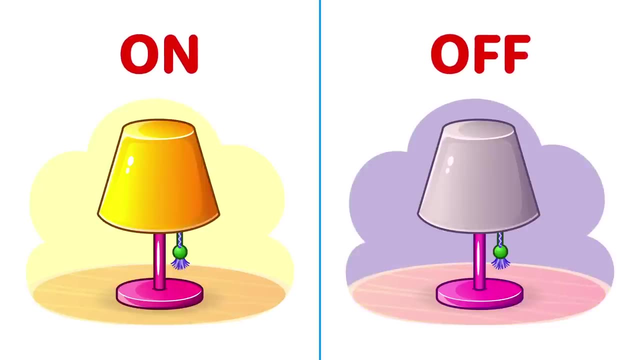 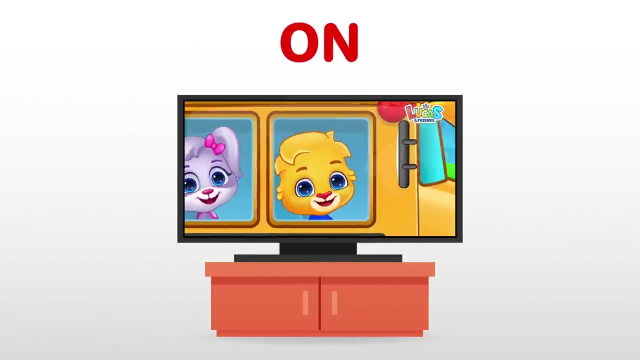 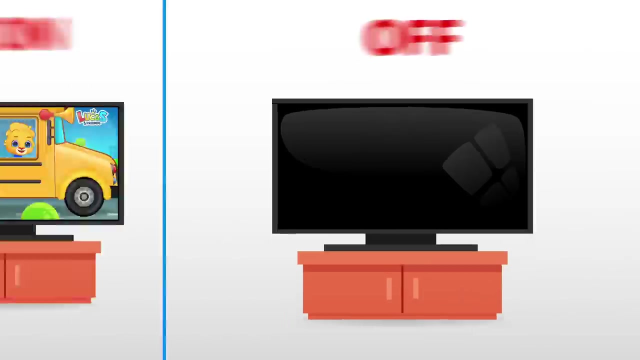 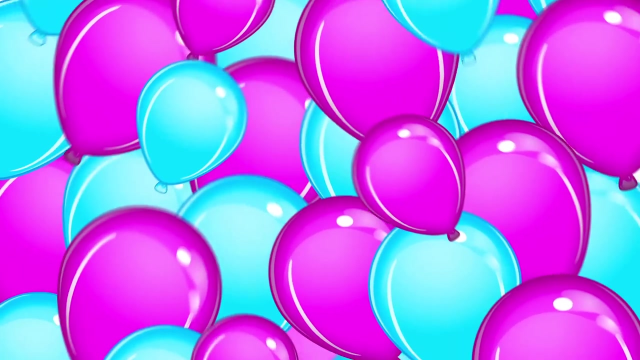 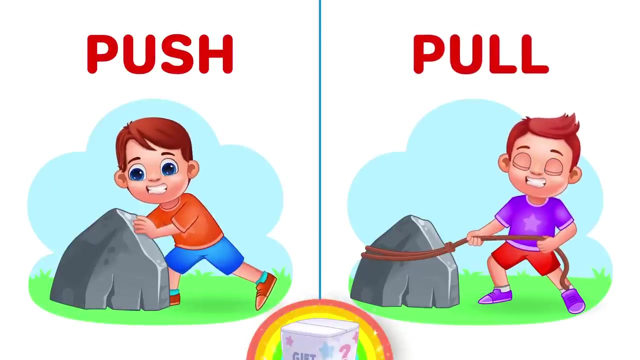 Quiet and noisy shh On off, On and off, On and off, On and off, On. Turn on the TV Off. Turn off the TV, On and off, Push, pull, Push and pull, Push and pull, Push and pull, Pull, Push. Brody is pushing. 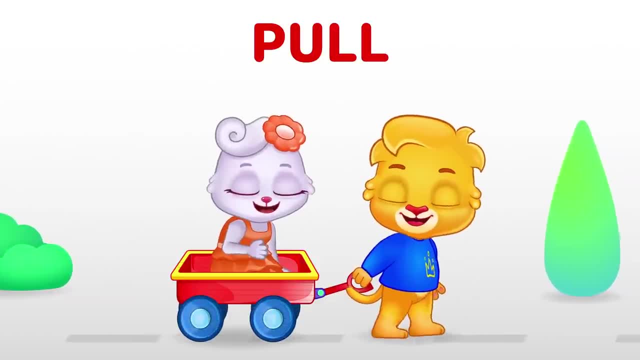 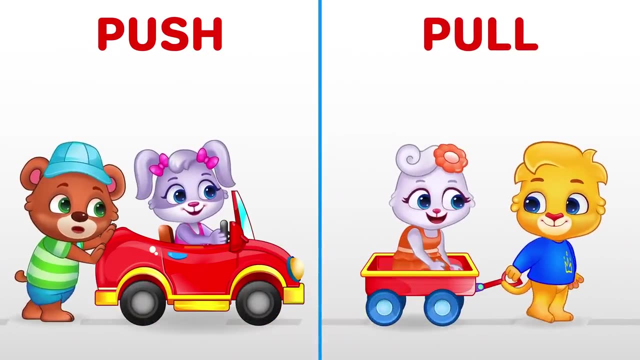 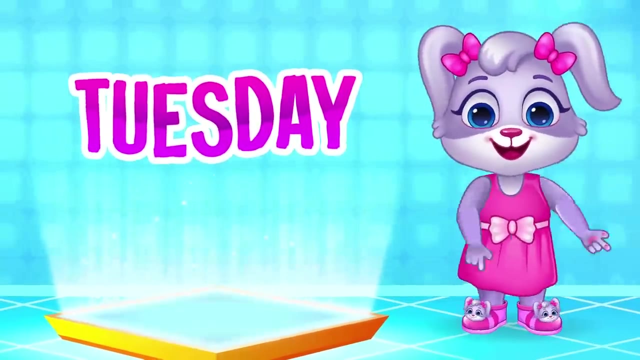 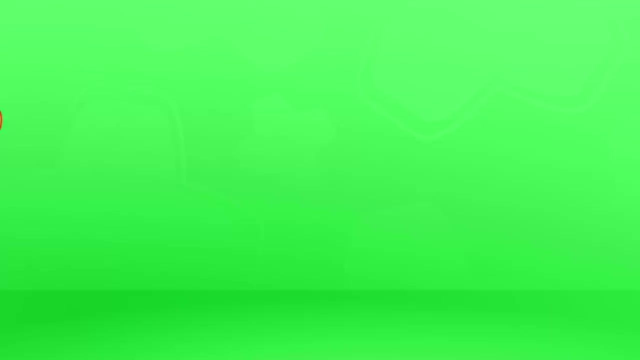 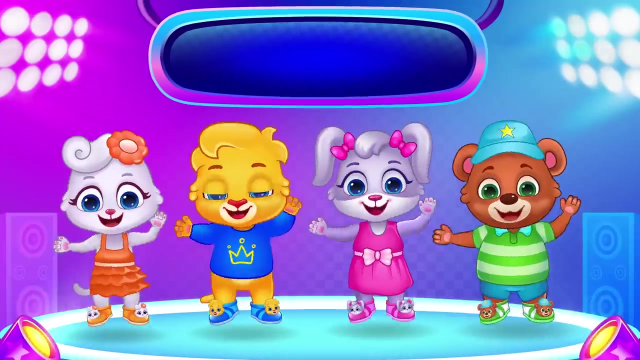 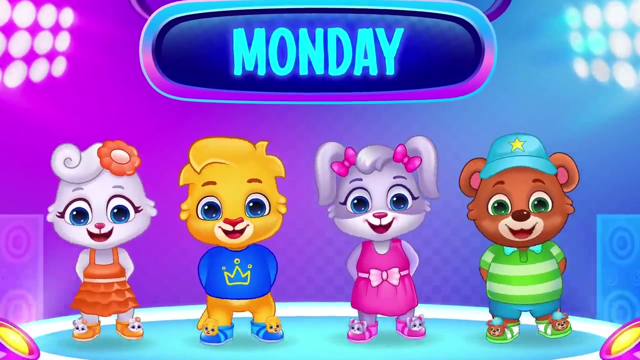 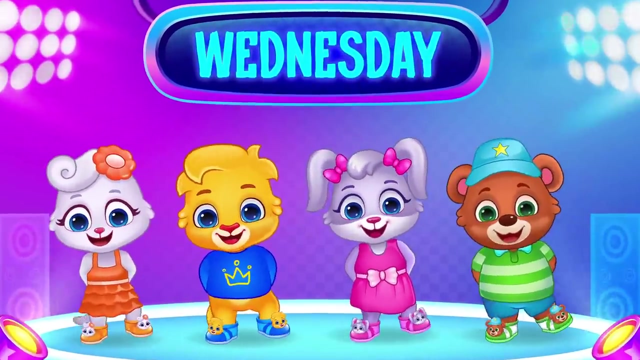 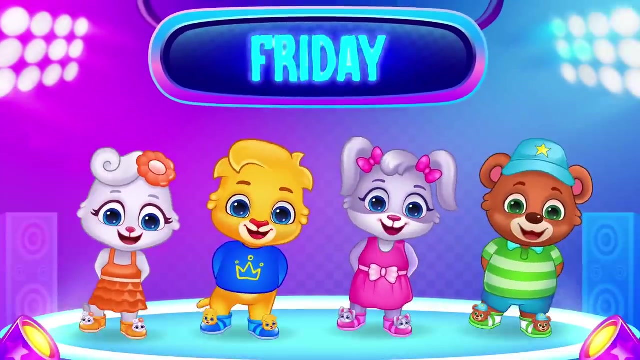 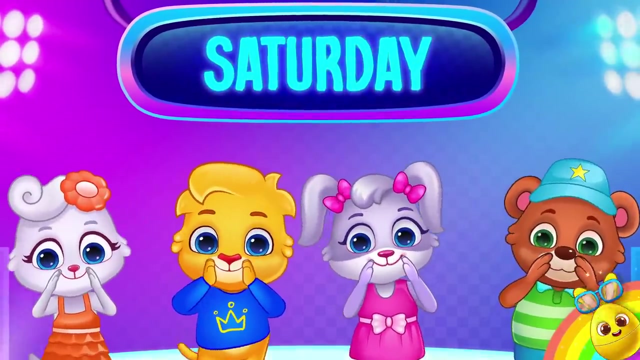 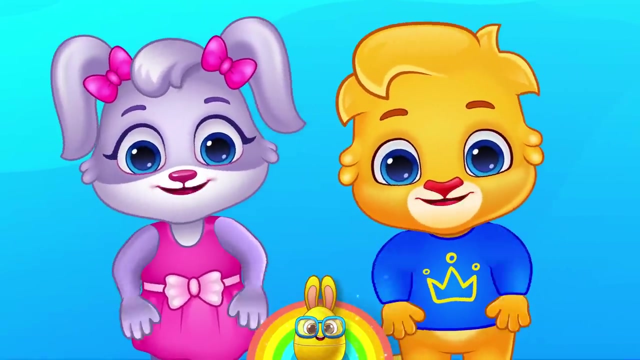 Pull. Lucas is pulling, Push and pull. Sunday, Monday, Tuesday, Wednesday, Thursday, Friday, Saturday. Can you repeat it with me? Yeah, Sunday, Sunday. Monday, Monday, Tuesday, Tuesday, Wednesday, Wednesday, Thursday, Thursday, Friday, Friday, Saturday, Saturday. This is so much fun, Let's sing it again Sunday. 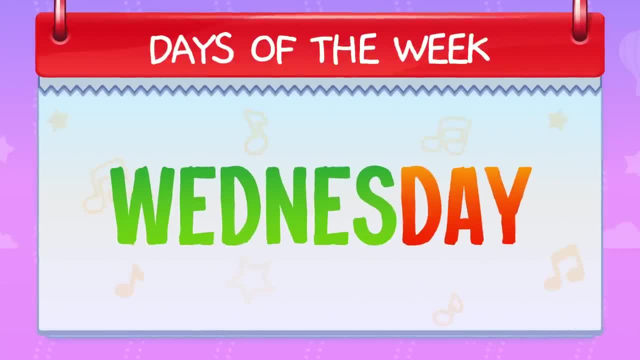 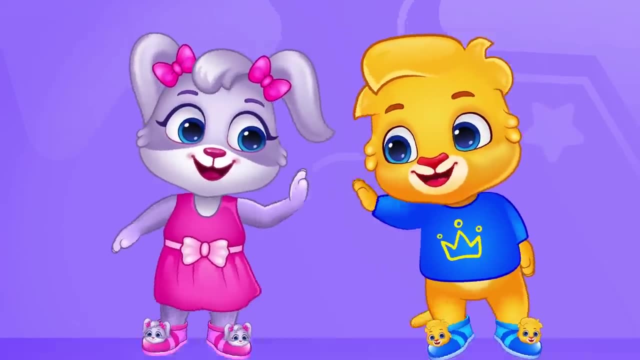 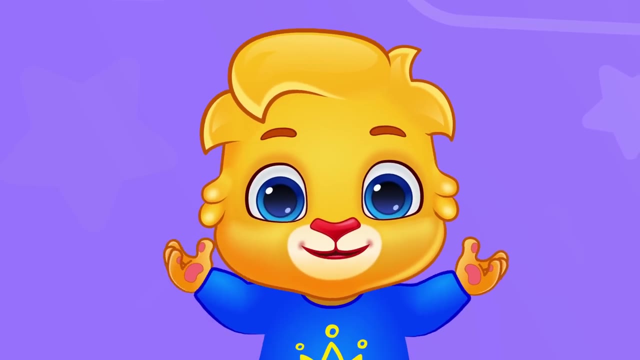 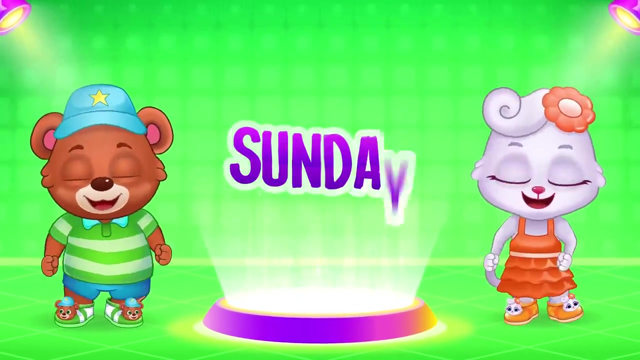 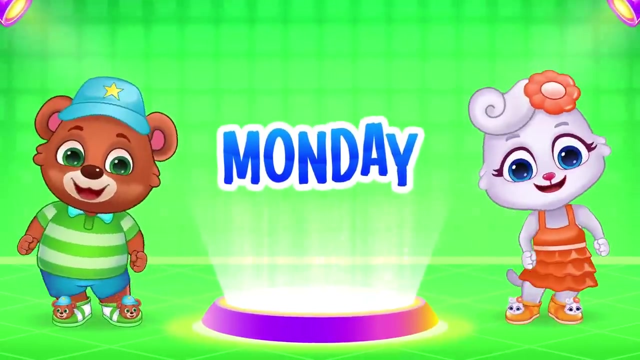 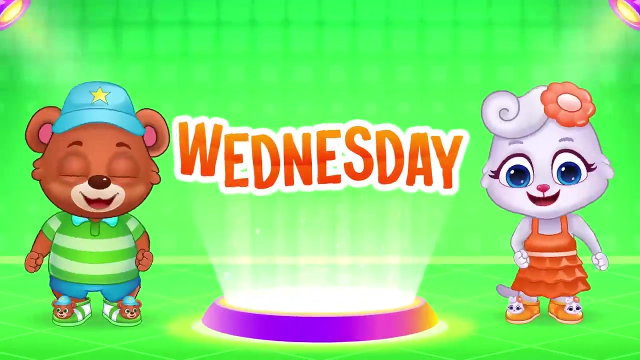 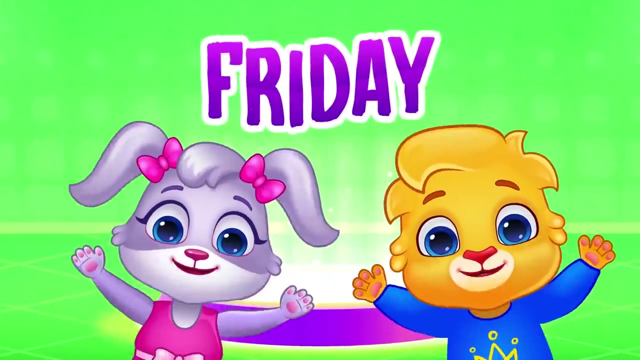 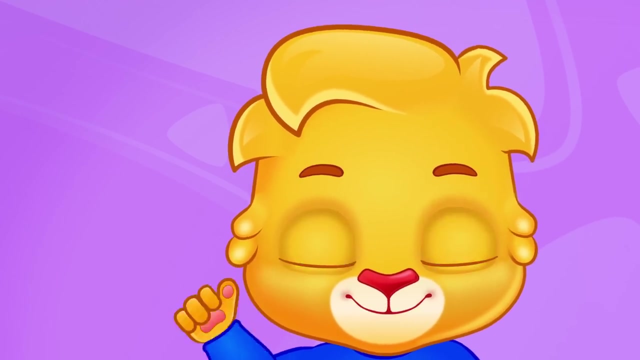 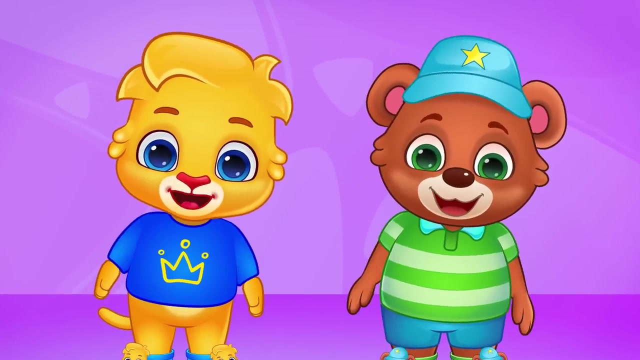 Monday, Tuesday, Wednesday, Thursday, Saturday. Yeah, Awesome, Can you sing with me one more time with a loud voice? Let's go Sunday, Sunday, Monday, Monday, Tuesday, Tuesday, Wednesday, Thursday, Thursday, Thursday, Friday, Friday, Saturday, Saturday. Hey, Can we do it a little faster? Let's go. 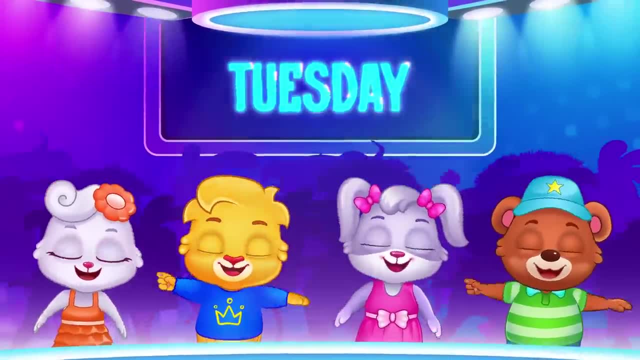 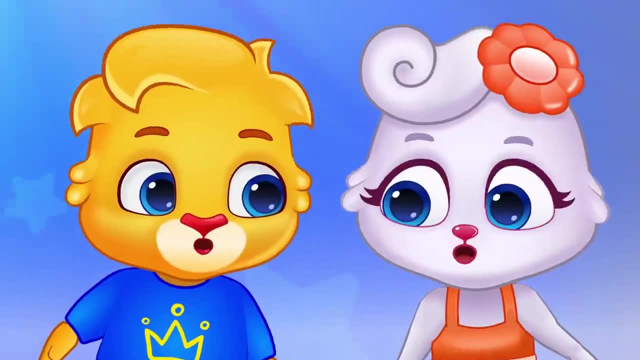 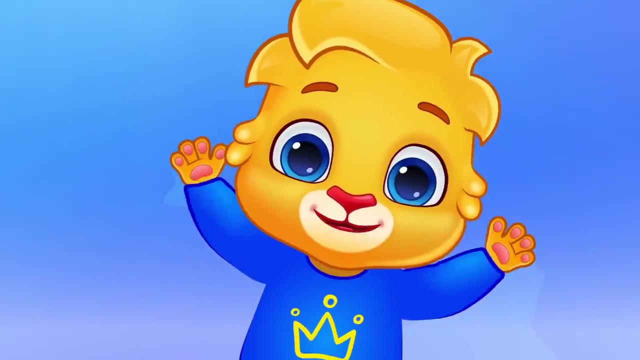 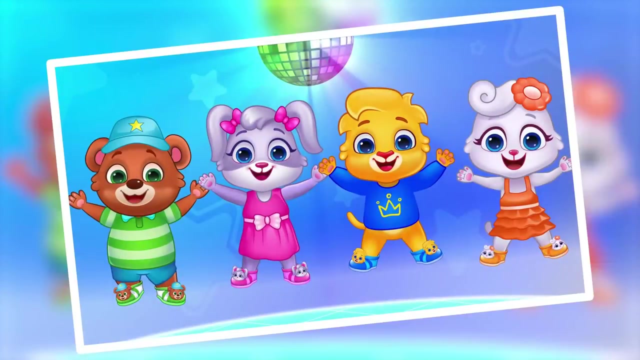 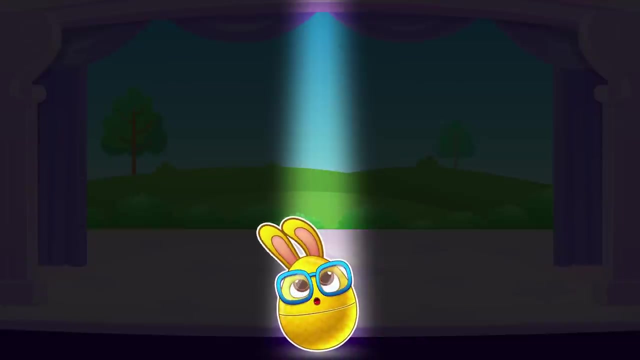 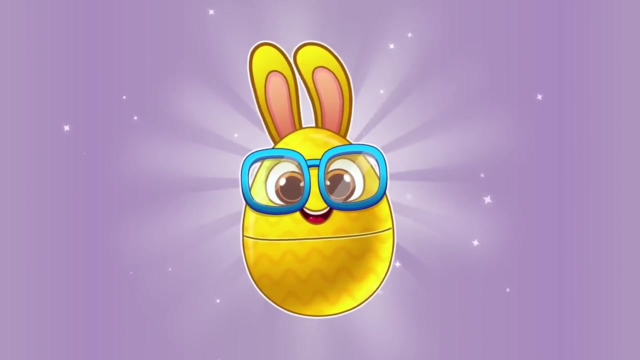 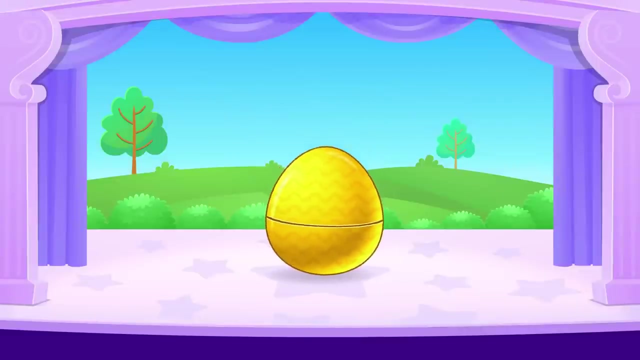 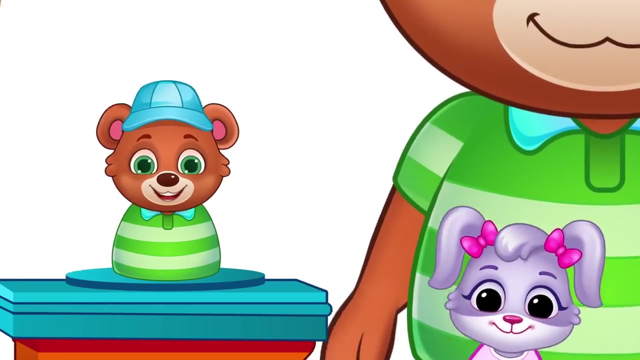 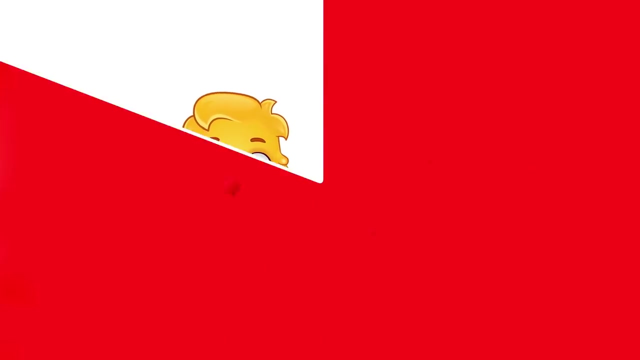 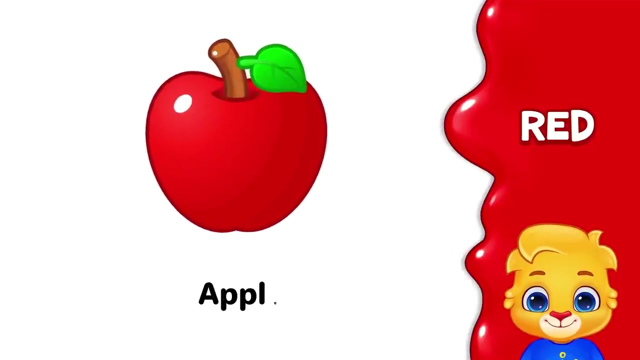 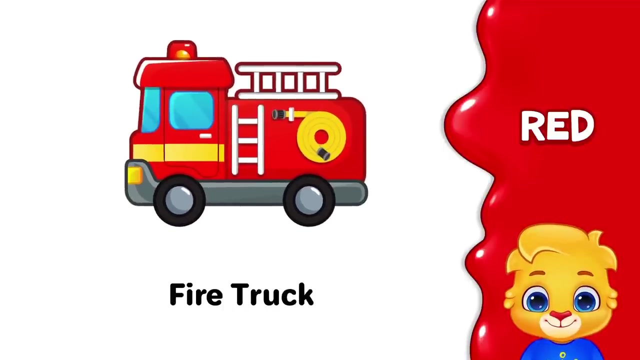 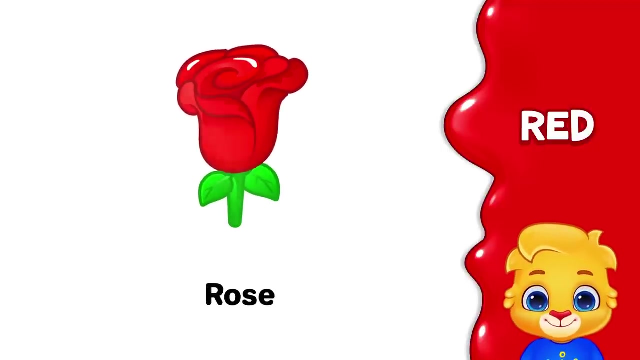 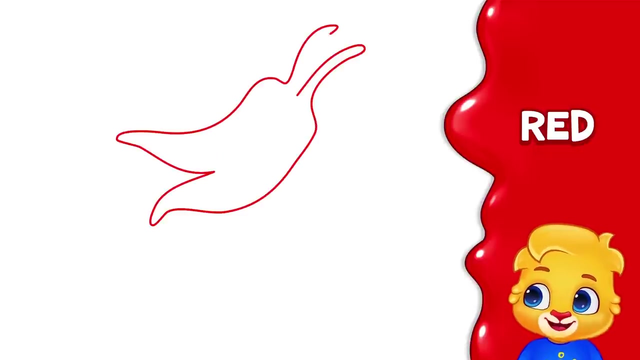 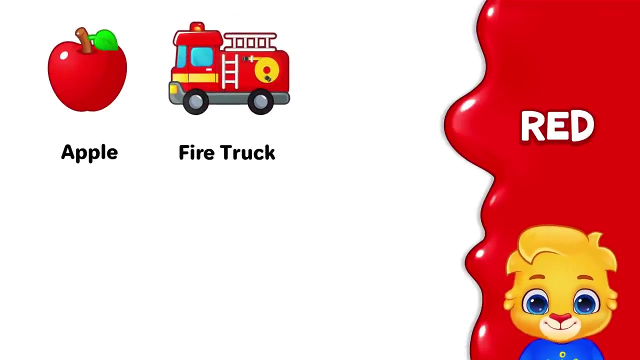 Sunday, Monday, Tuesday, Friday, Saturday, Sunday, Monday, Tuesday, Wednesday, Thursday, Friday, Saturday. Keep learning, keep smiling. Sunday, Sunday, Sunday, Saturday: Sunday: Sunday, Sunday: red apple is red, fire truck is red, rose is red, car is red, strawberry is red, red chili is red. red apple, red fire truck, red rose, red car, red.